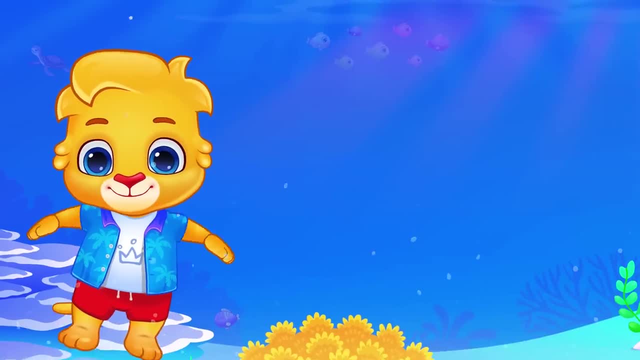 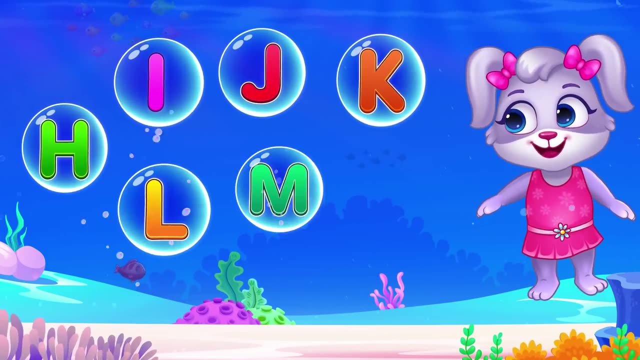 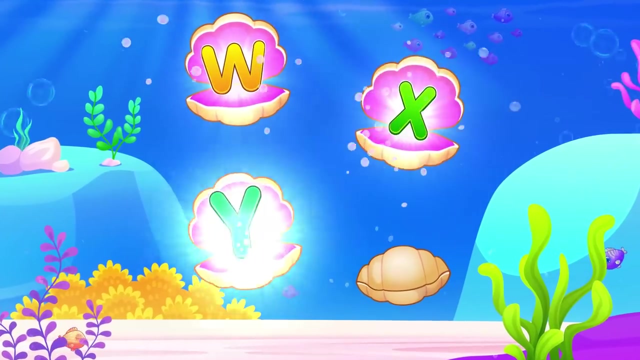 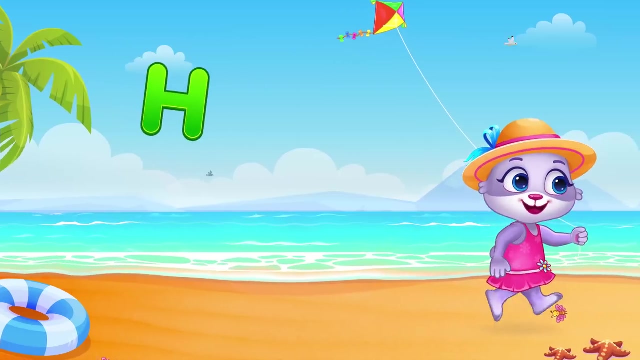 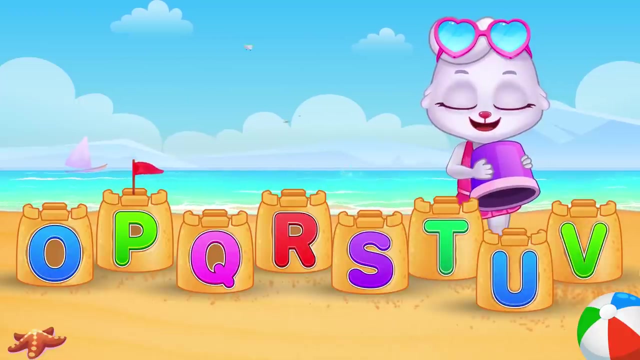 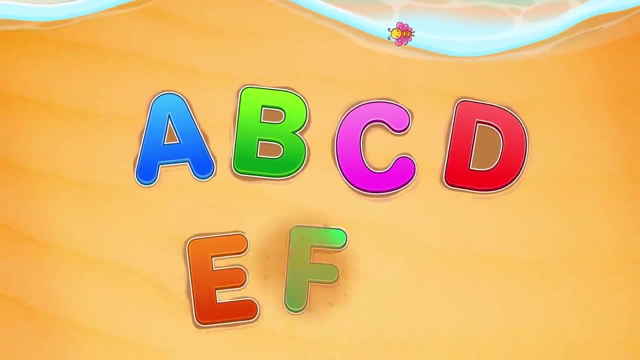 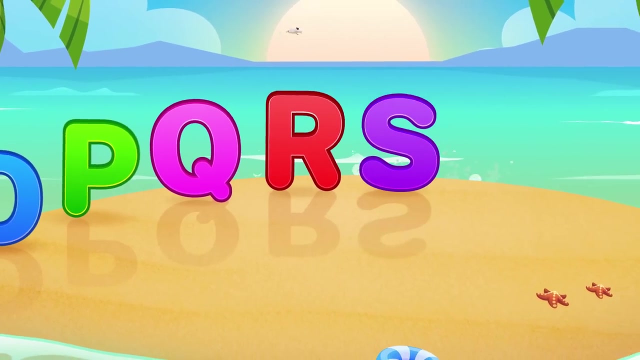 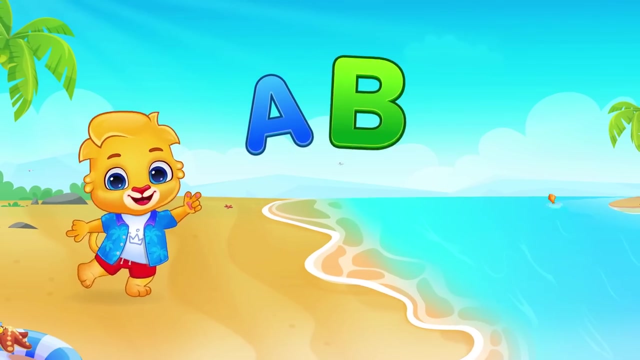 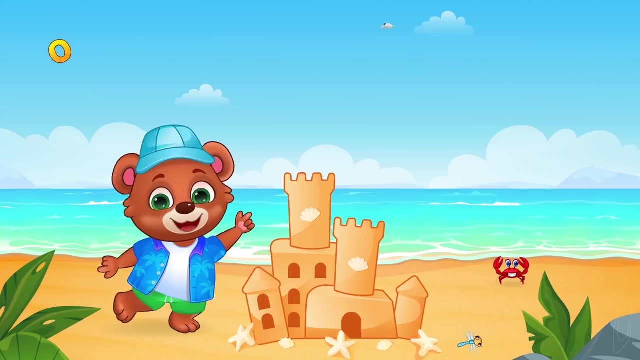 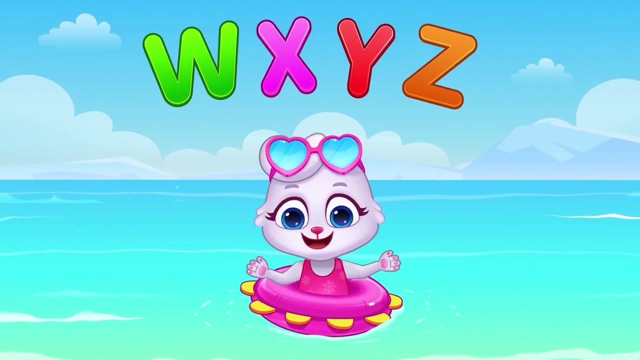 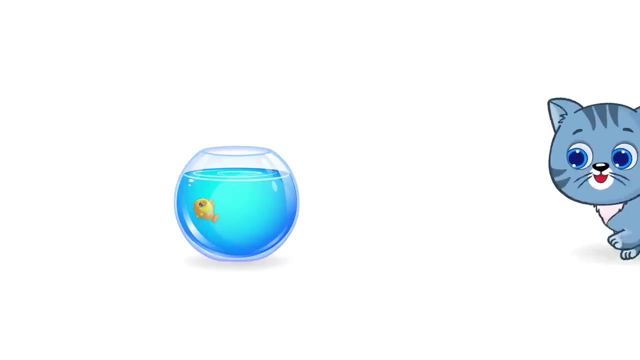 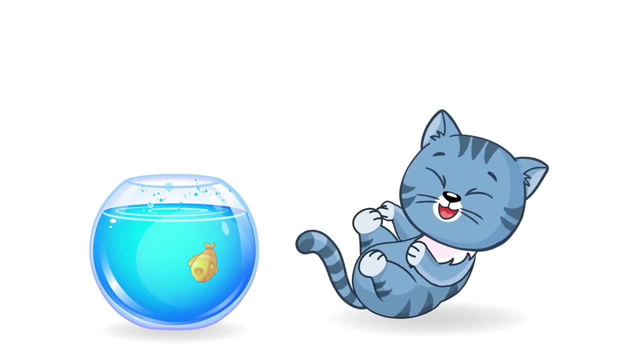 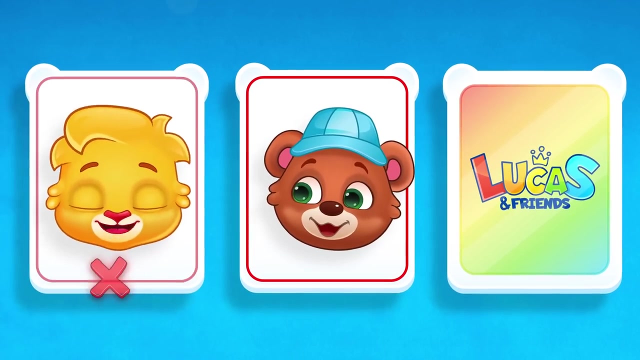 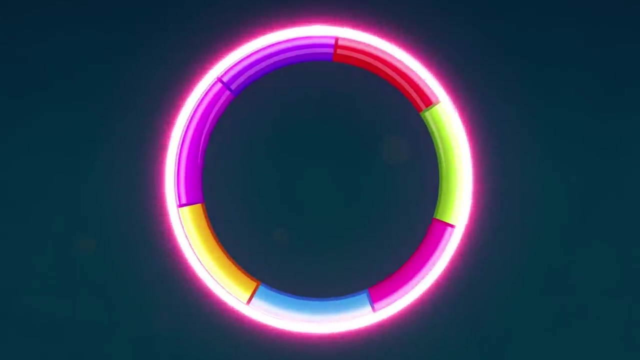 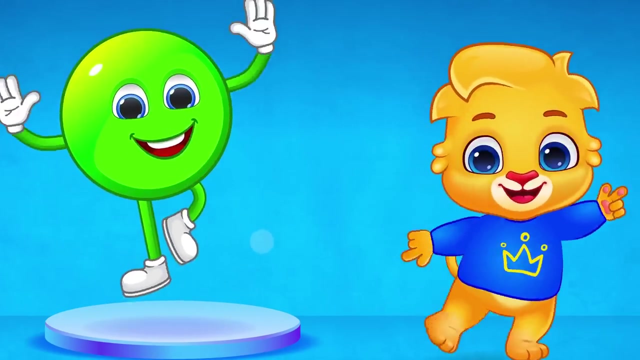 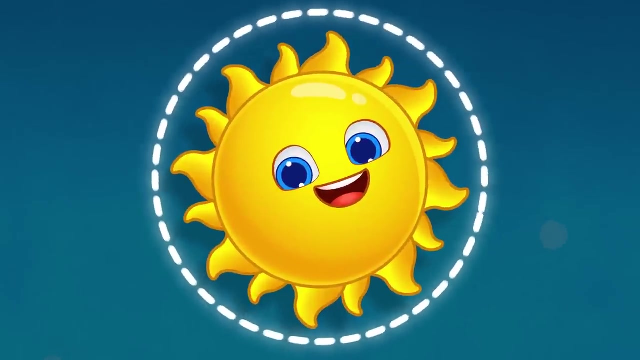 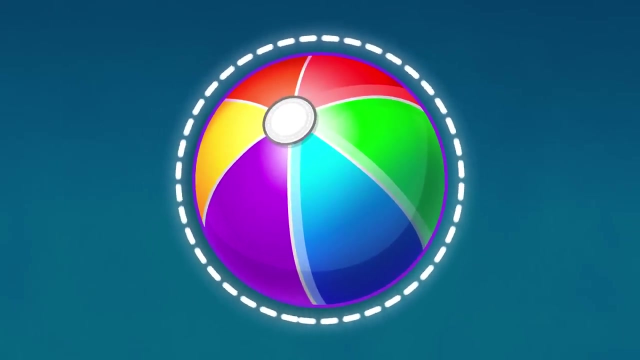 Thank you for watching. Thank you for watching P-Q-R-S-T-U-V-W-X-Y-N. Hula Hoop Ring. Hula Hoop Ring, Circle, Circle, Circle. This is Circle. Sun, Sun Circle. Ball Ball Circle. Donut, Donut, Donut Circle. 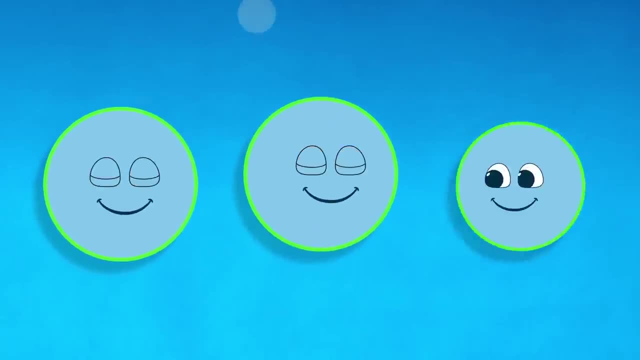 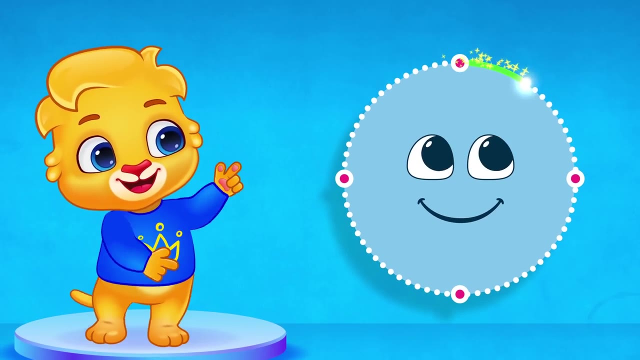 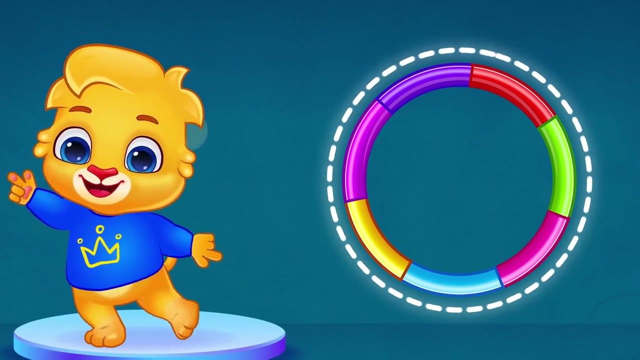 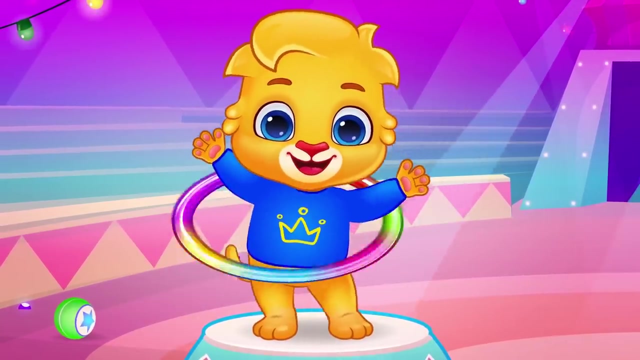 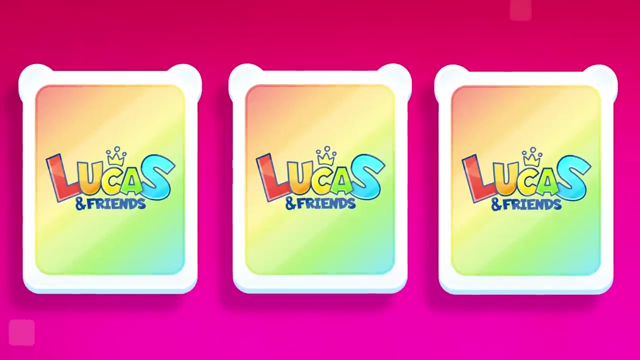 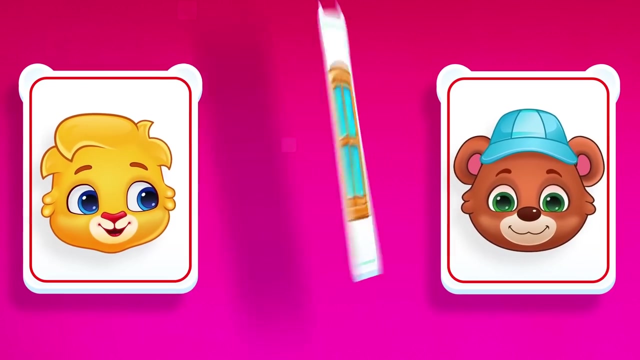 Circle, Circle, Circle Circle, Sun Ball, Donut Donut Circle. Circle Circle. The shape of a hula hoop is a circle. Lucas is dancing with the hula hoop. Woo-hoo, Yeah, That was scary, tho, Lucas. lol, That's not interesting. Where's the ball in the air? 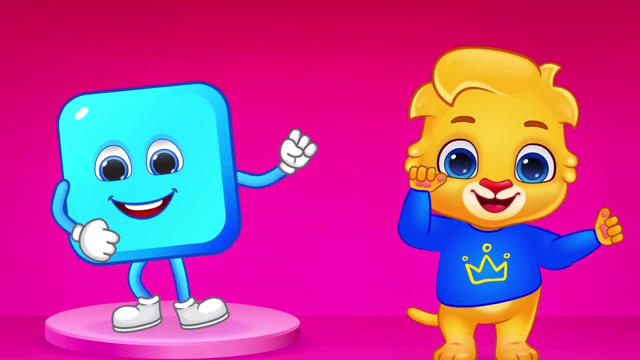 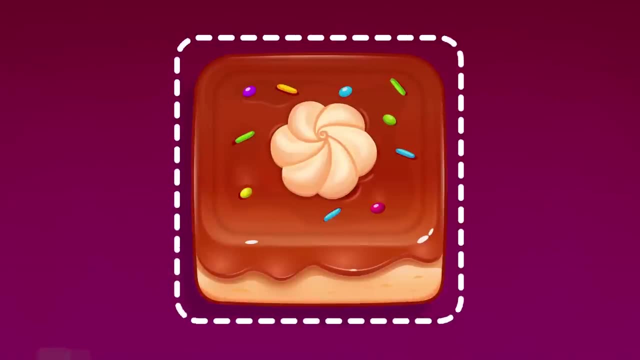 Where's the ball in the air There? Where's the ball in the air There? aspirations, Wow, While changing styles, Looking funny. SOC DO with 하는. Actually, this is a flower For a competition. If you see any Kawaii器, It's the very base of the sun. 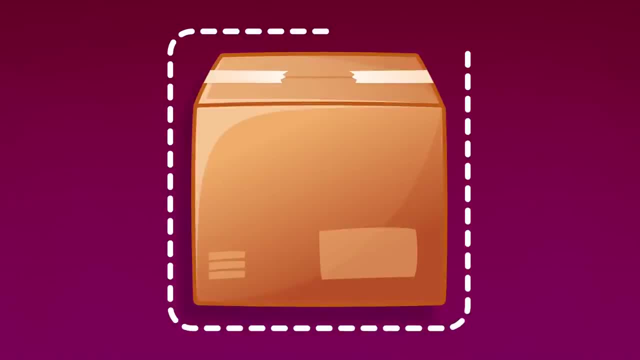 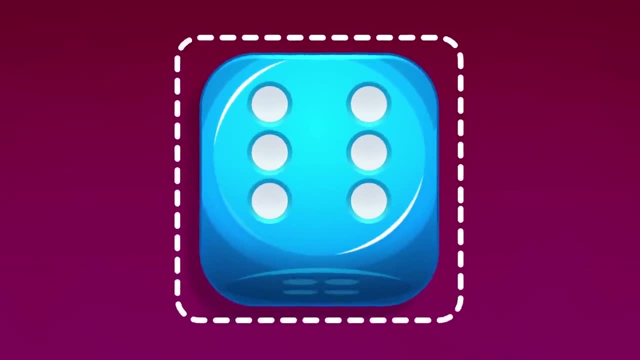 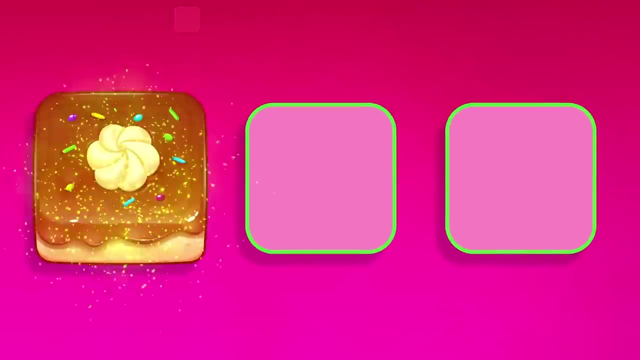 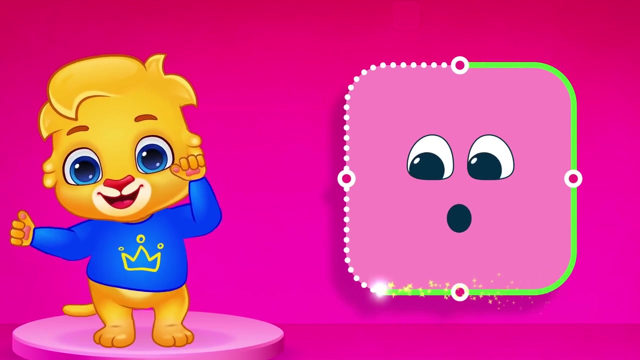 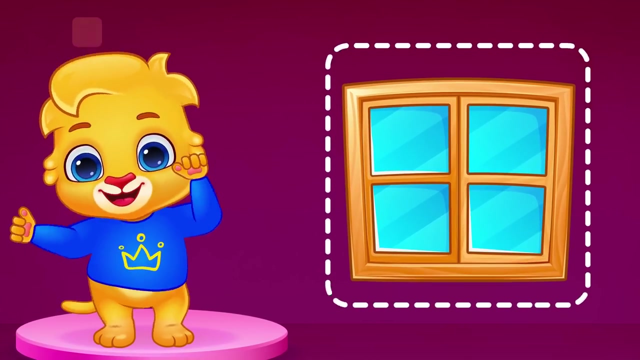 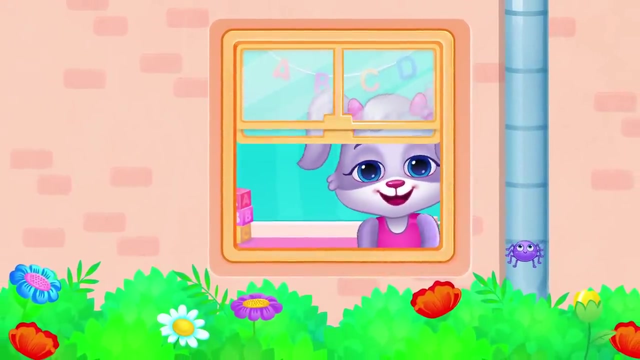 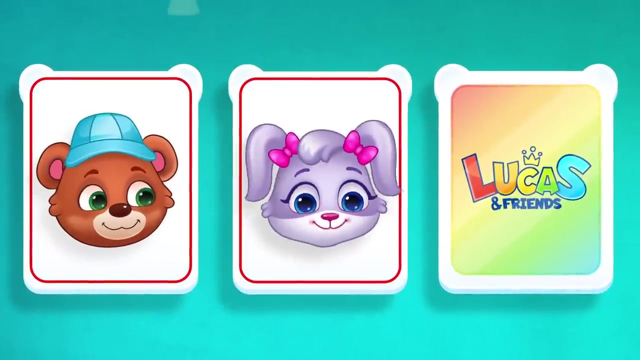 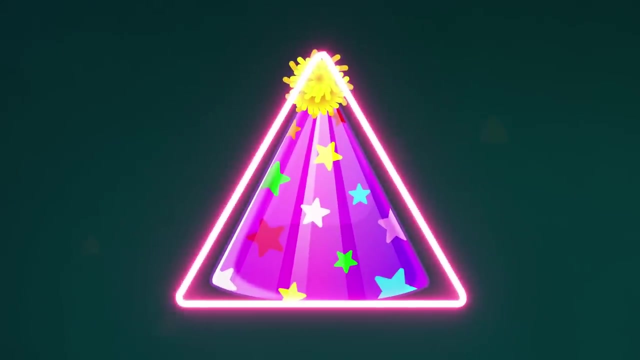 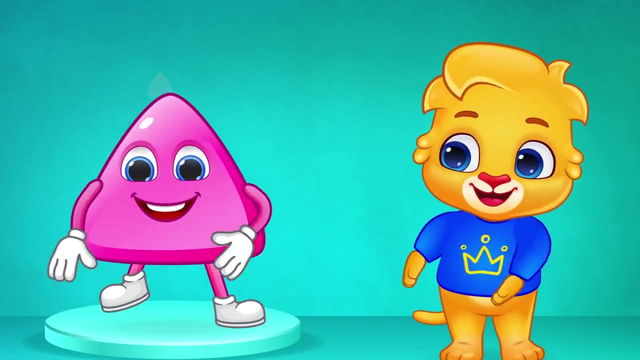 It's called Box box square. Dice dice square, Square, square, square. Cake box dice square, Square, square. This window has a square shape. Ruby is looking out the window. Cap cap, triangle, Triangle, triangle. This is 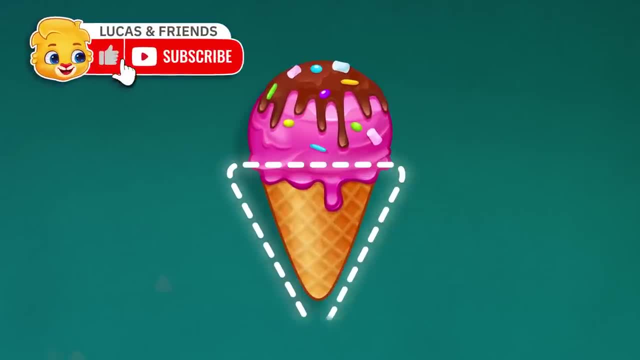 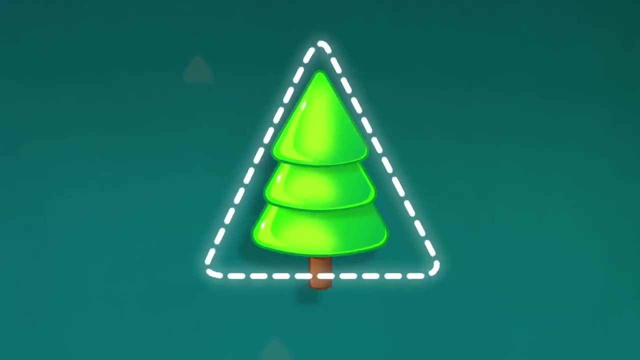 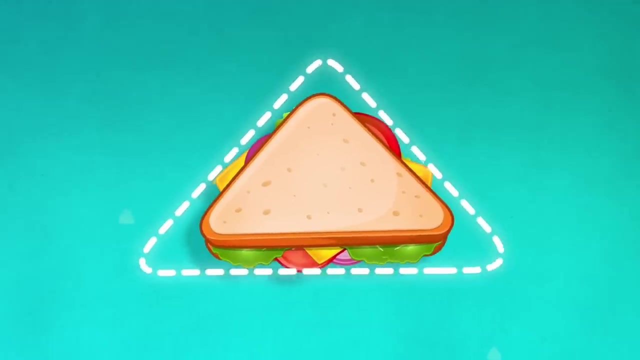 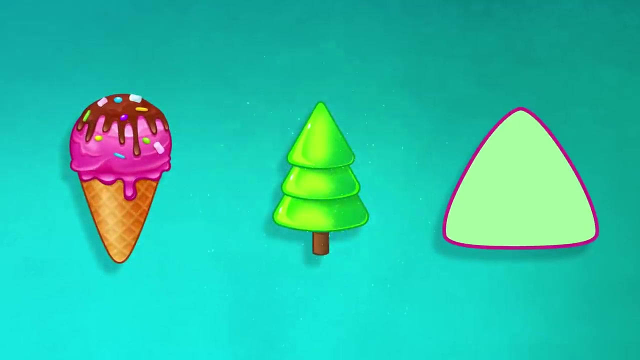 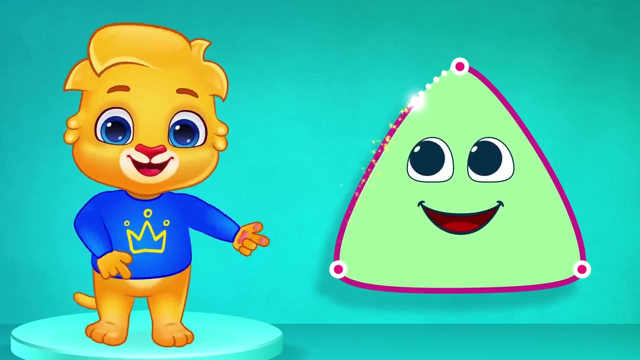 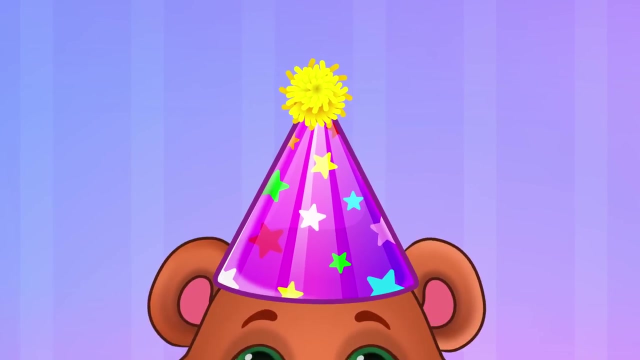 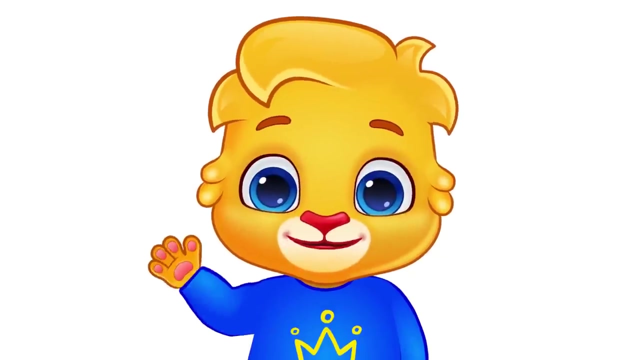 Triangle. Ice cream cone. ice cream cone- Triangle. Tree tree Triangle. Sandwich sandwich Triangle triangle triangle triangle. Ice cream cone- Tree sandwich Triangle. Triangle triangle. A birthday cap looks like a triangle shape. Brody's wearing a birthday cap. Hi, I'm Lucas. 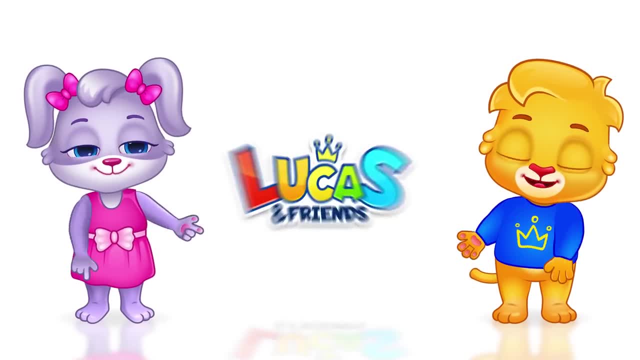 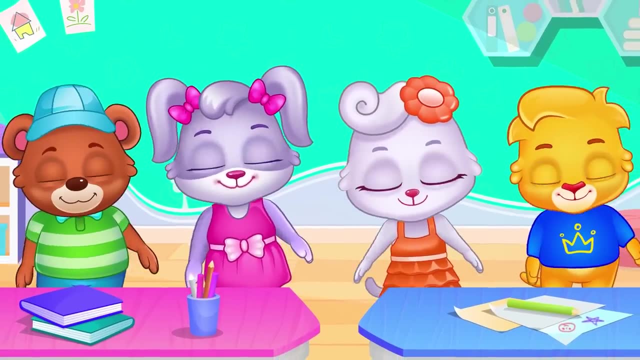 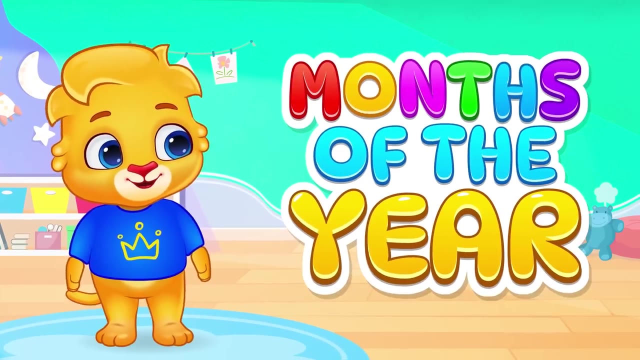 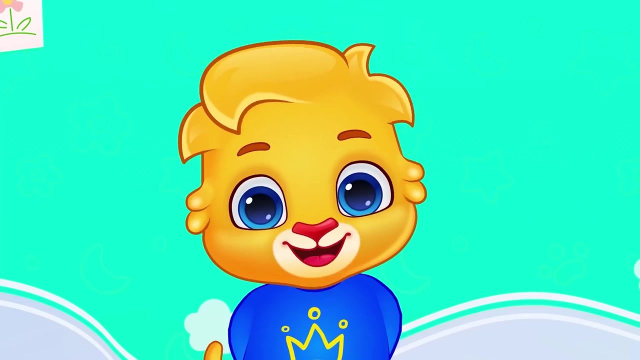 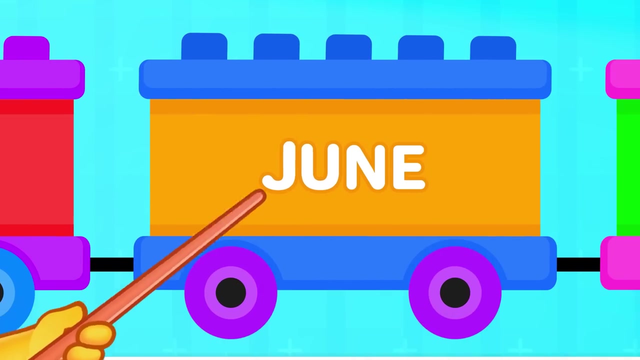 Hi, I'm Ruby And we're Lucas and Friends. Hi, kids, welcome to class. Hello, Can anyone guess what we're learning today? Let's go: January, February, March, April, May, June, July, August, September, October, November, December. May, June, July, August, September, October, November, December. 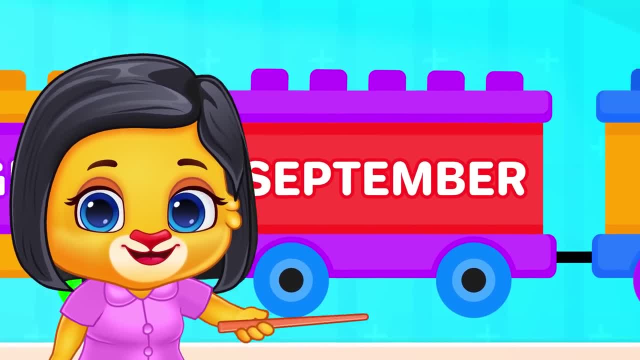 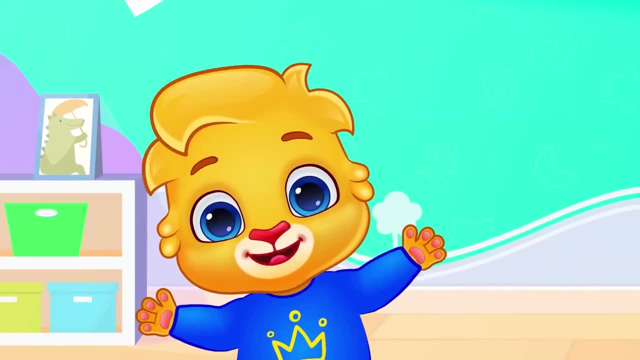 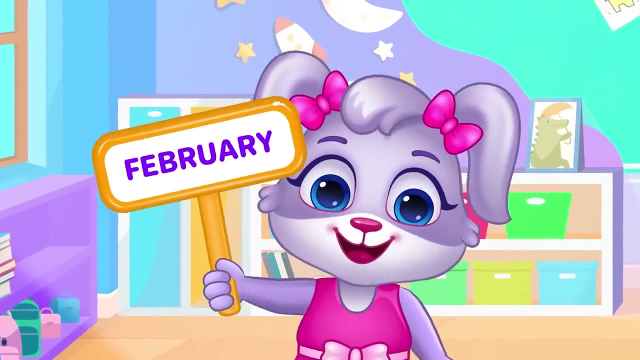 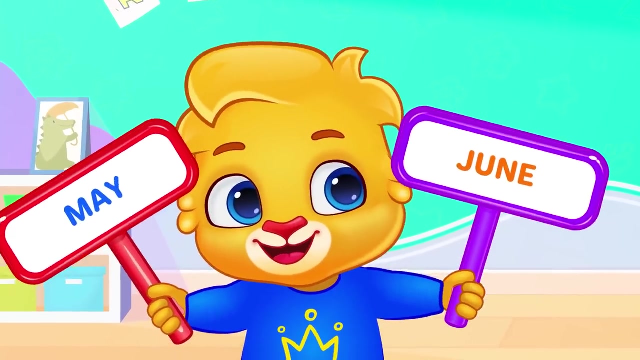 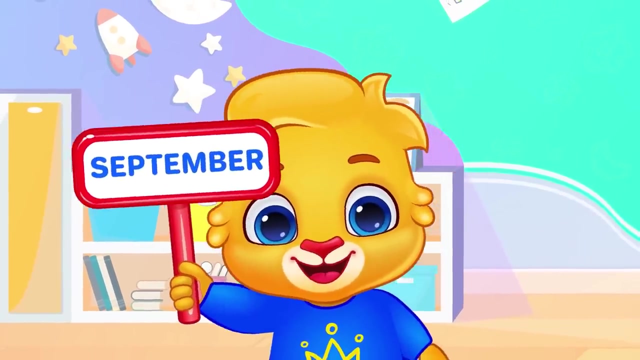 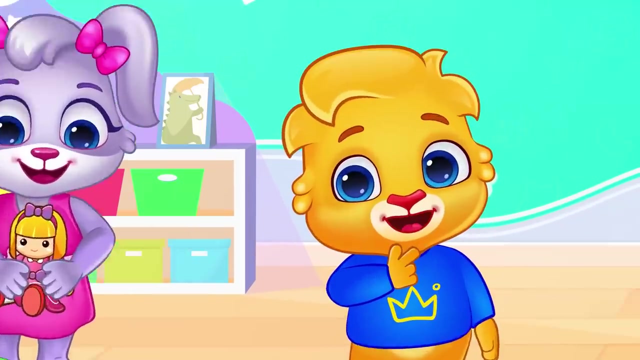 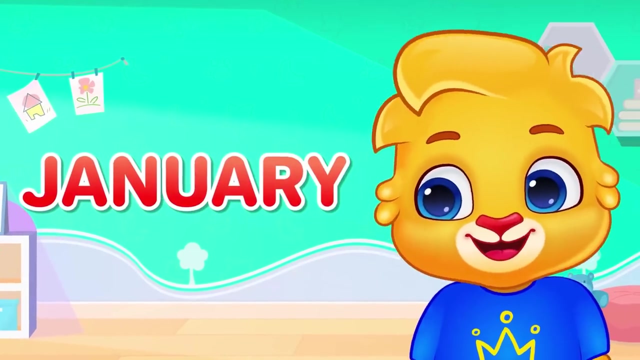 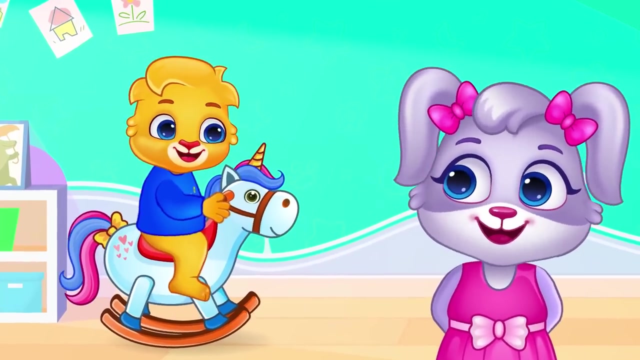 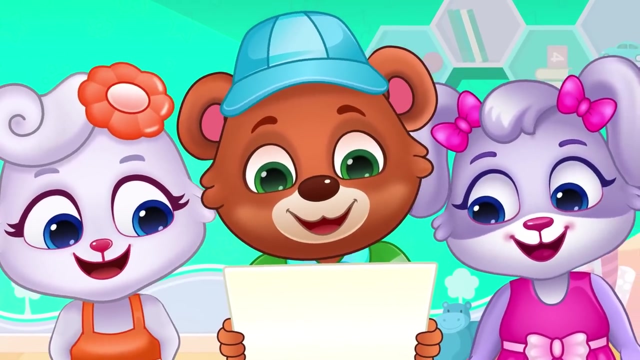 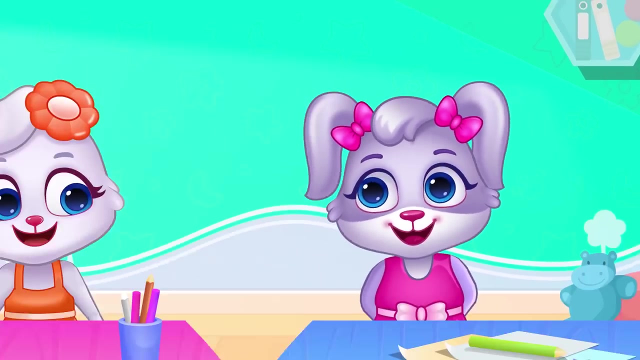 December, May, July, July, August, September, October, November, December. Let's say this again, Let's say this again: Yes, Yes, January, February, March, April, May, June, July, August, September, October, November, December. Hahaha, Can you repeat it with me? Yeah, January, February, March, April, May, June, July. 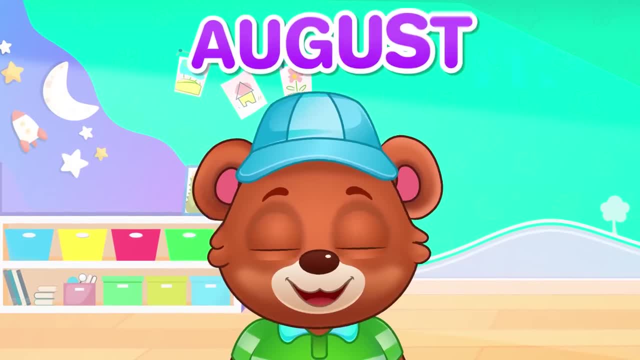 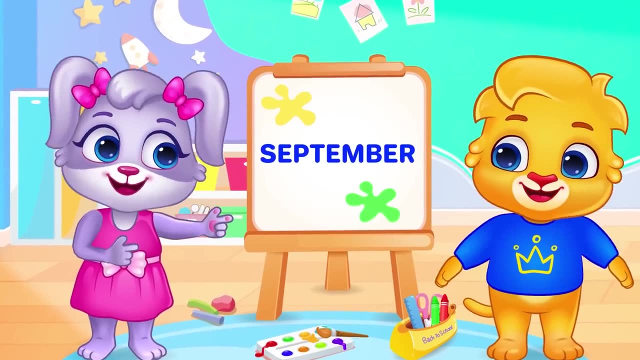 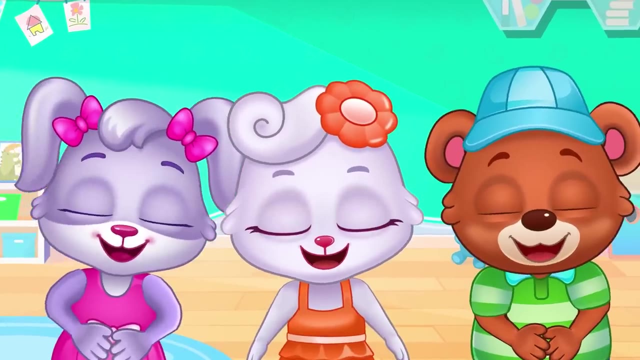 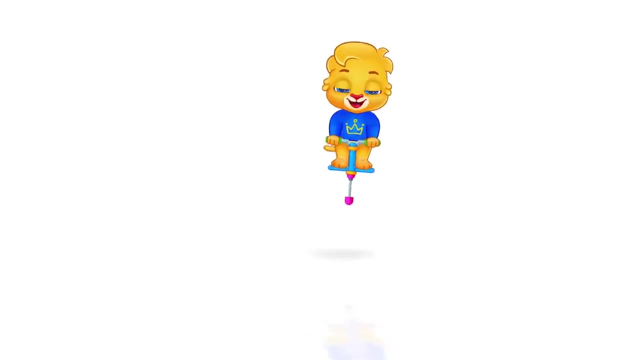 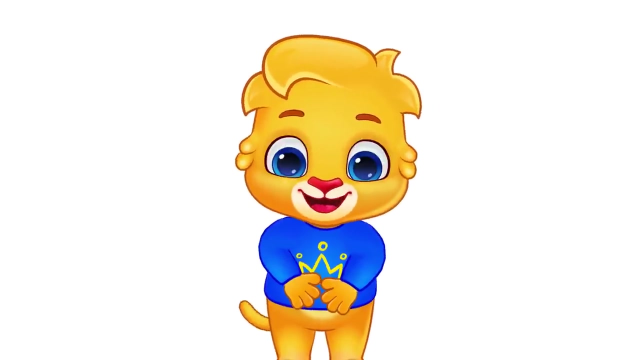 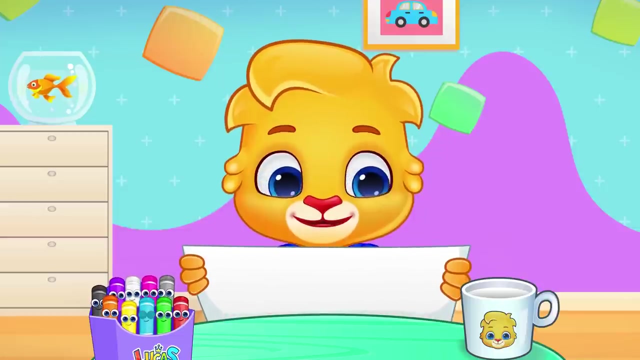 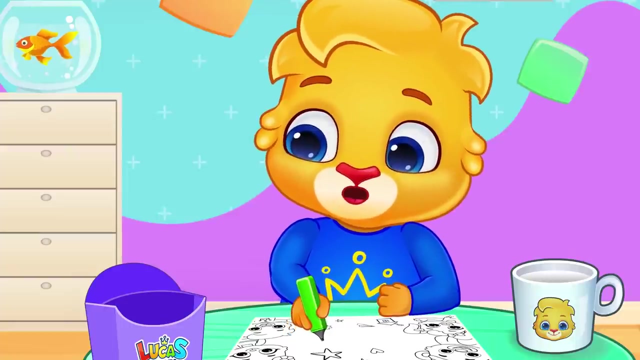 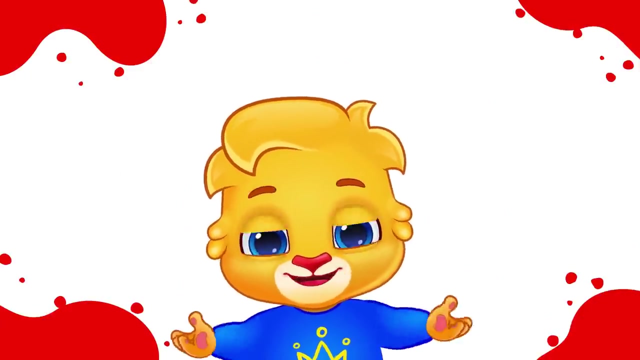 July, July, July, August, August, August, Hey, September, September, October, October, November, November, December, December, Hahaha, Woohoo, Hi, I'm Lucas. Hahaha, Papa, Hahaha, Oh, Oh, Hahaha, Hahaha, Red color, red color, where are you? 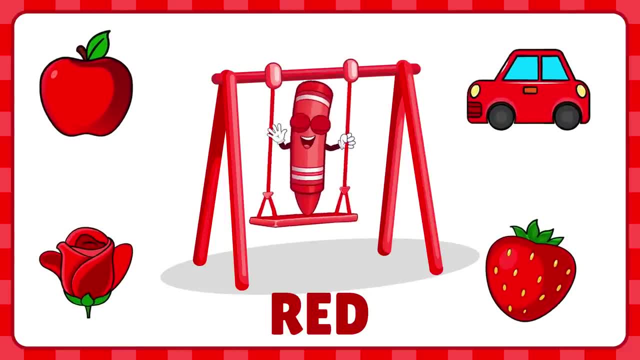 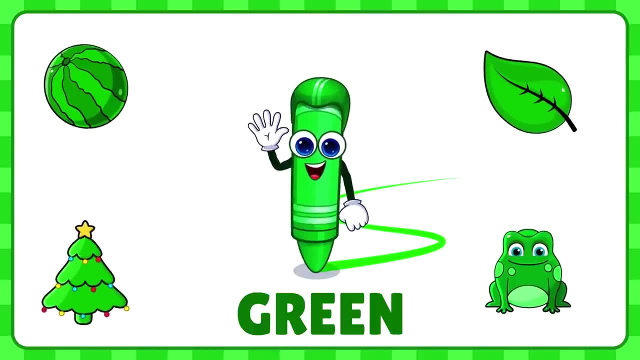 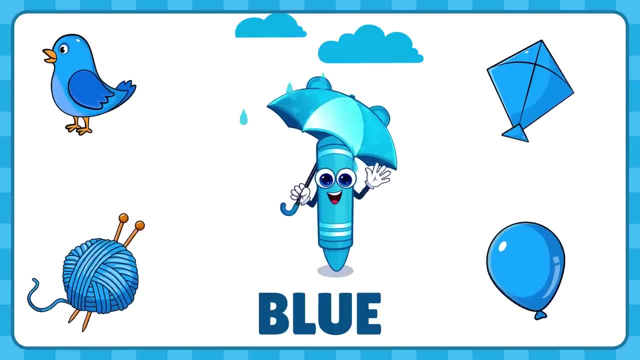 Here I am, here I am. how do you do Green color, green color- where are you Here? I am, here, I am. how do you do Blue color, blue color- where are you Here? I am, here, I am. how do you do. 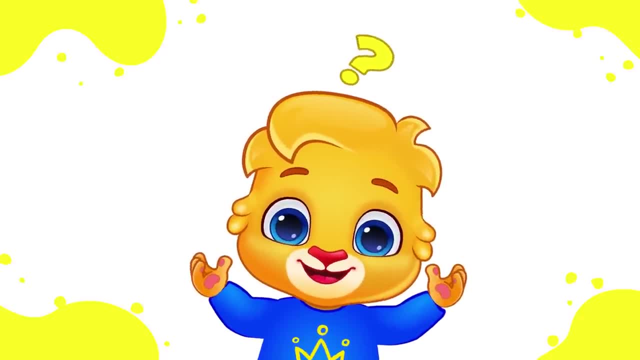 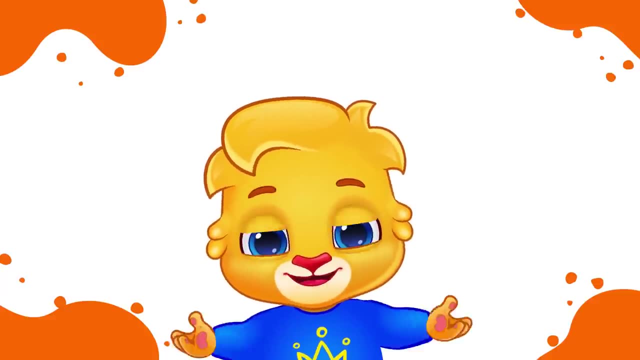 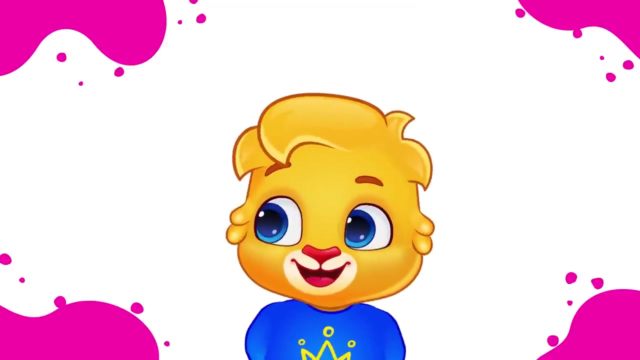 Yellow color, yellow color- where are you Here? I am here, I am. how do you do Orange color? orange color: where are you Here? I am here, I am. how do you do Pink color, pink color- where are you? 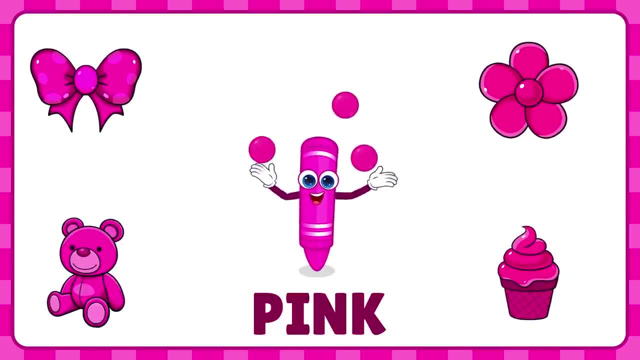 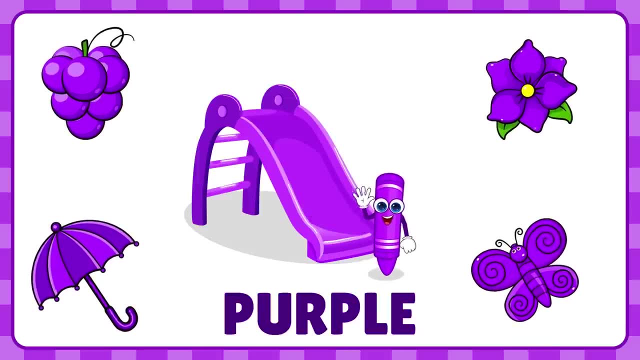 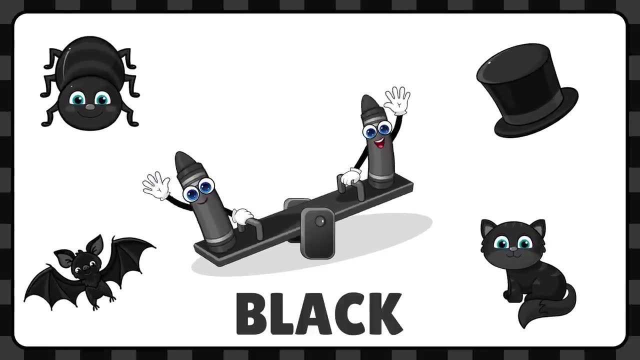 Here I am, here I am. how do you do Purple color, purple color- where are you Here? I am, here, I am. how do you do Black color, black color- where are you Here? I am, here, I am. how do you do. 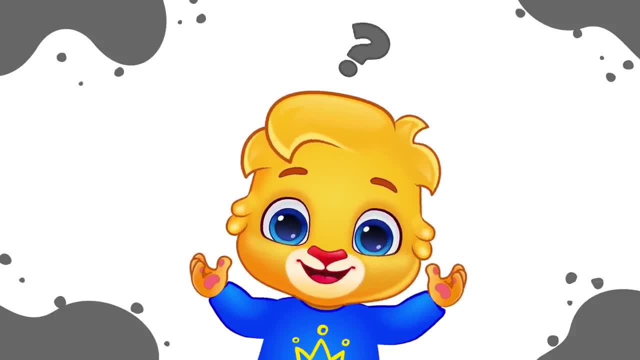 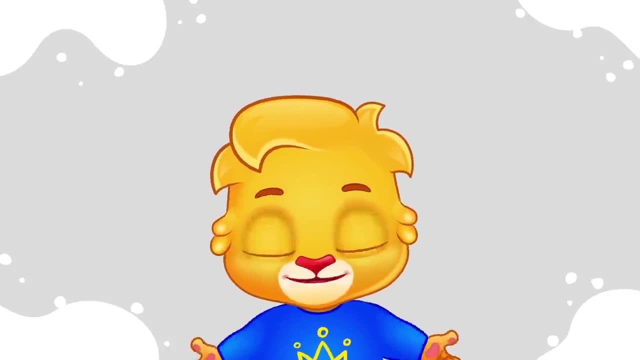 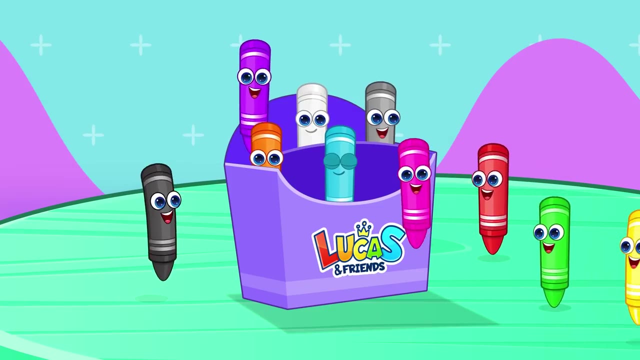 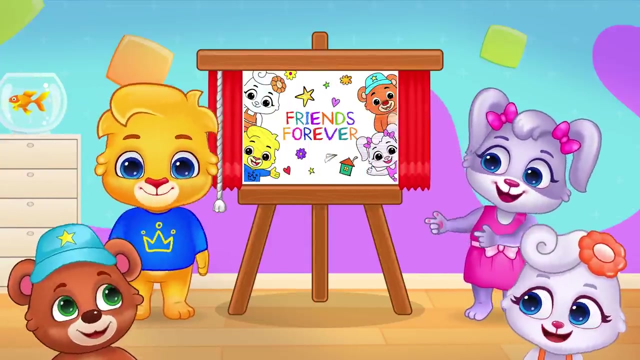 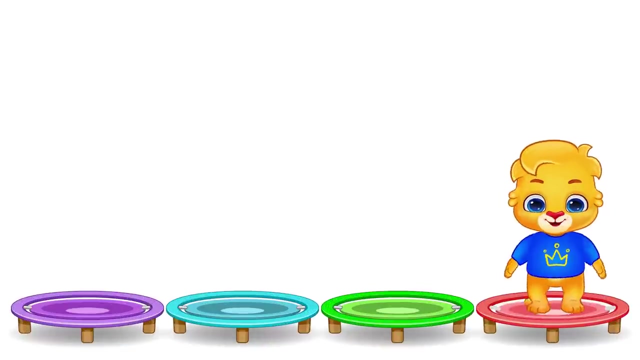 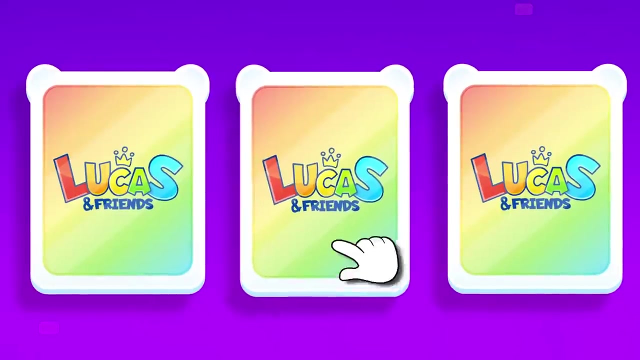 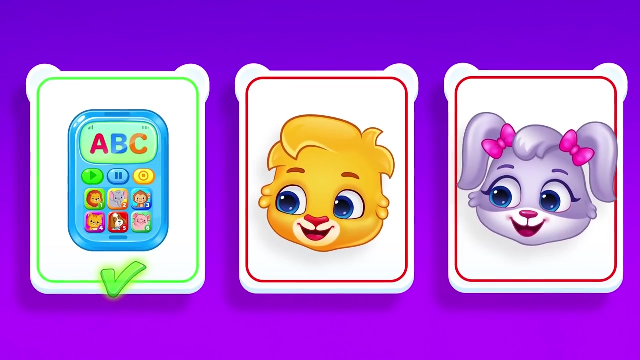 Gray color- gray color. where are you Here? I am here, I am. how do you do White color, white color: where are you Here? I am here, I am. how do you do Yeah, Yeah Phone. 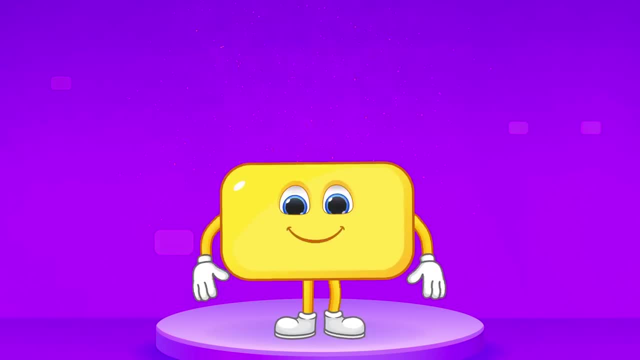 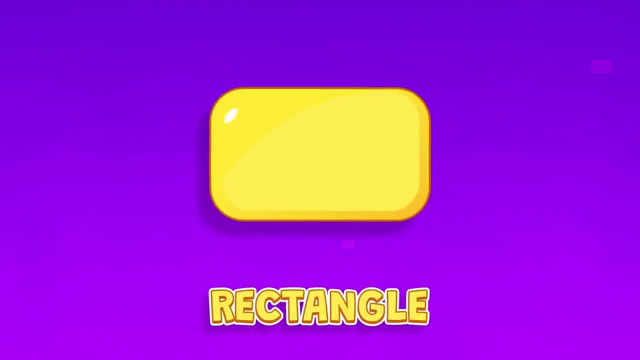 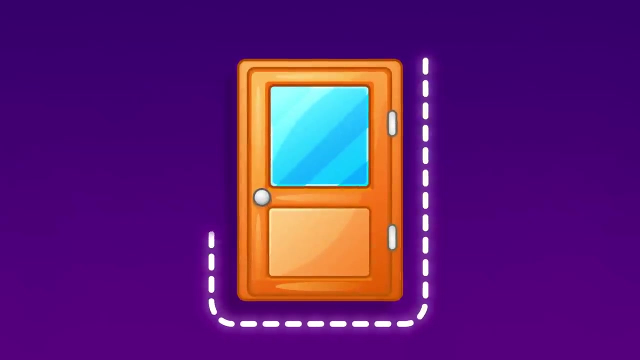 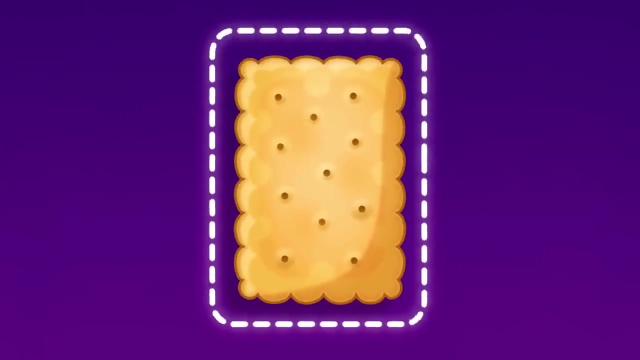 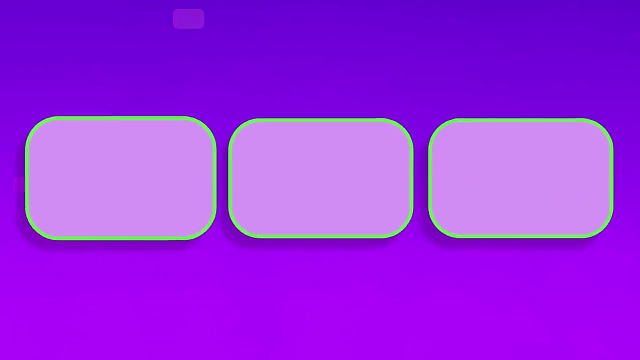 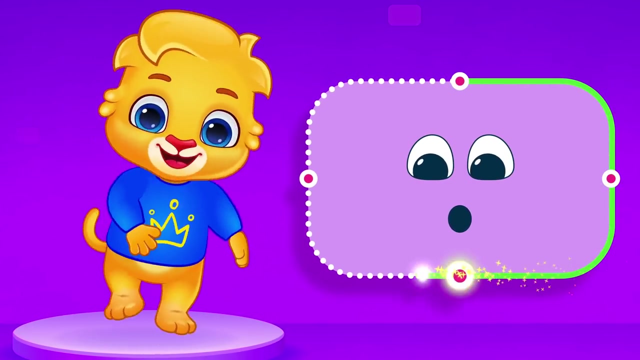 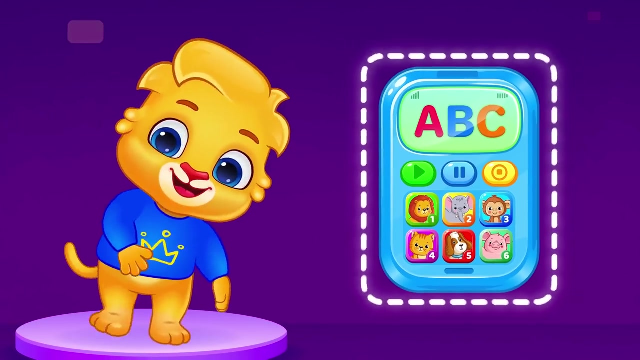 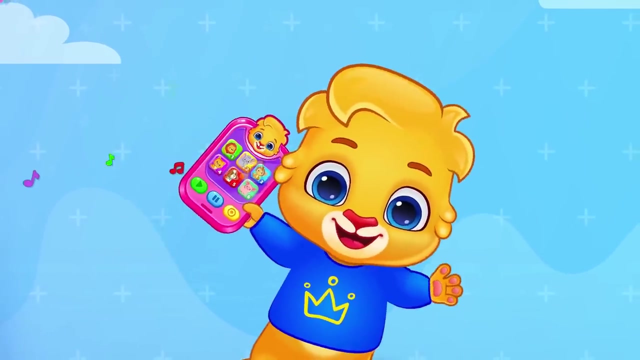 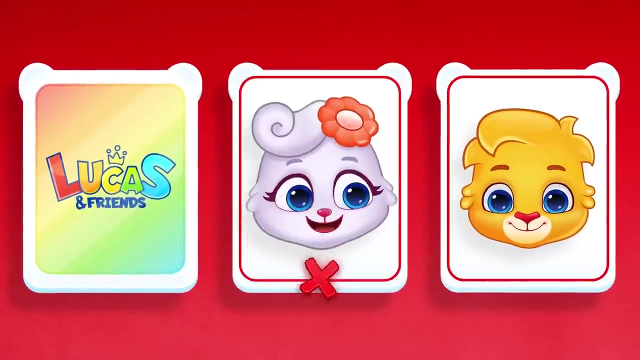 Phone Rectangle, Rectangle, Rectangle. This is rectangle Bag Bag Rectangle, Door Door Rectangle, Biscuit, Biscuit Rectangle, Rectangle, Rectangle Bag Door, Biscuit Rectangle. Wow, Rectangle, Rectangle. The shape of a phone is a rectangle. Lucas is playing music on the phone, Woohoo. 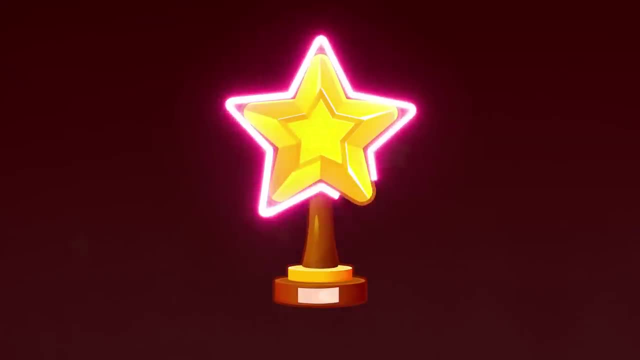 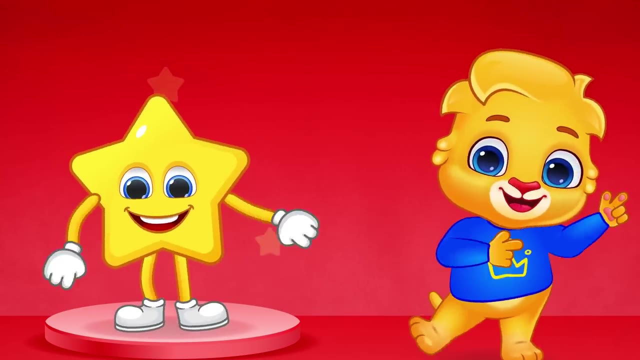 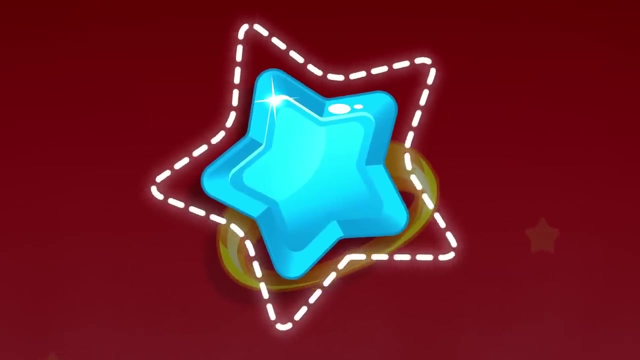 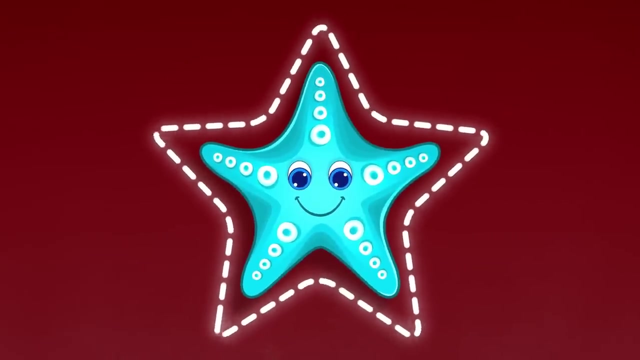 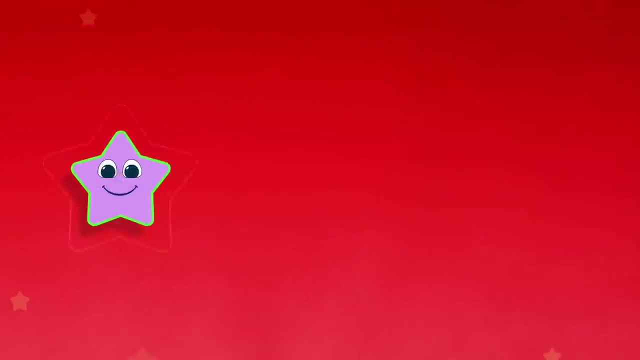 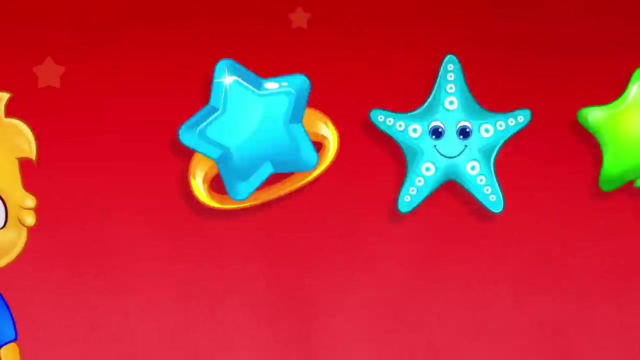 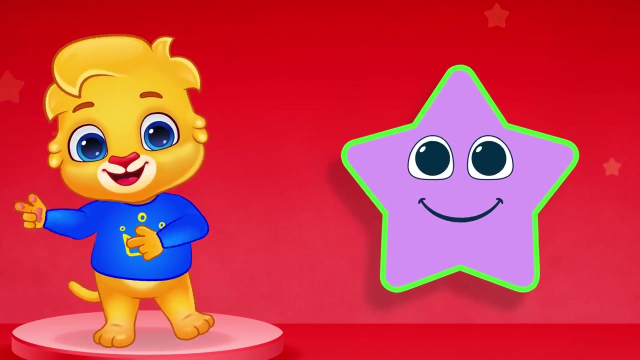 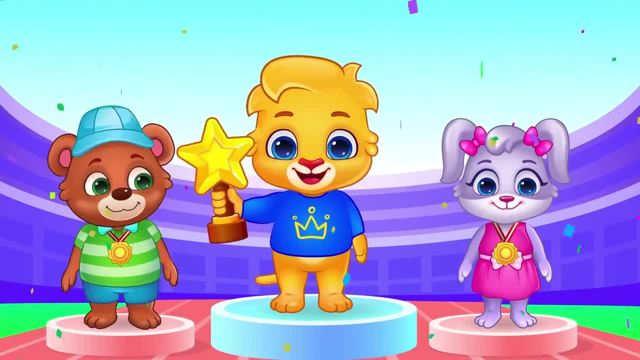 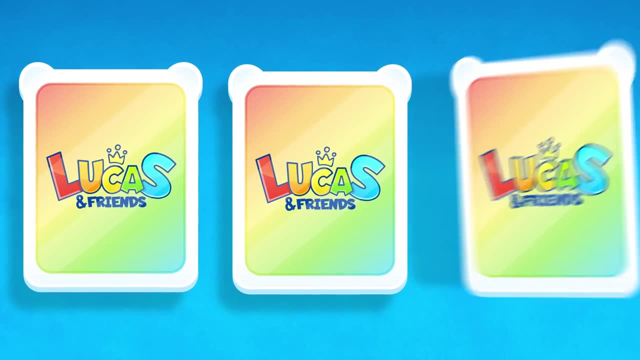 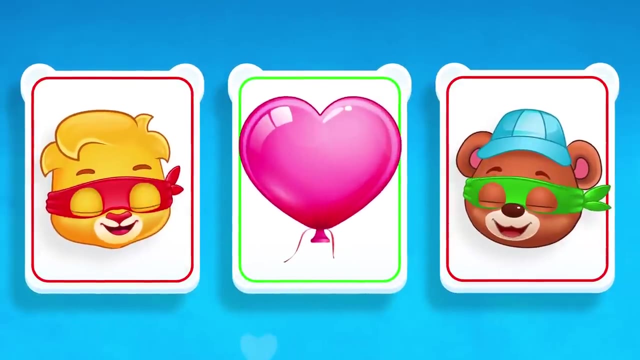 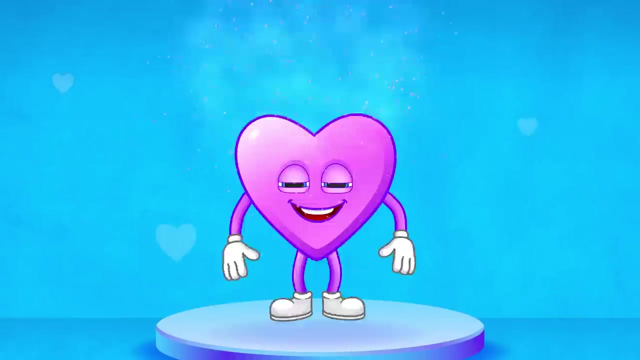 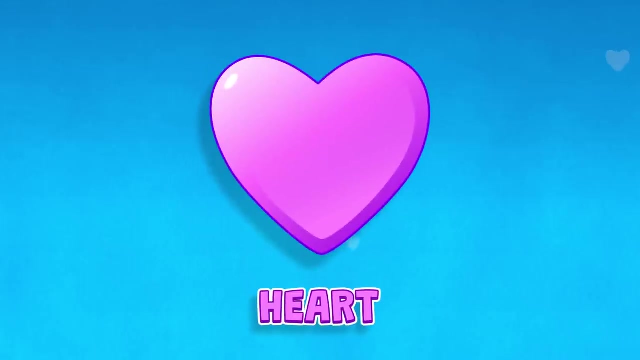 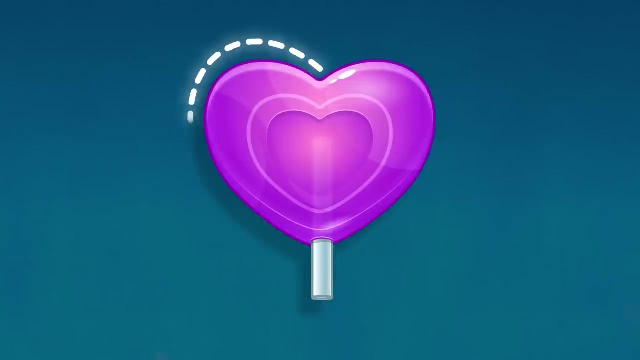 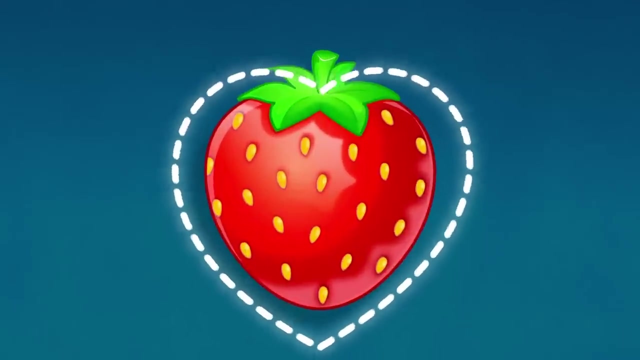 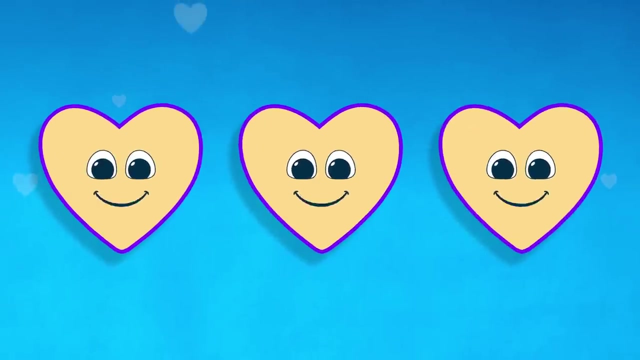 Lucas won the star-shaped trophy in a tournament Balloon Balloon: Heart, Heart, Heart. This is Heart Leaf Leaf, Heart Candy, Candy, Heart Strawberry, Strawberry, Heart, Heart, Heart, Heart Leaf Candy. 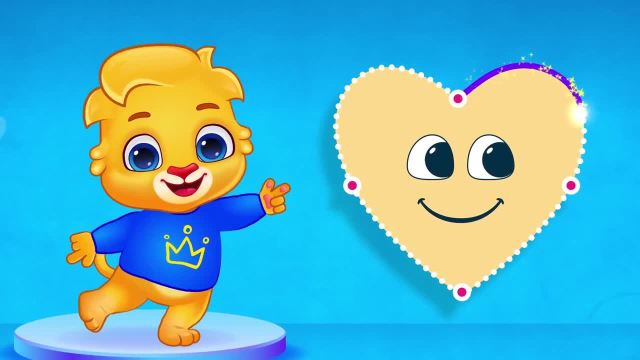 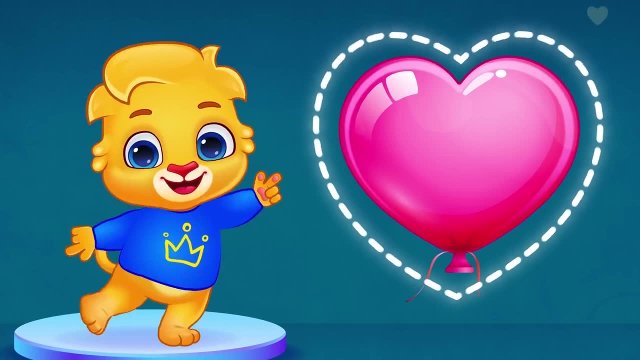 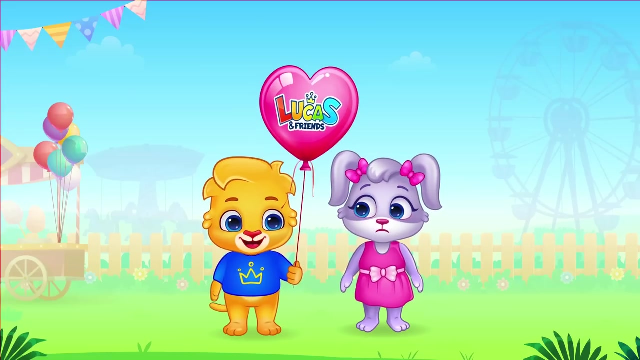 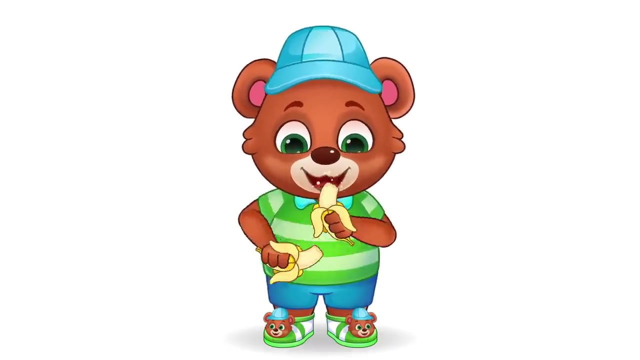 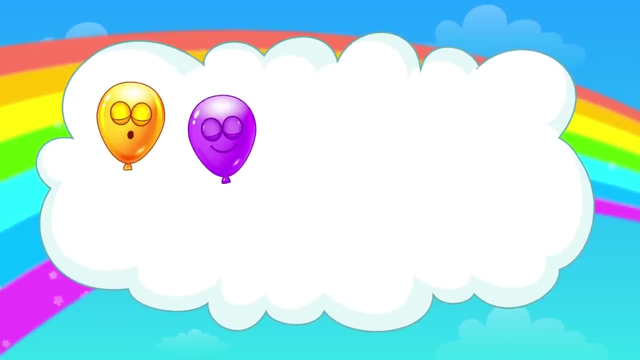 Strawberry Heart, Heart, Heart. This balloon has a heart shape. Lucas popped the balloon. Yeah, Uh-huh, Wow scatter Like this. One, Two, Three, Four, Five, Six, Seven, Eight, Nine, TEN. 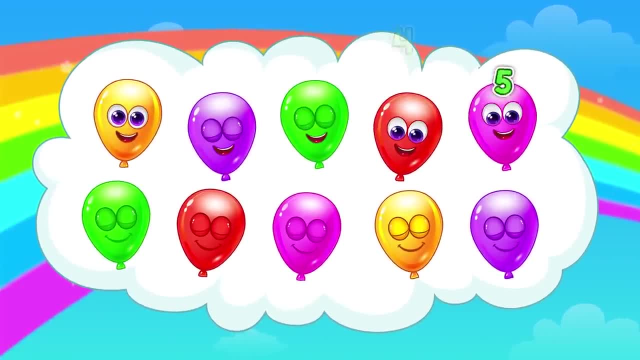 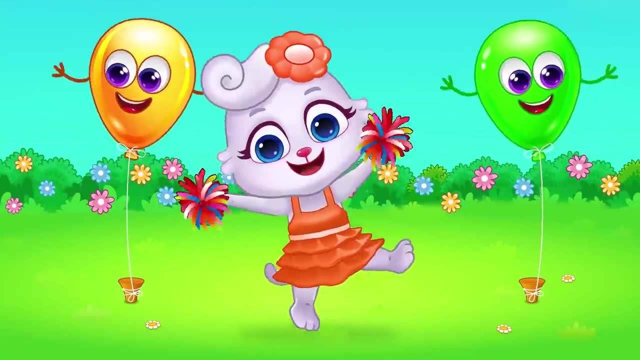 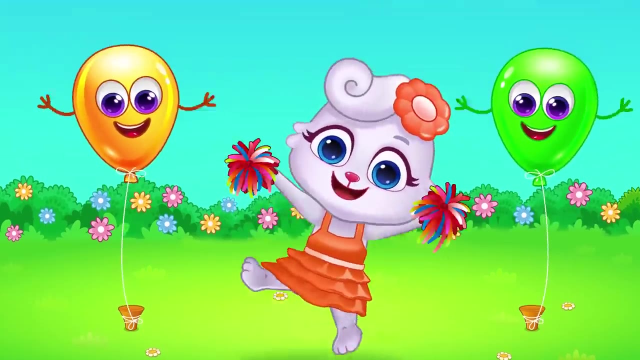 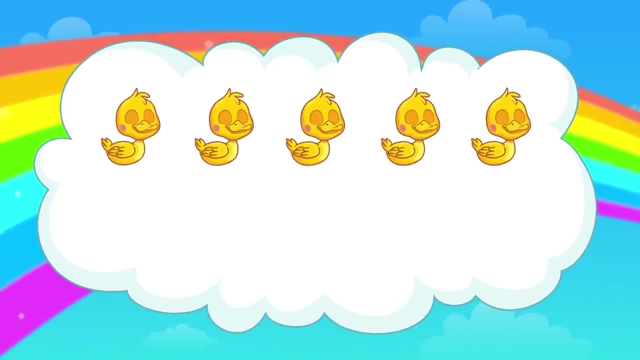 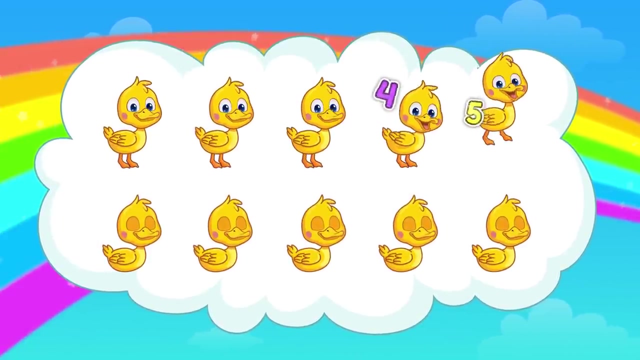 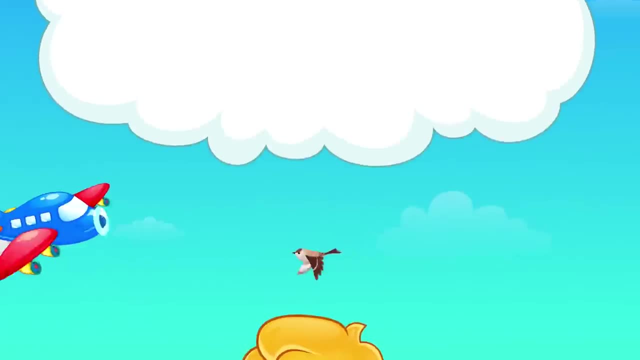 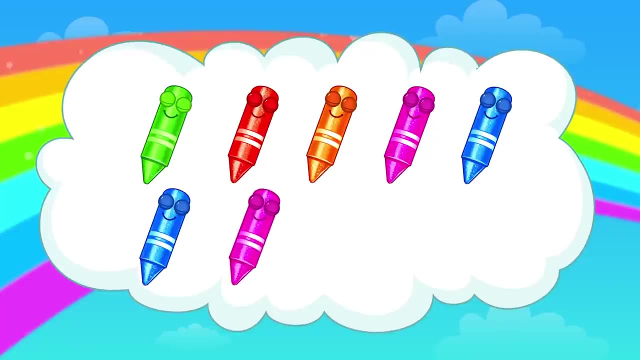 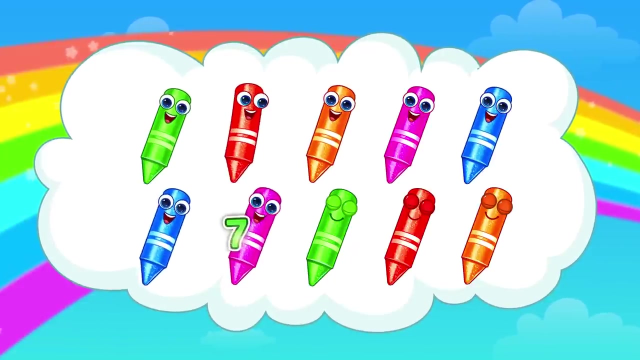 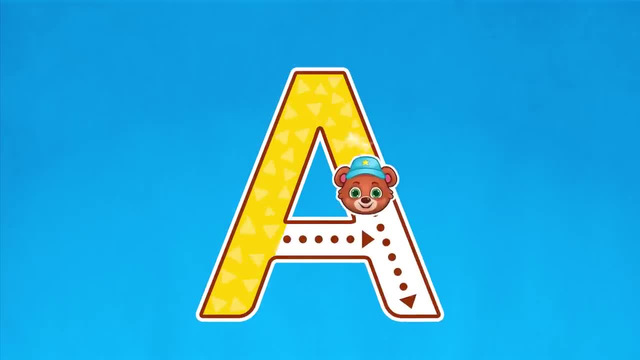 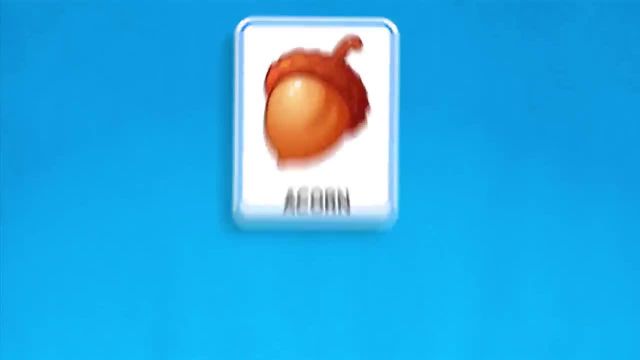 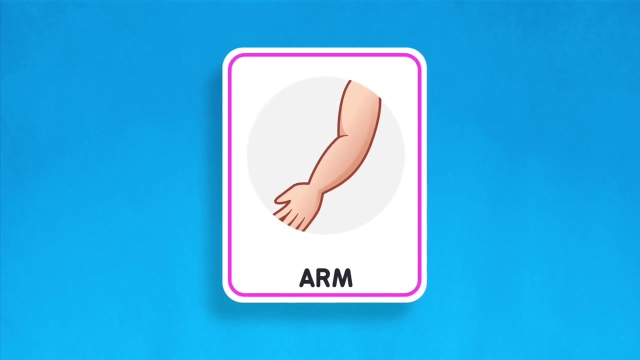 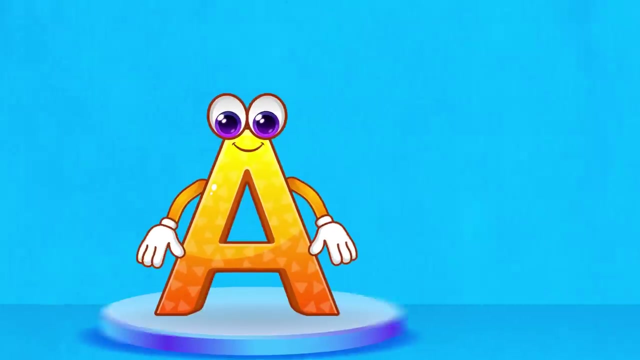 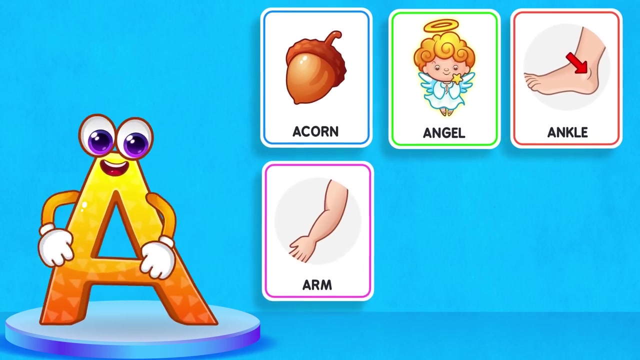 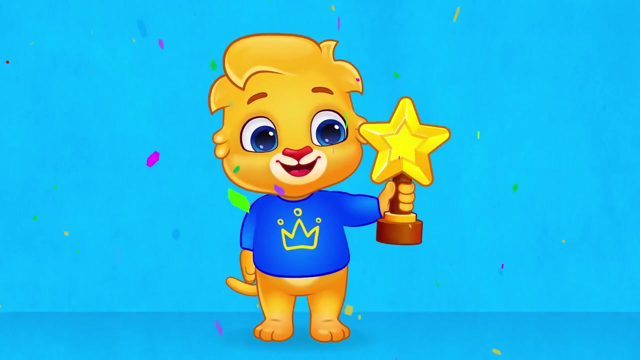 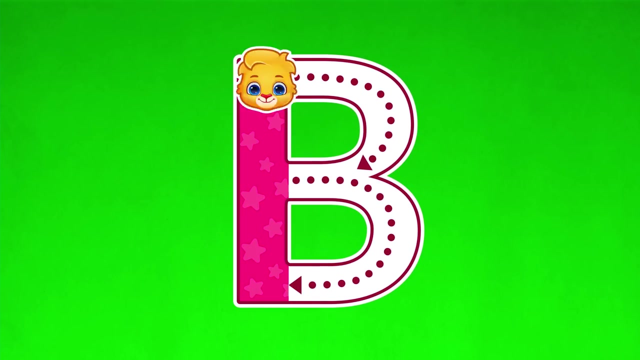 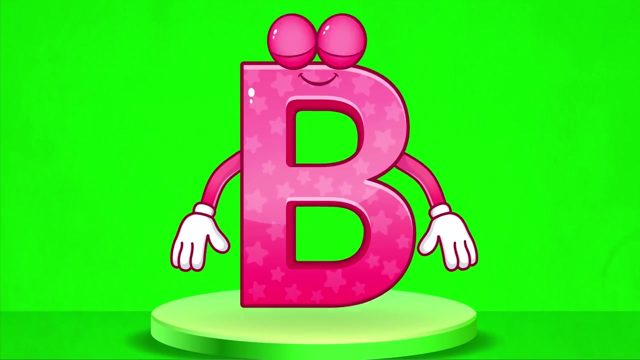 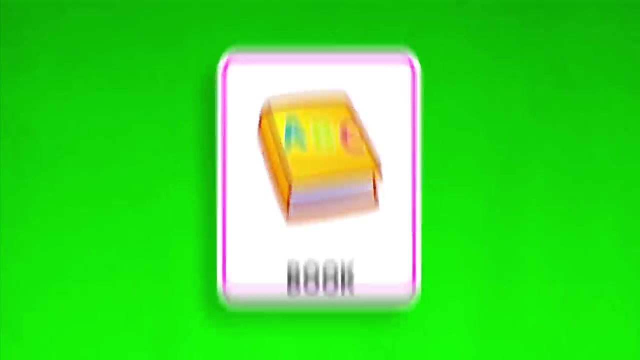 A. This is A. A is for acorn Angel Ankle Arm Arrow Award. This is A. A is for acorn Angel Ankle Arm Arrow Award. Yeah, B, B, This is B. B is for balloon, Bear, Biscuit, Book, Broccoli, Butterfly. 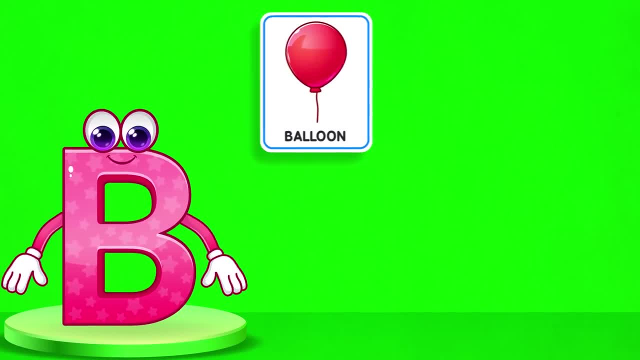 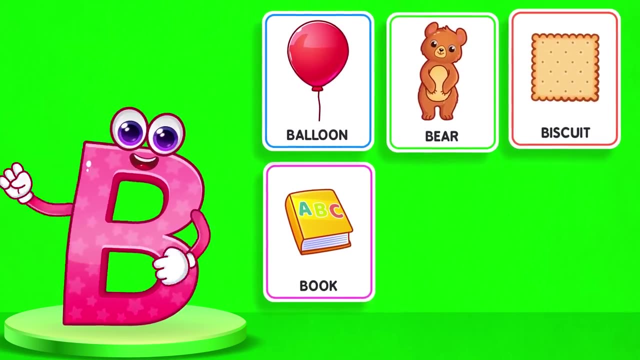 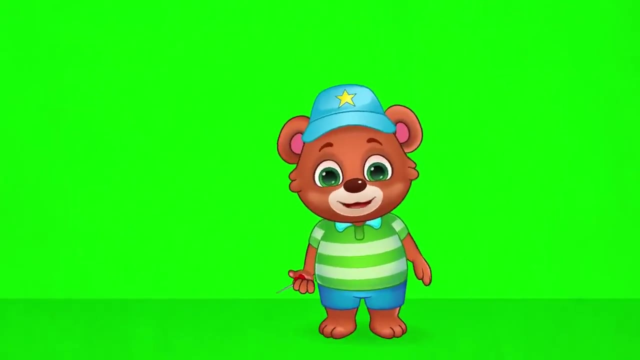 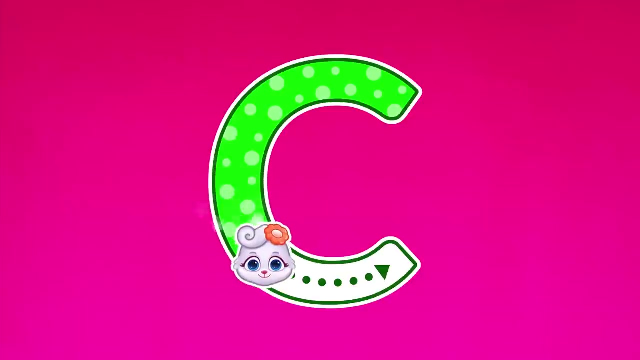 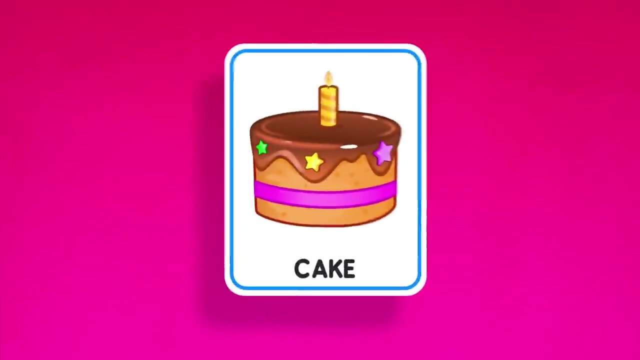 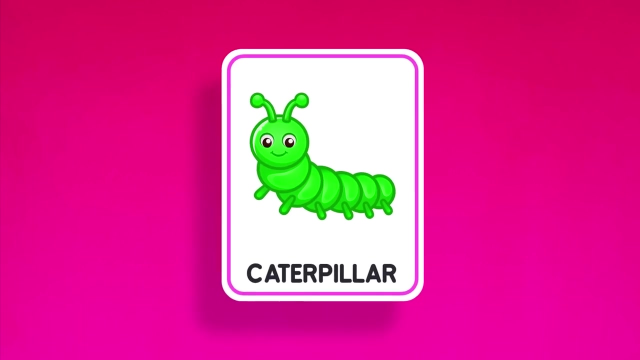 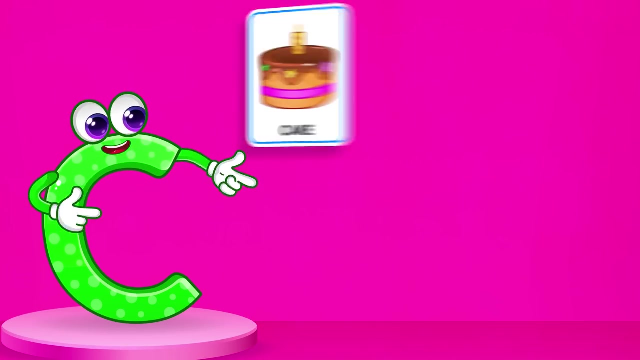 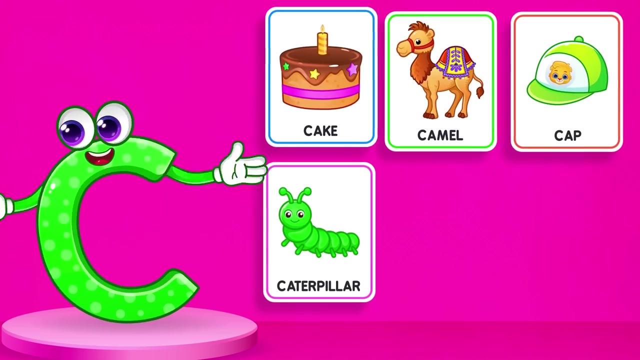 This is B. B is for balloon, Bear, Biscuit, Book, Broccoli, Butterfly, Woohoo, C. This is C. C is for cake: Camel Cap, Caterpillar Coconut Cookies. This is C. C is for cake: Camel Cap, Caterpillar Coconut Cookies. 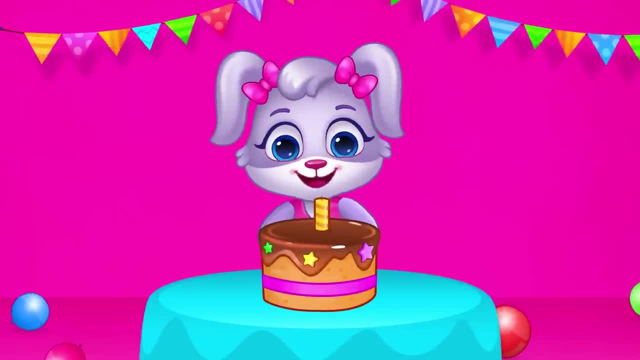 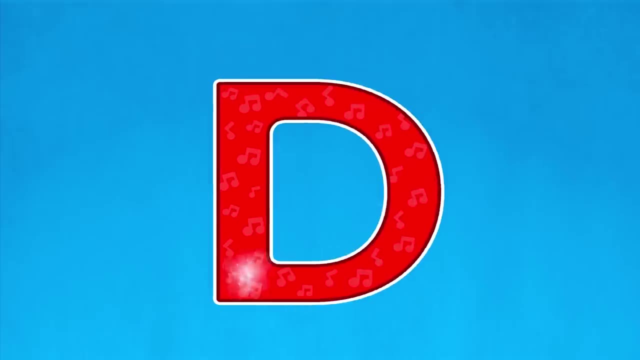 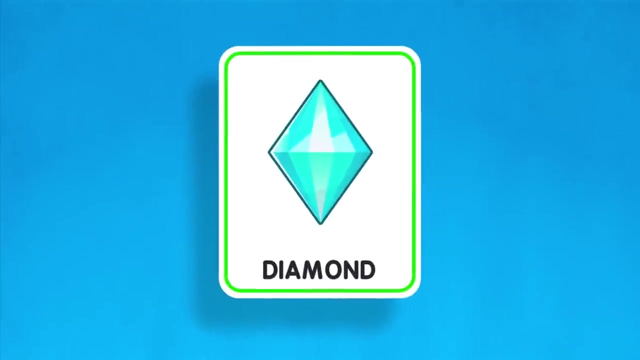 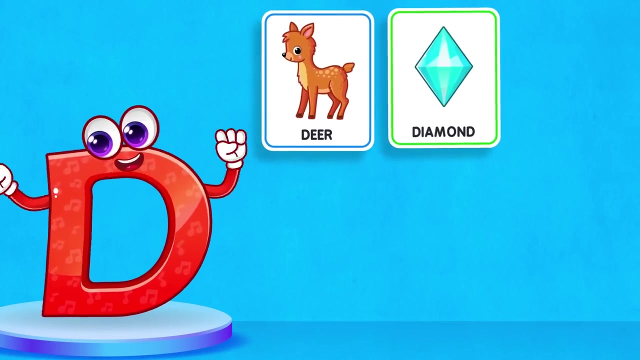 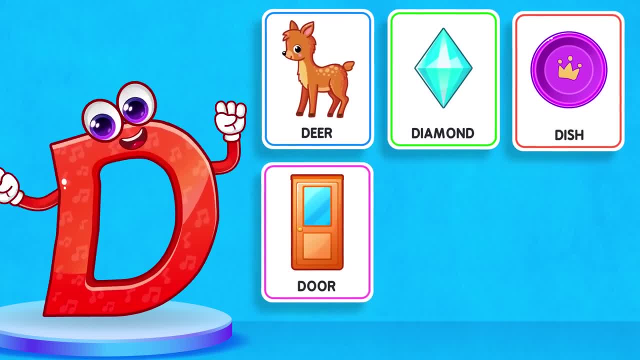 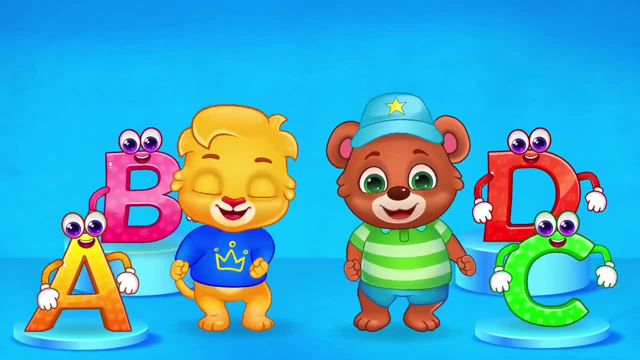 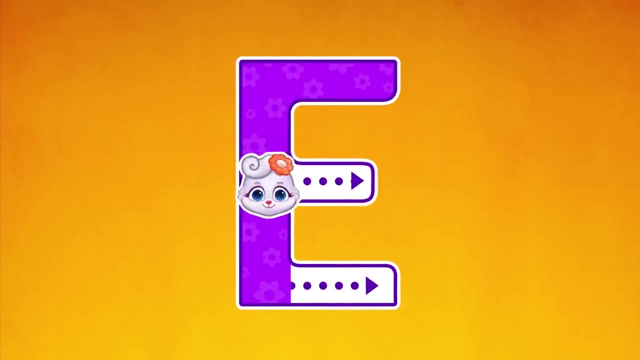 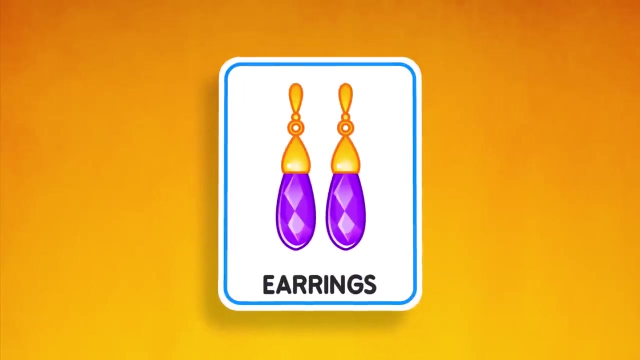 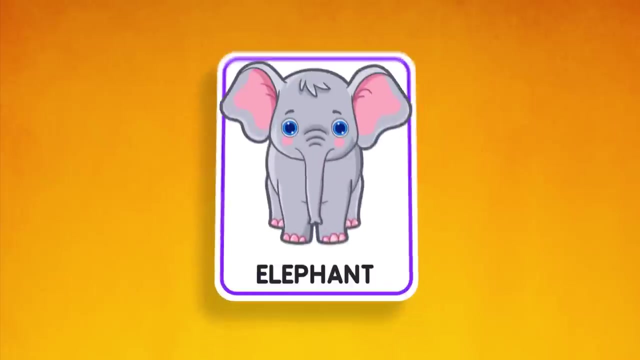 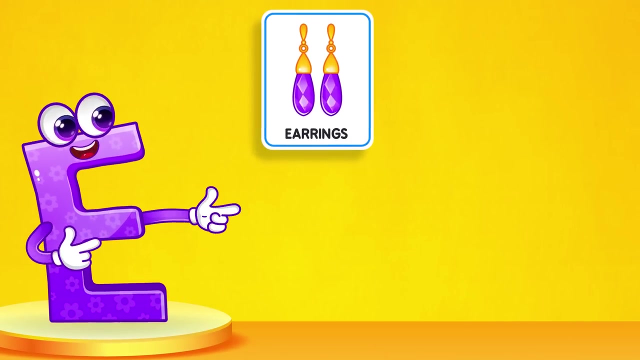 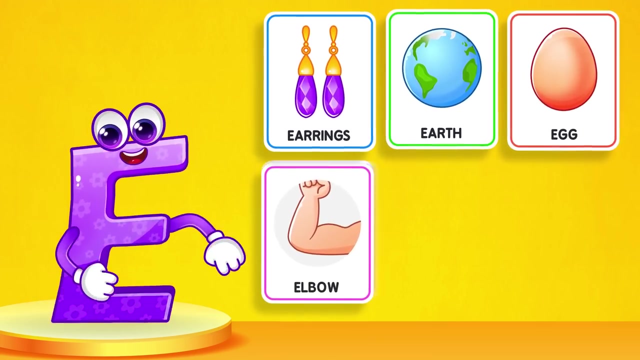 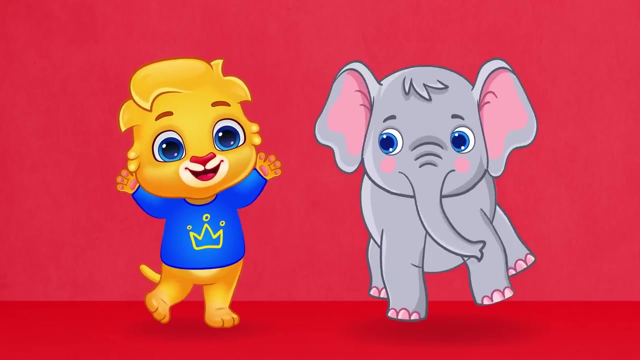 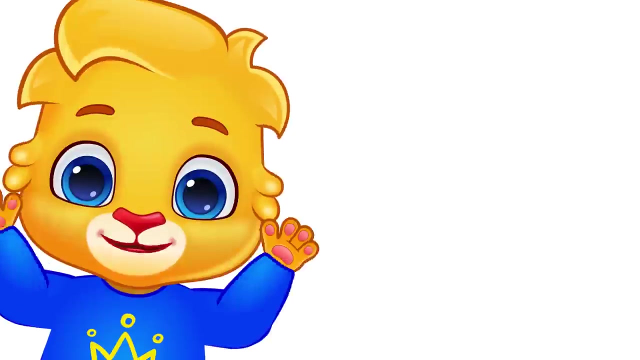 D, D, D D. Doughnut Dove E. This is E. E is for Earrings Earth Egg Elbow Elephant Eraser. This is E. E is for Earrings Earth Egg Elbow Elephant Eraser. Peek-a-boo, Peek-a-boo. 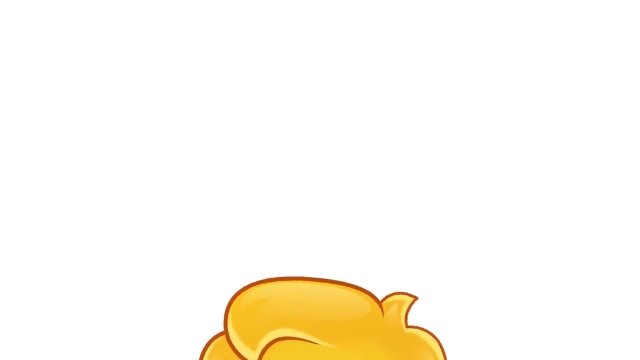 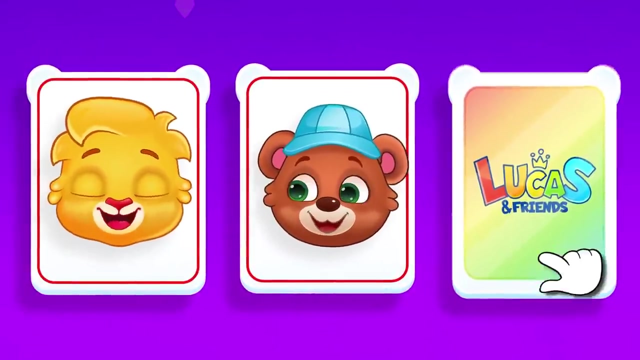 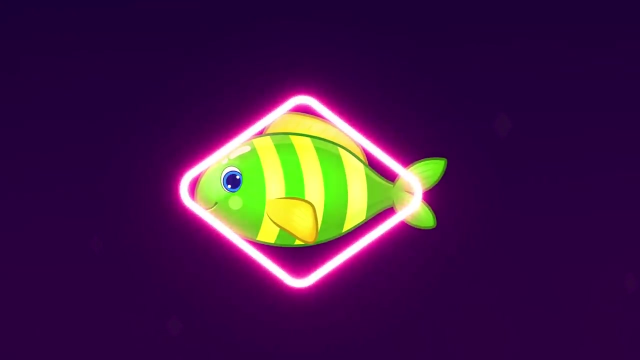 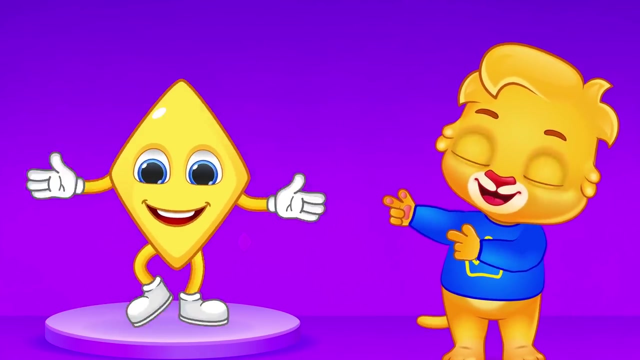 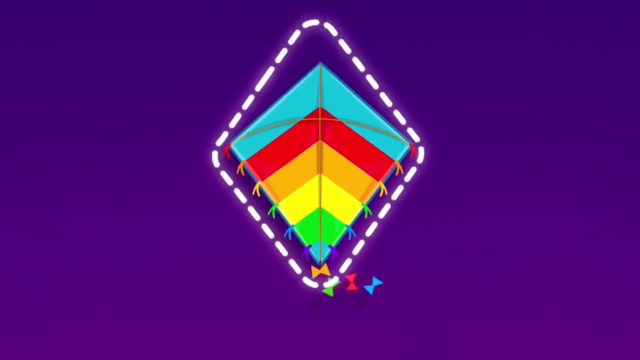 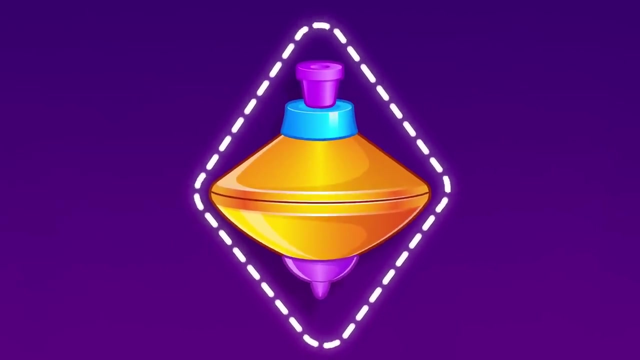 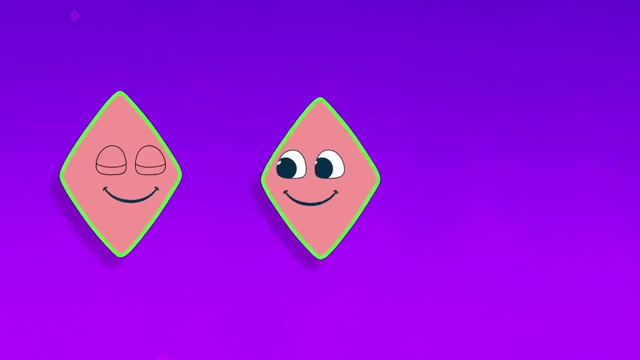 Peek-a-boo, Peek-a-boo Fish Fish. Rhombus, Rhombus, Rhombus. This is Rhombus. This is Rhombus. Kite, Kite. Rhombus. Toy Toy. Rhombus- Diamond Diamond. Rhombus, Rhombus, Rhombus. 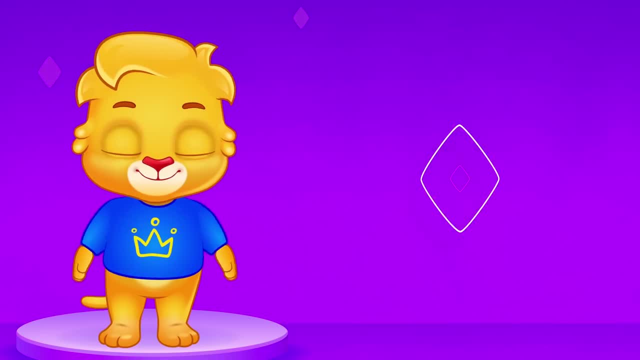 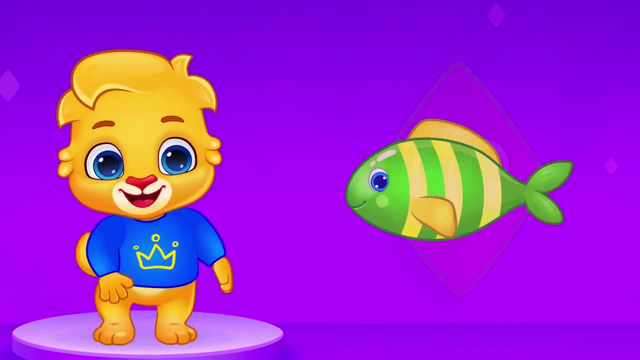 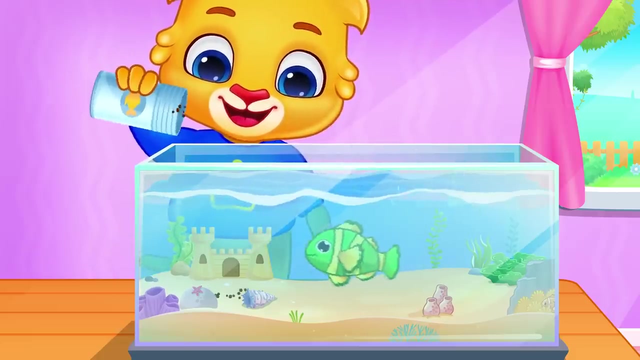 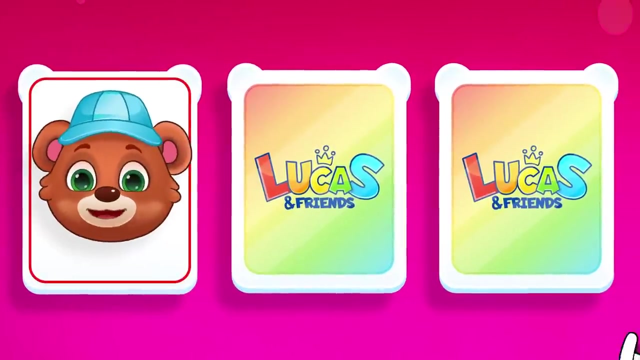 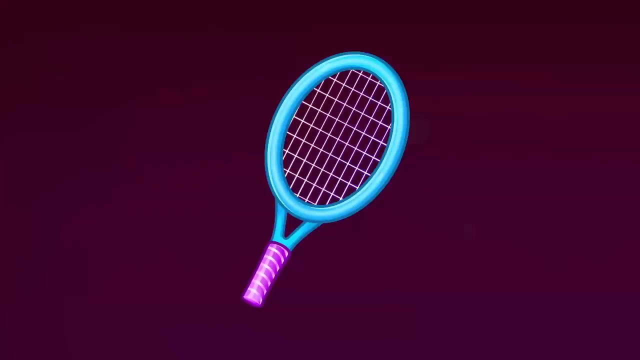 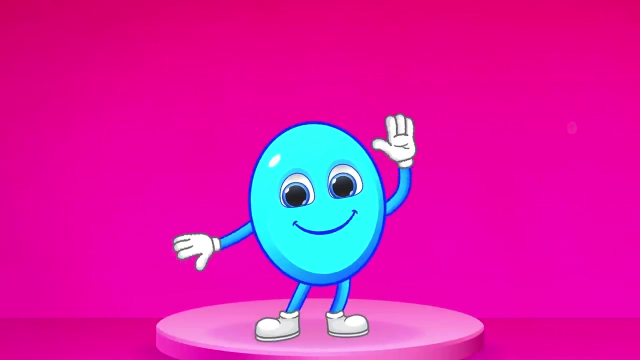 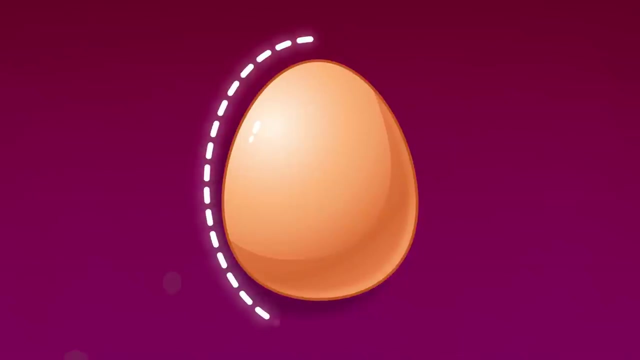 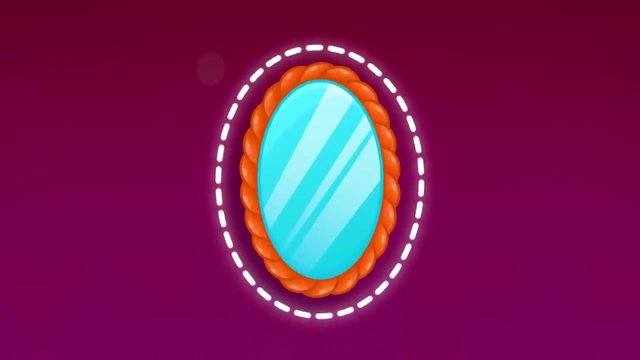 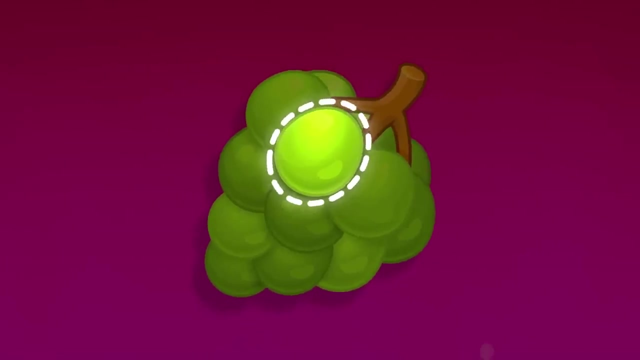 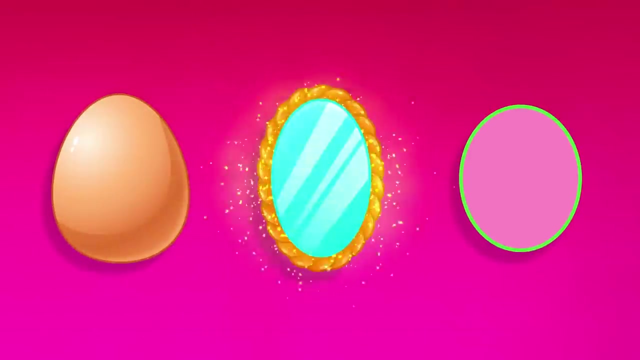 Kite Toy Diamond Rhombus, Rhombus, Rhombus Rhombus, Diamond Diamond. This is oval egg egg oval mirror mirror oval grapes, grapes, oval oval oval oval egg mirror grapes. 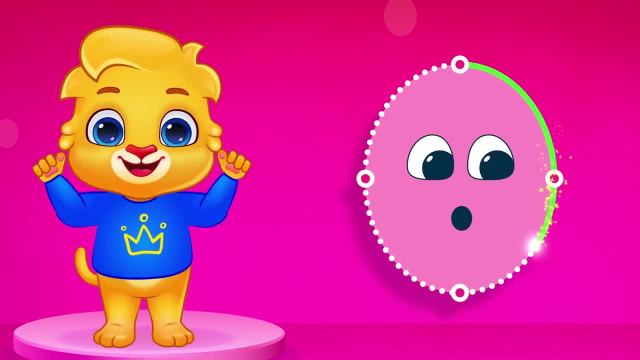 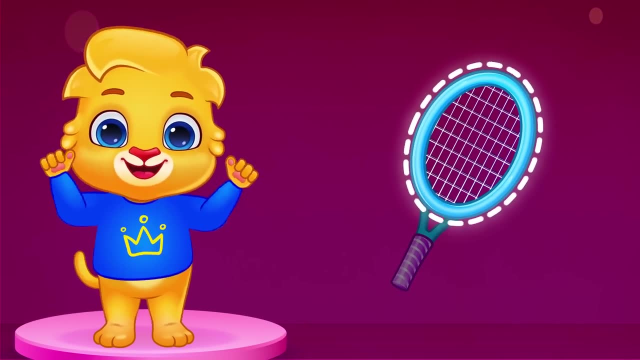 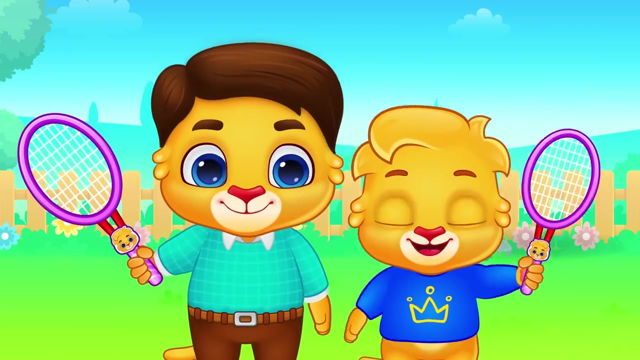 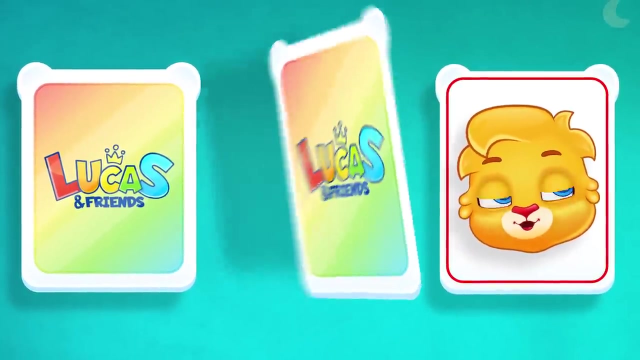 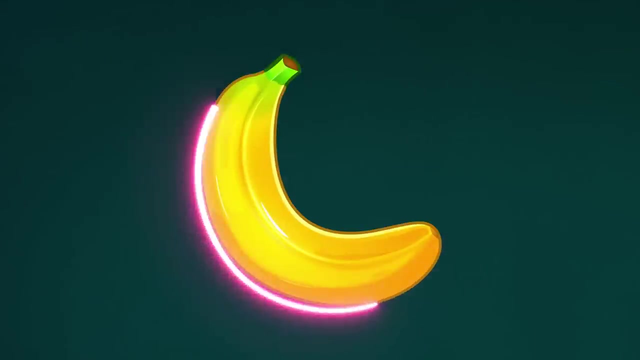 Yahoo, Oval, Wow, Oval oval. The racket looks like an oval. Lucas and his dad are playing with a racket. Woohoo, Eee, Ow, ow, ow, Yes, yes, yes, Banana, Banana Crescent. 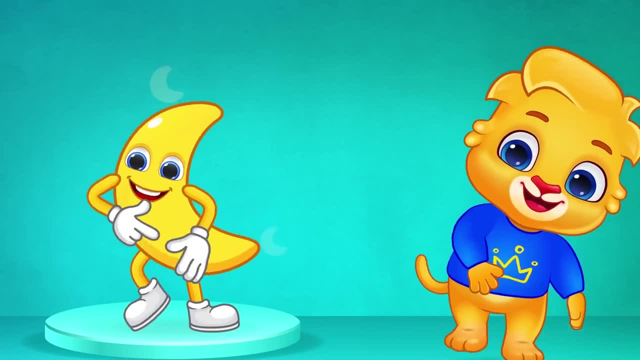 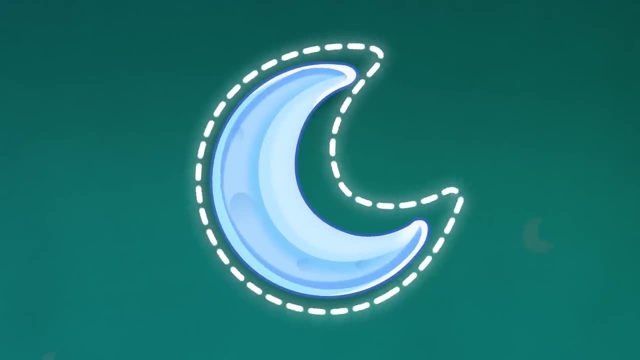 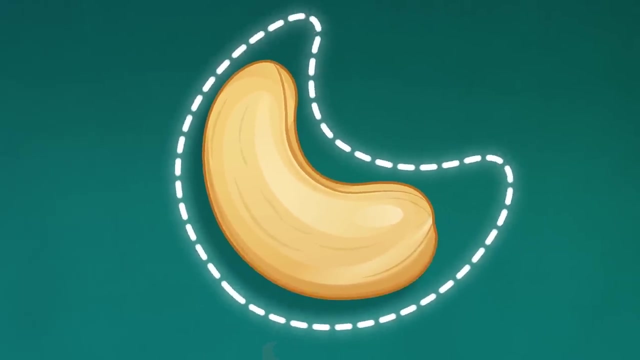 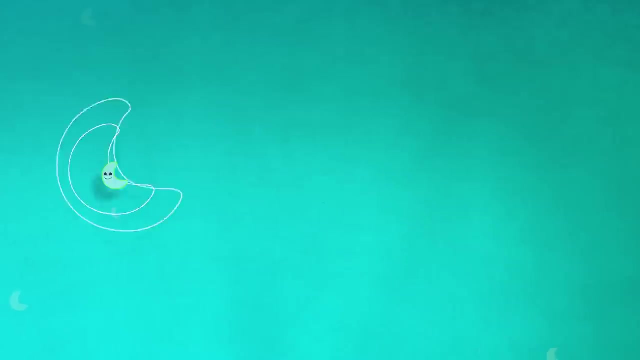 Crescent. Hello, Crescent, This is Crescent Moon Moon. Crescent- Cashew Cashew. Crescent Fringell Fringell. Crescent Crescent. Crescent. Crescent. Crescent Moon Cashew, Fringell. 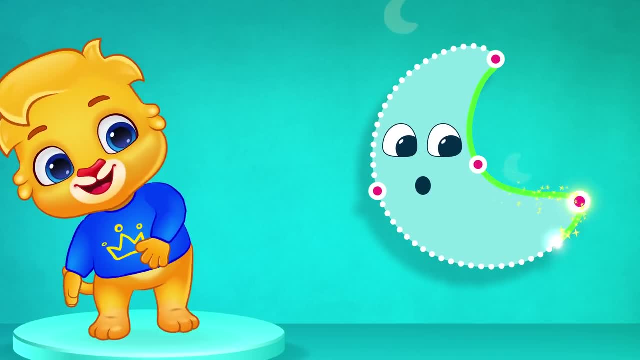 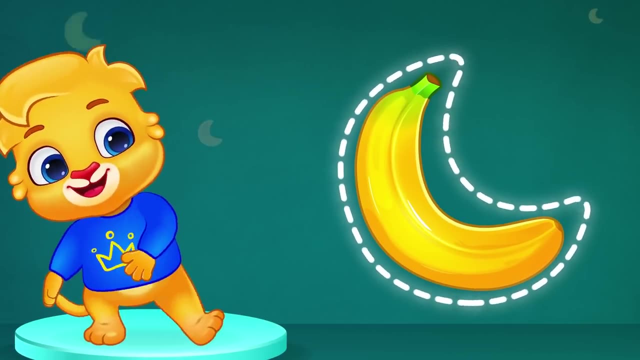 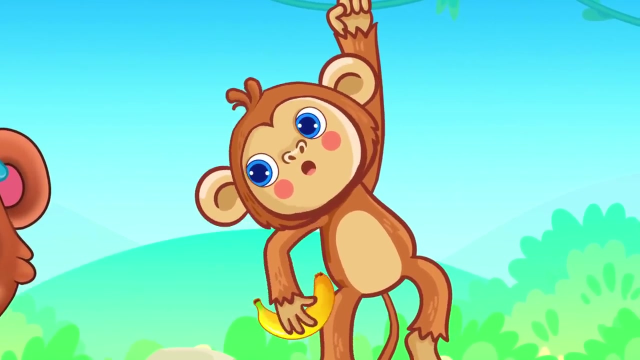 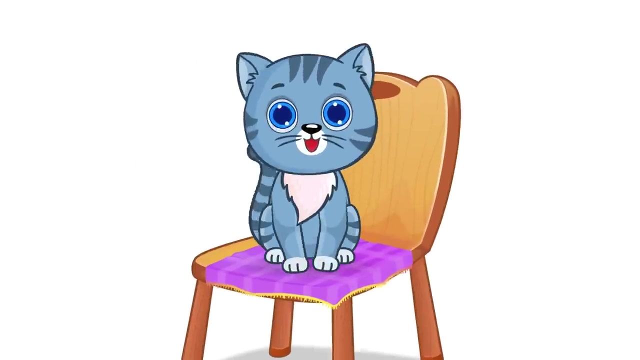 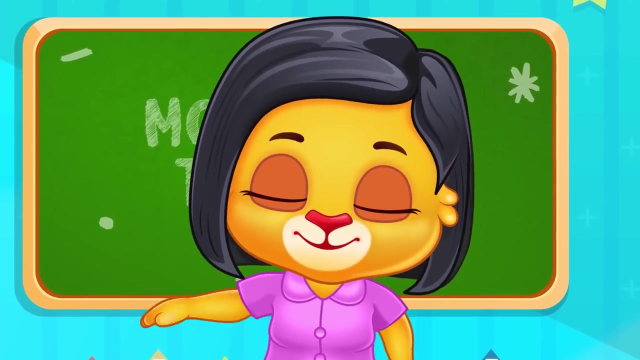 Yes, Crescent Ora, Wow, Crescent Crescent. The shape of the banana is like a crescent. Brody gave a banana to the monkey. Wow, Wow, Wow, Wow, Wow. Very good children, Now it's time to dance. 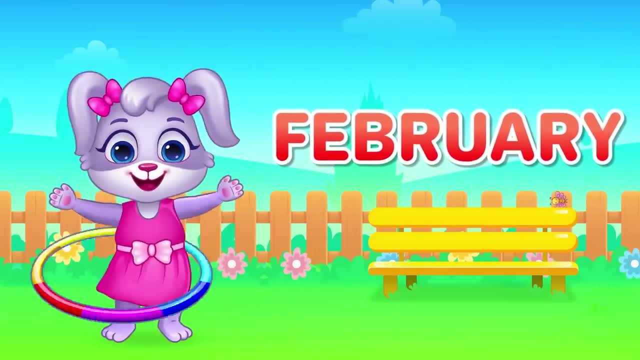 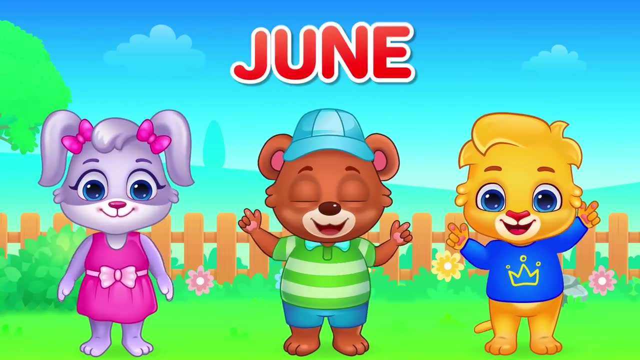 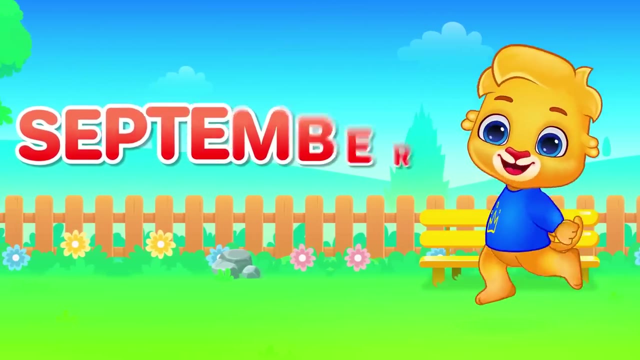 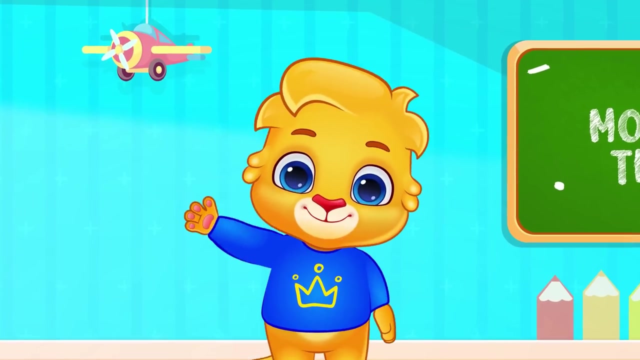 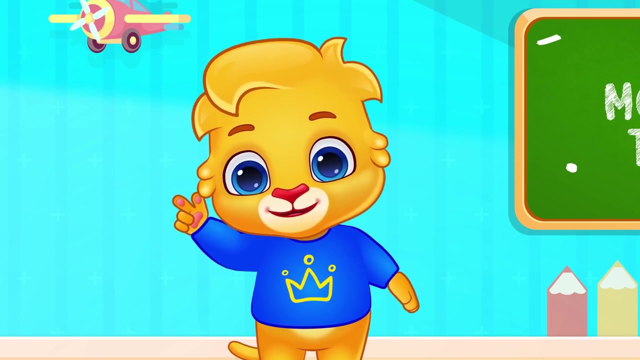 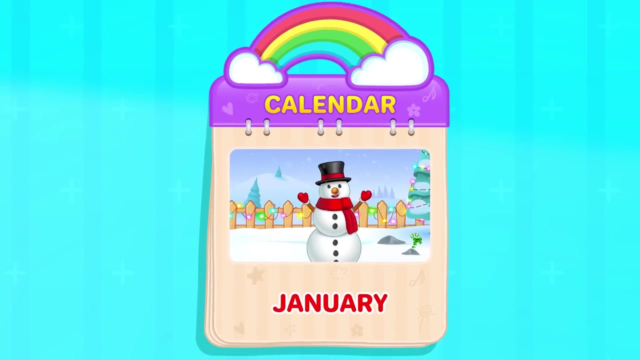 January, February, March, April, May, June, July, August, September, October, November, December. Hi, Let's sing it one more time to make sure we remember it, But this time very slowly. Are you ready? Yeah, January. Well, hello there, boys and girls. 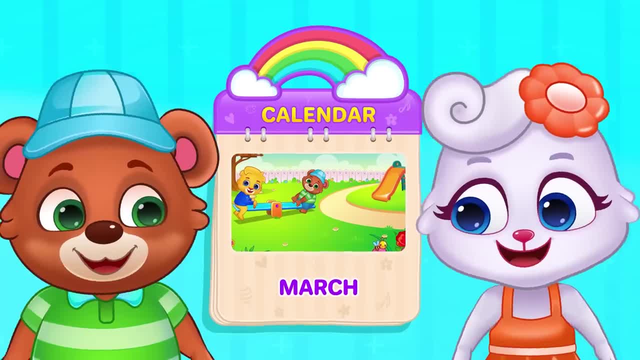 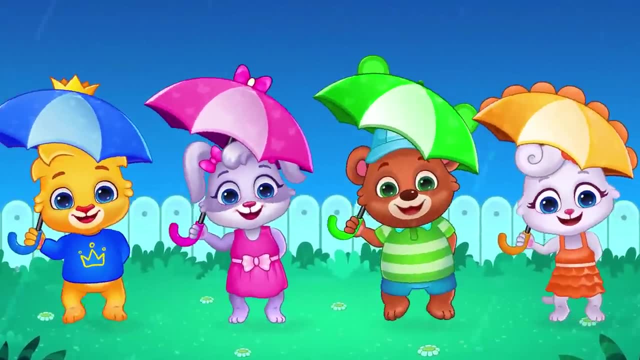 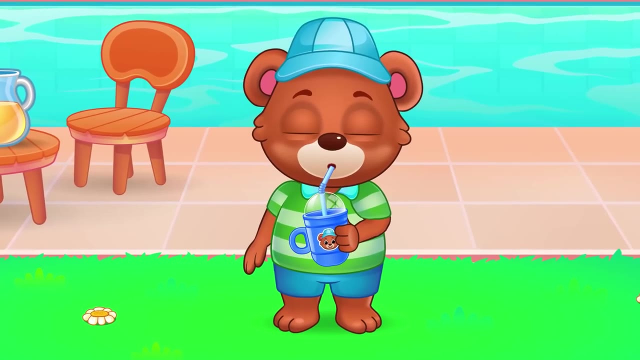 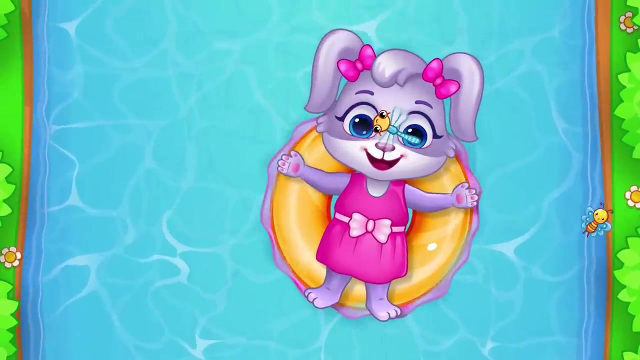 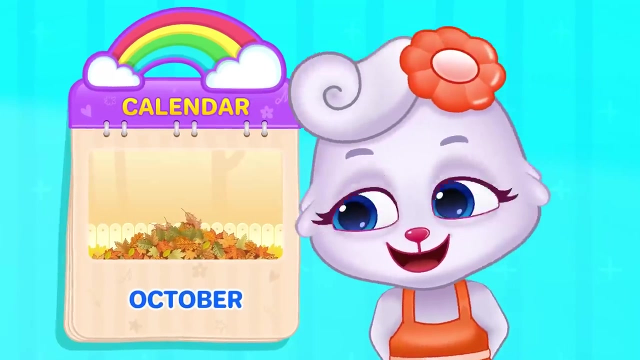 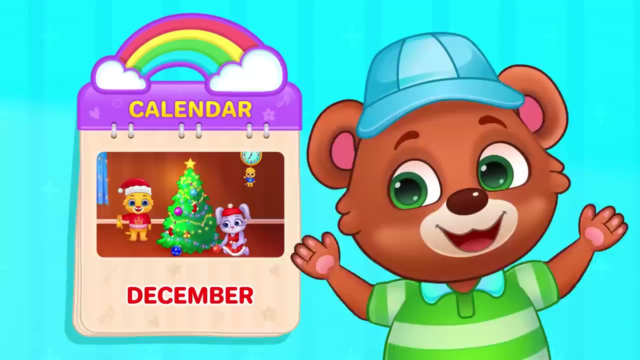 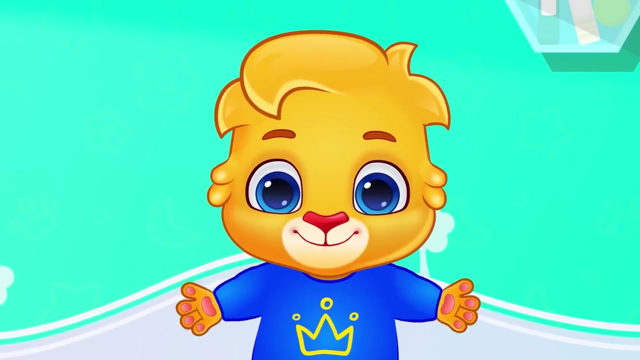 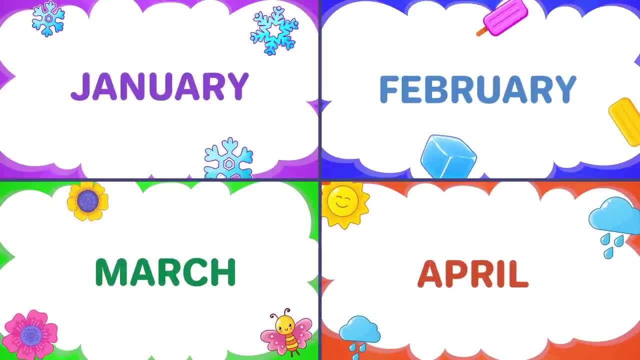 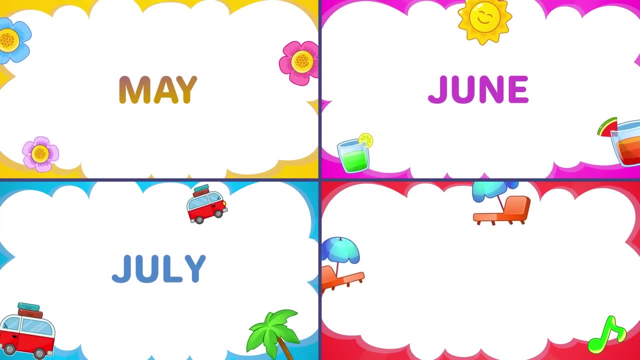 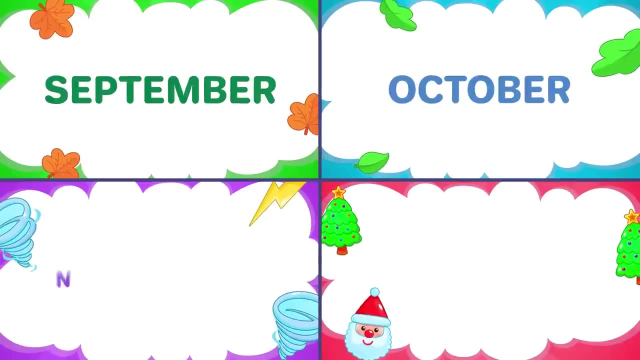 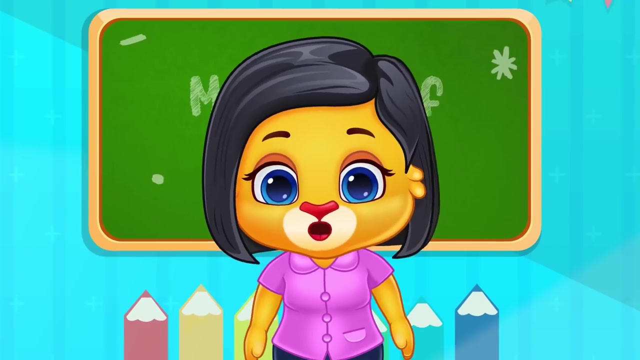 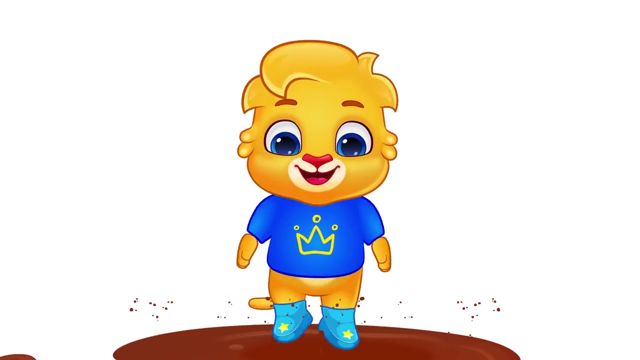 January, February, March, April, January, February, March, April, May, June, July, August, May, June, July, July, August, September, October, November, December, September, October, November, December, September, October, November, December. Woohoo, That was really fun. Very good children. Yeah, This is so much fun. 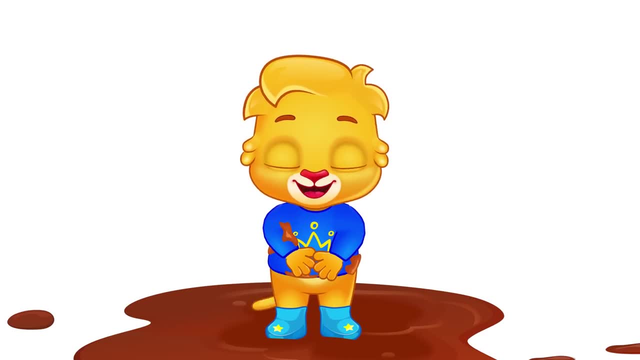 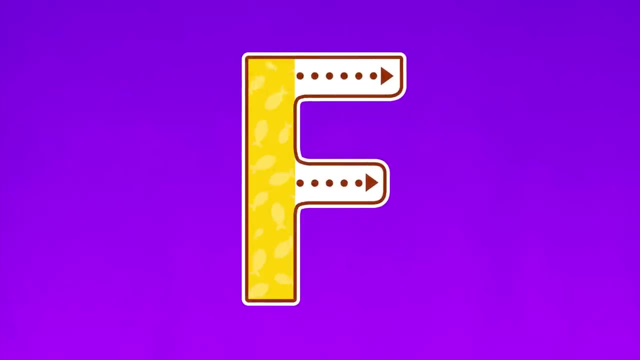 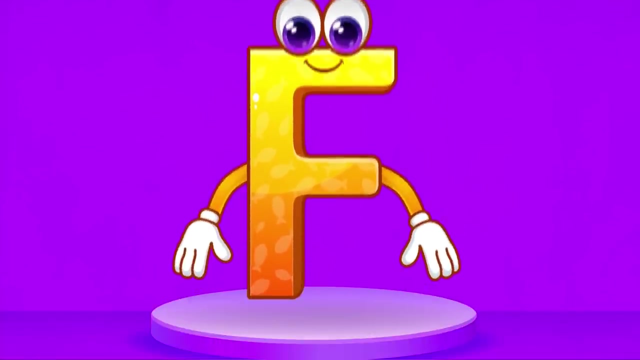 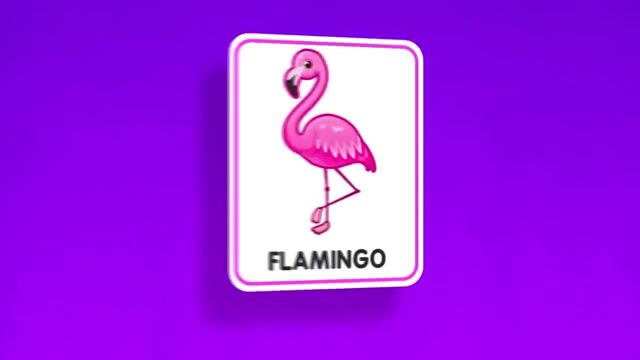 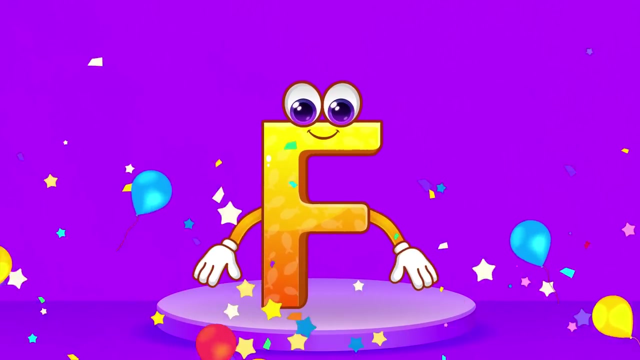 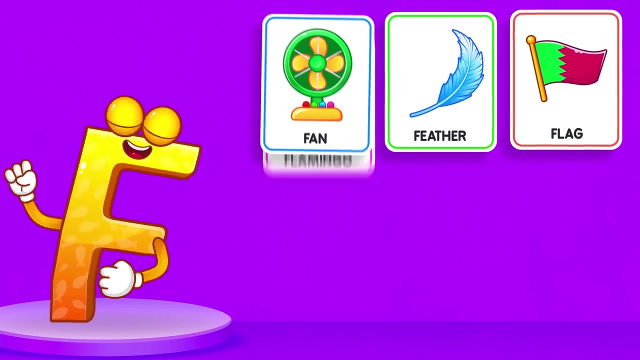 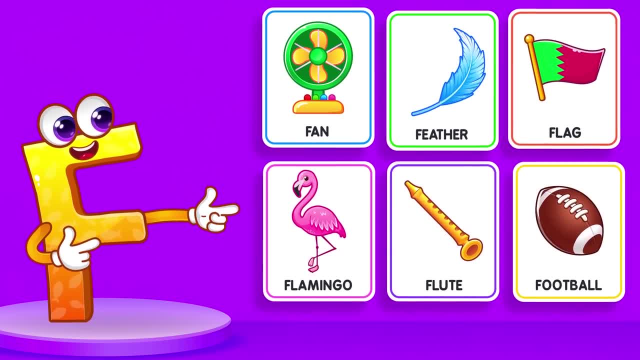 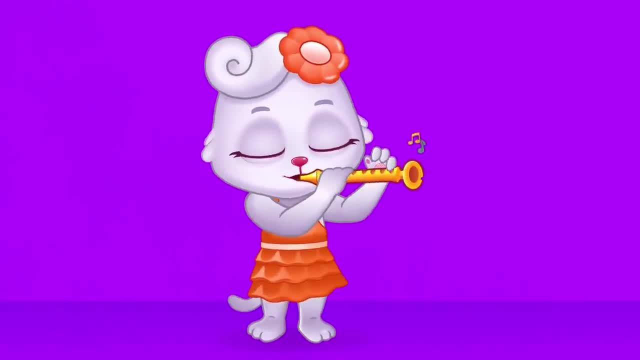 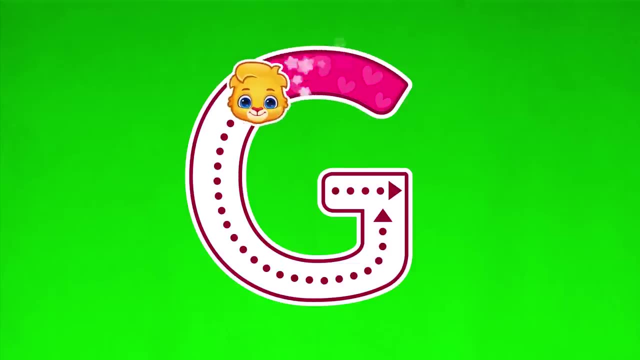 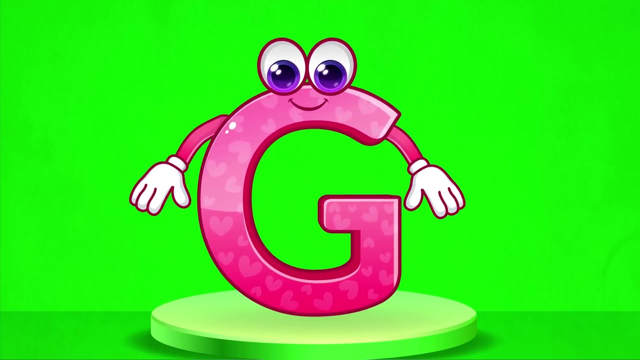 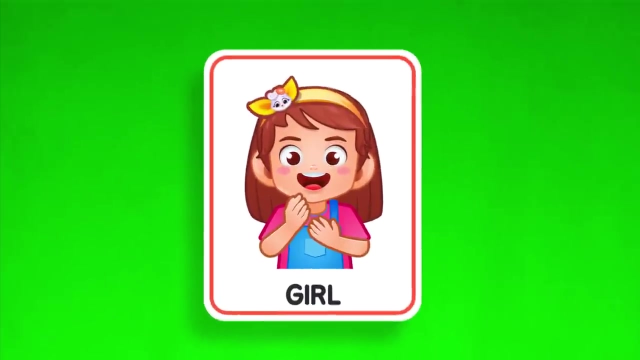 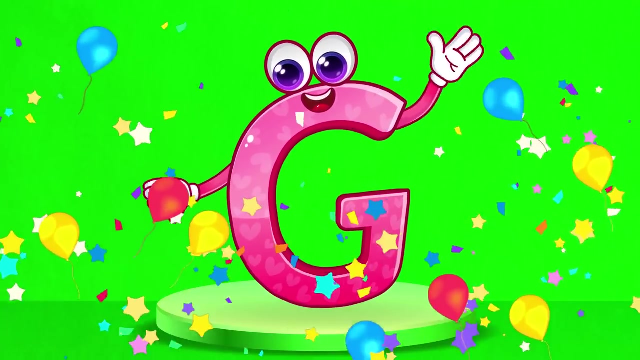 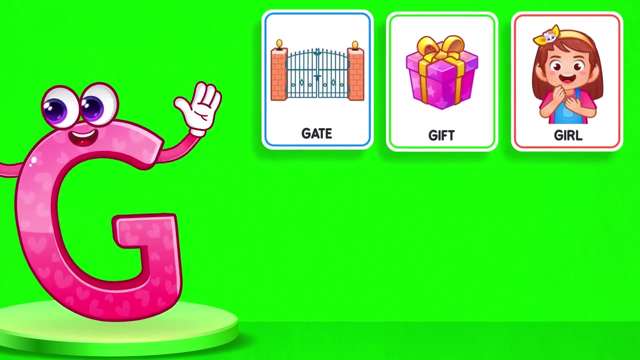 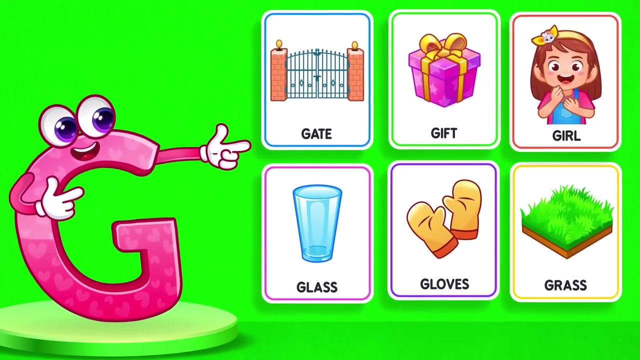 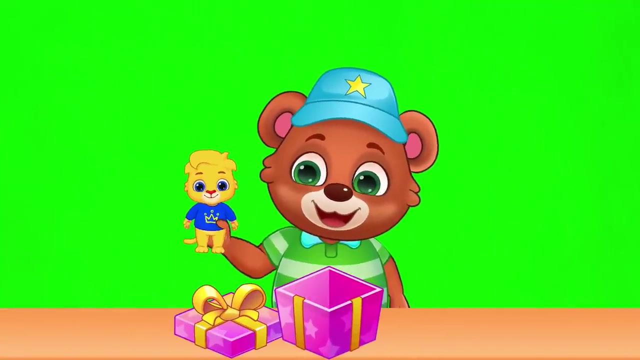 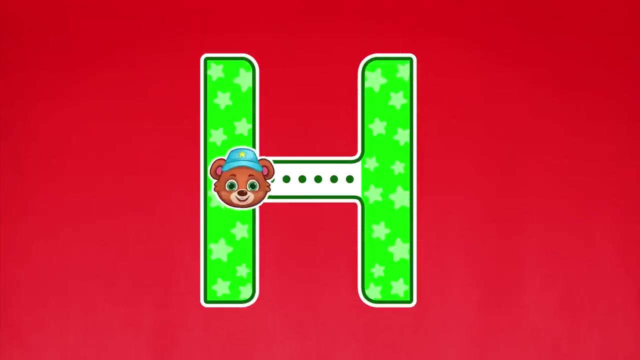 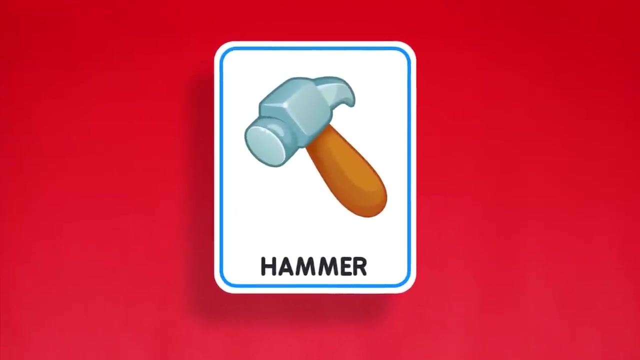 flute football. Aha, G. This is G. Hi, G is for gate gift girl, glass gloves grass. This is G. G is for gate gift girl, glass gloves grass. Aha, Ayo H. This is H. Hi, H is for hammer. 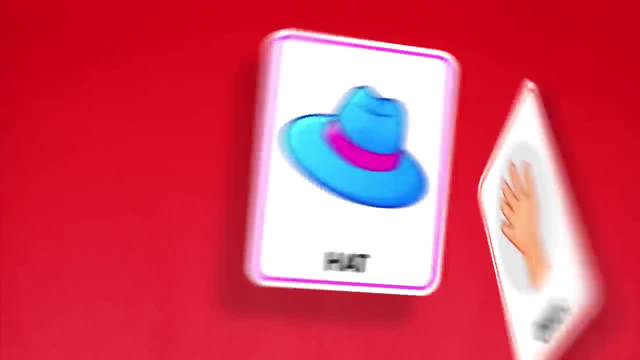 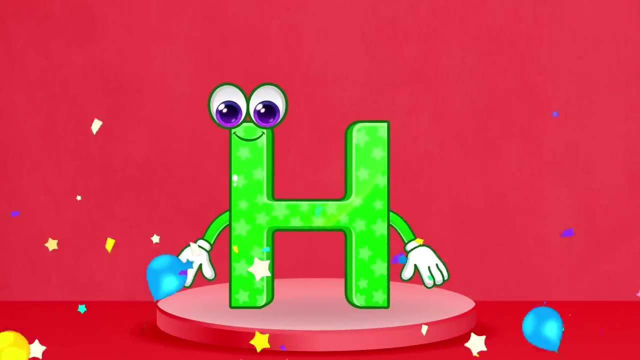 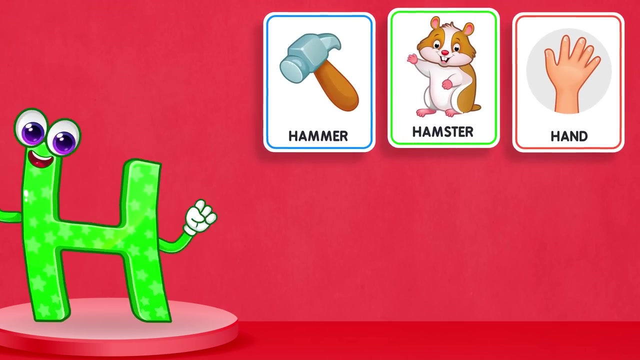 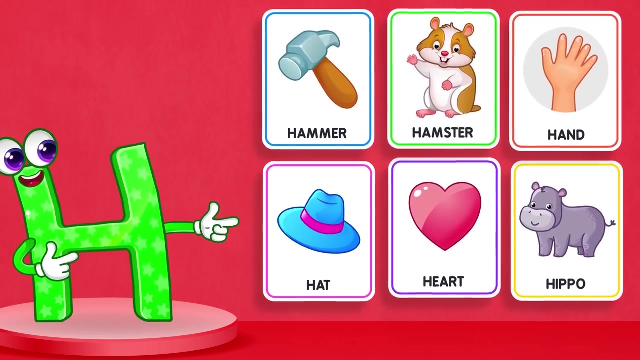 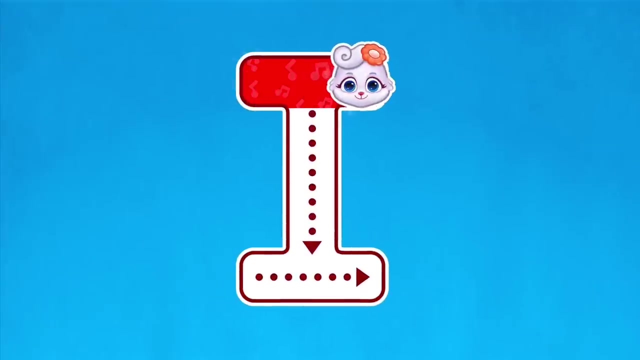 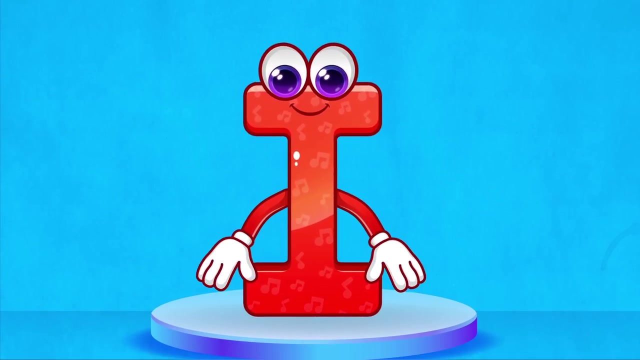 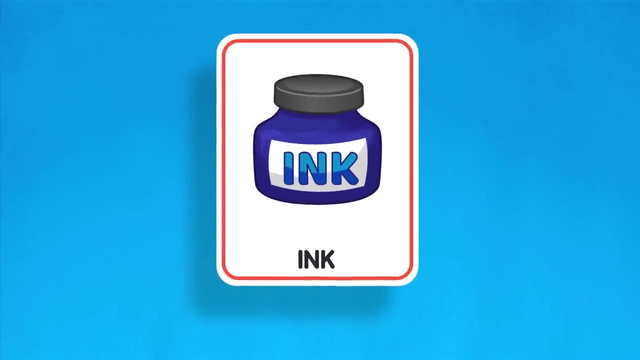 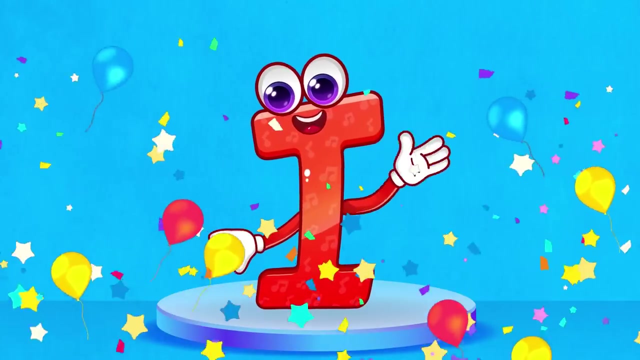 hamster hand hat heart hippo. This is H. H is for hammer. hamster hand hat heart hippo. I- This is I. Hi, I is for ice cream igloo. ink insect instrument island. This is I. I is for ice cream igloo. 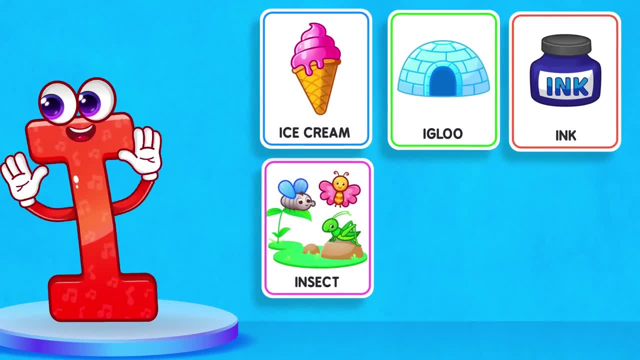 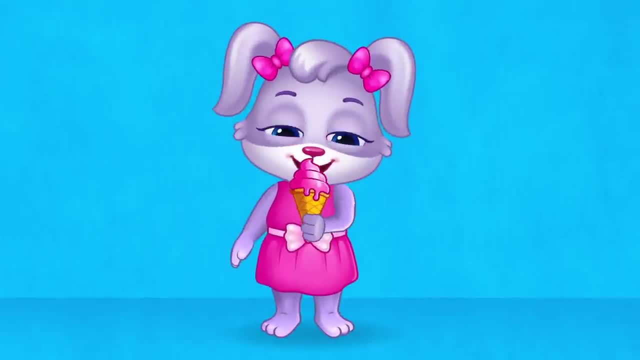 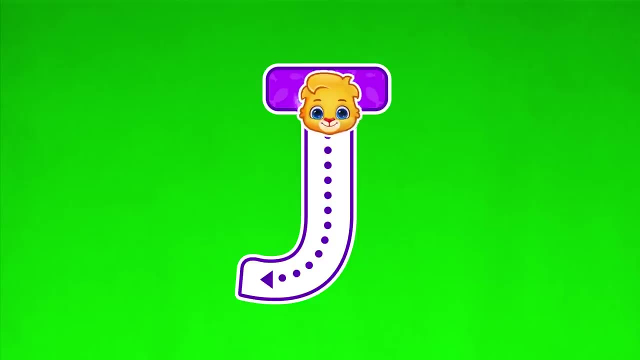 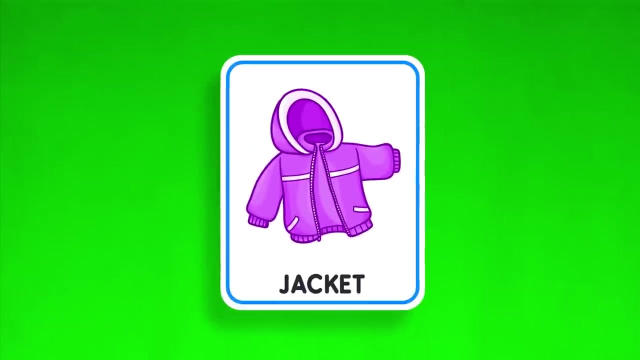 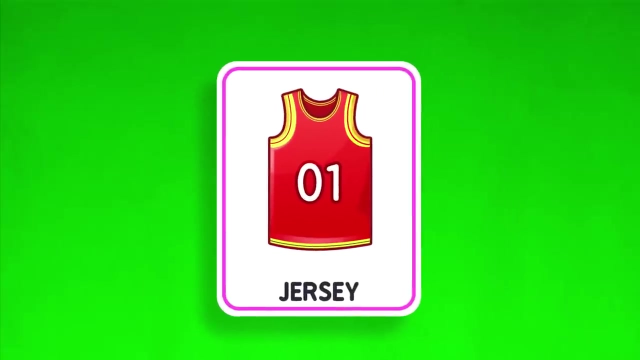 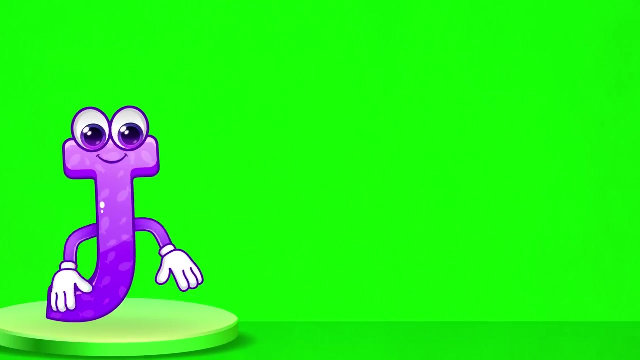 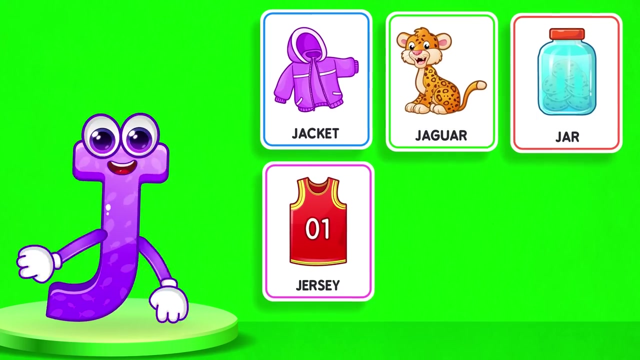 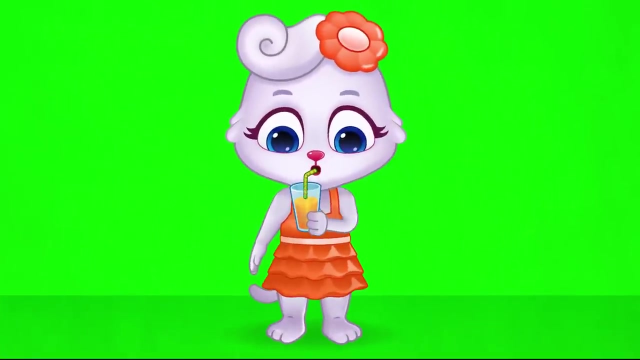 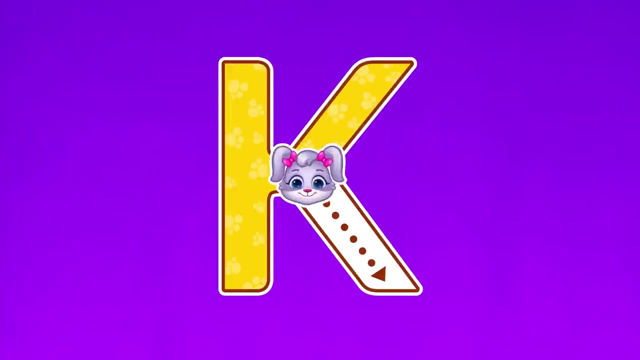 ink insect instrument island. J. This is J. This is J. Hi, J is for jacket jacket jaguar jar jersey jet juice. This is J. J is for jacket jaguar jar jersey jet juice. Aha, K, This is K, This is K. 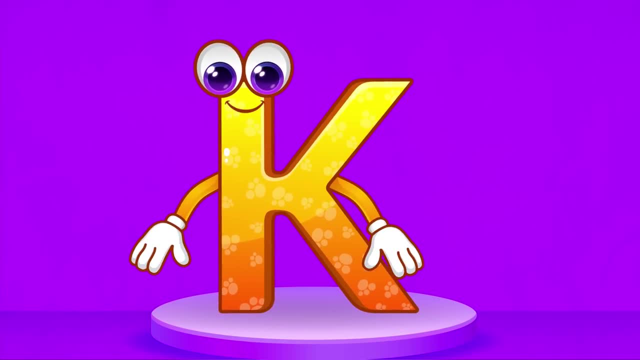 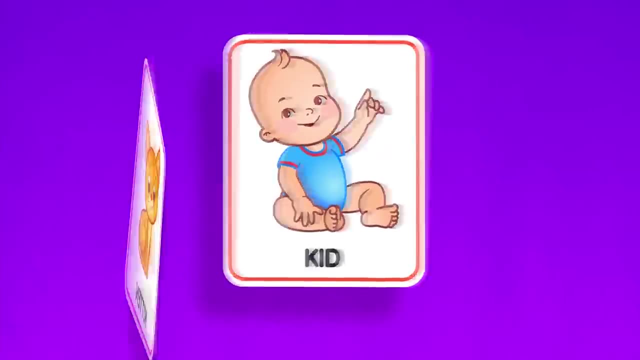 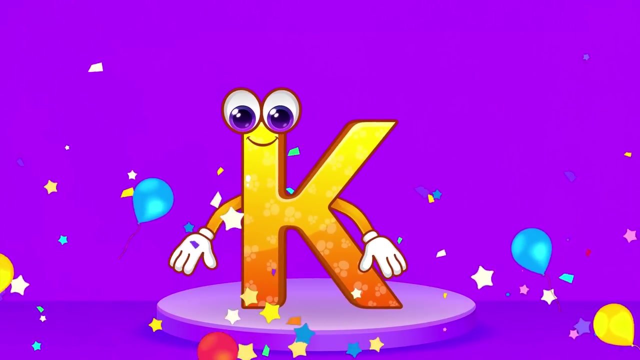 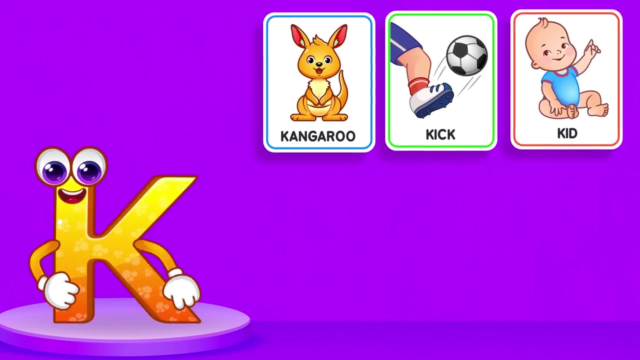 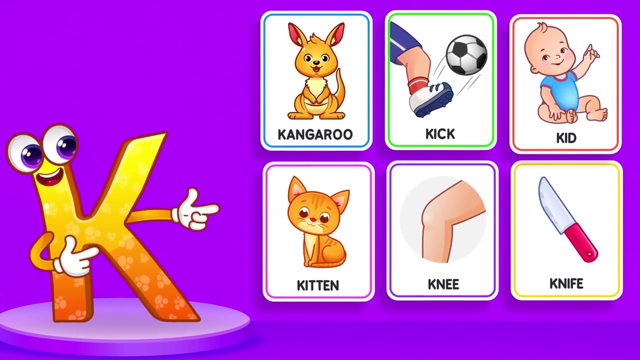 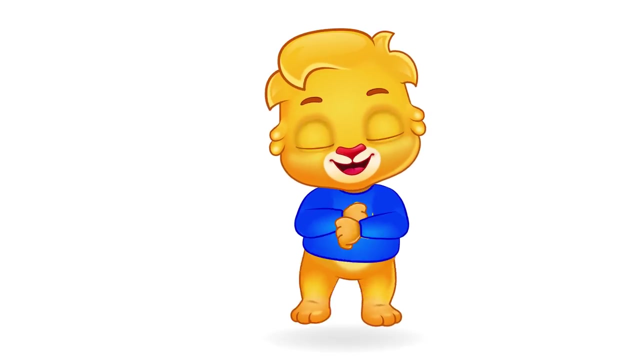 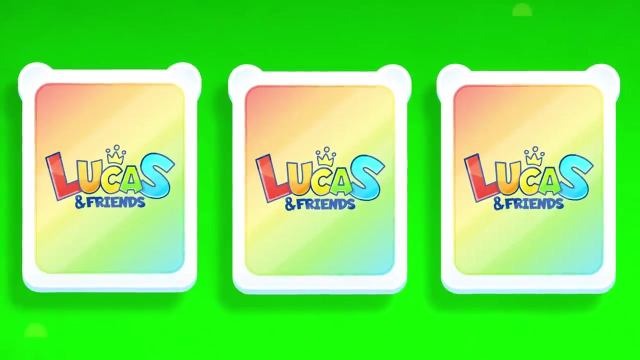 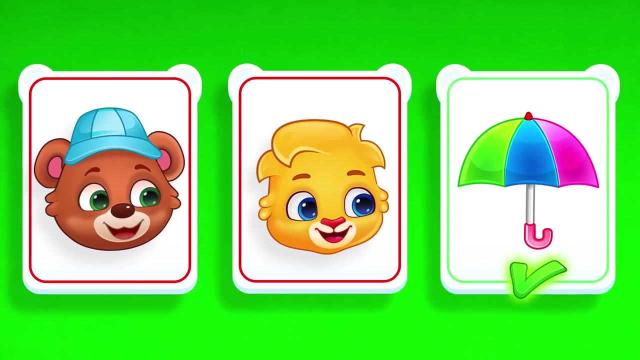 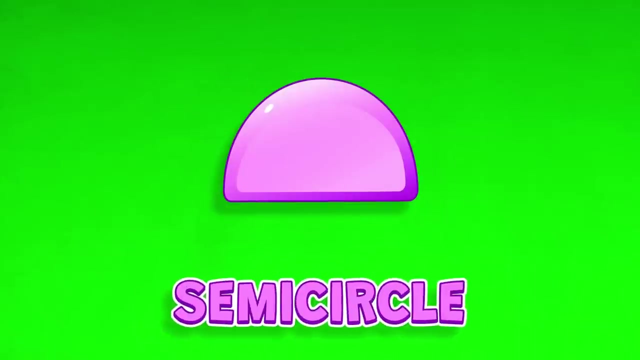 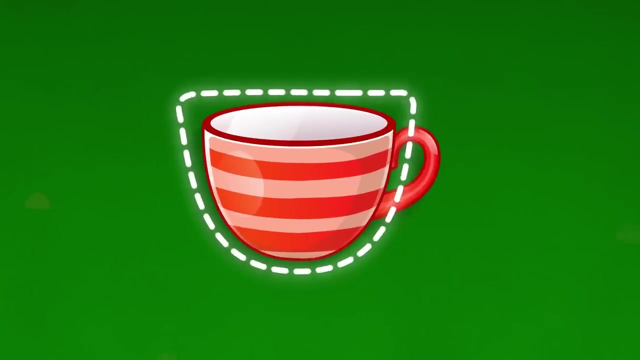 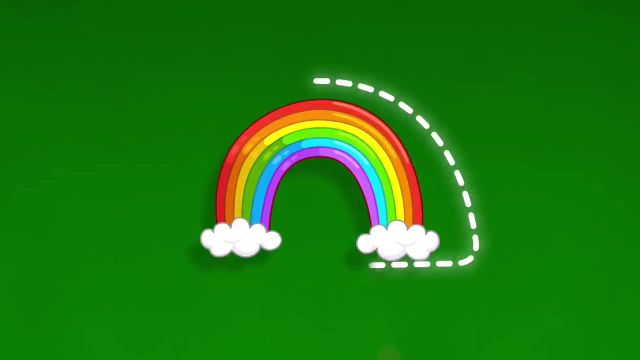 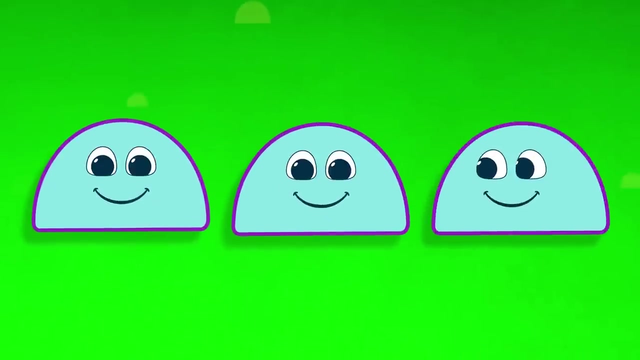 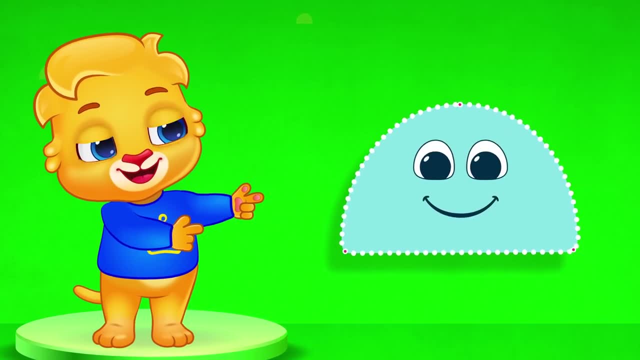 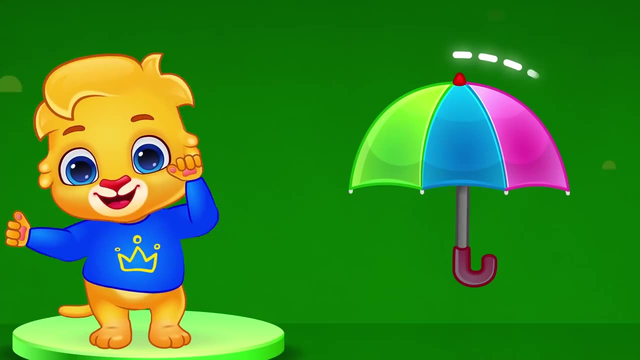 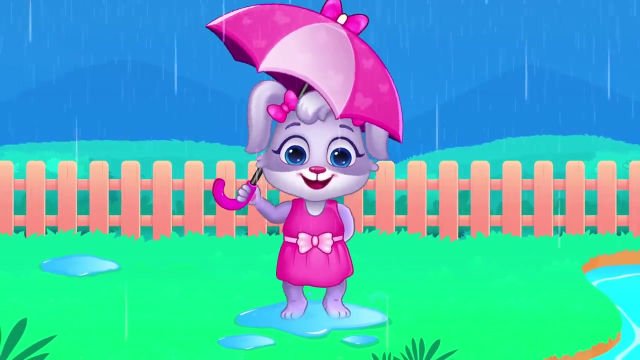 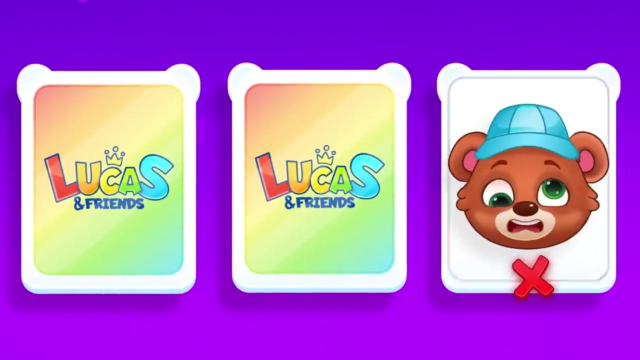 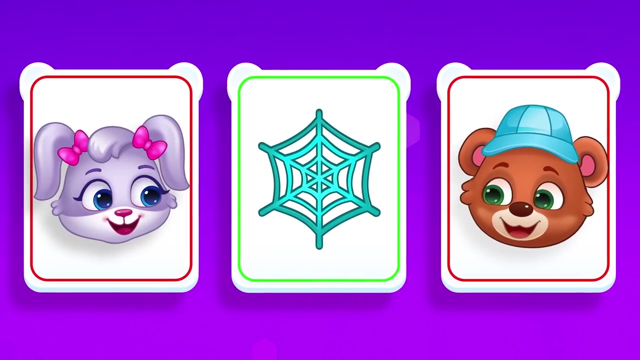 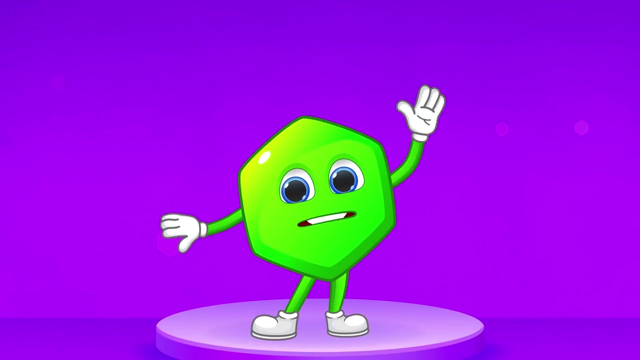 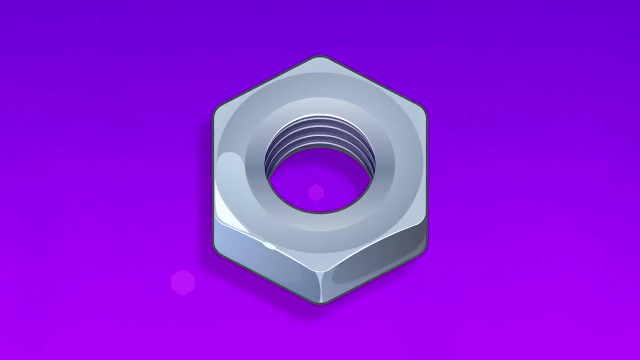 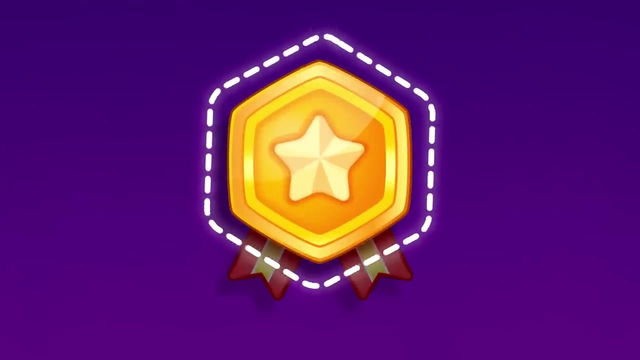 Igloo rainbow: semicircle, semicircle, semicircle. umbrella looks like a semicircle. Ruby is dancing with an umbrella, Web, web, hexagon, hexagon, hexagon. This is hexagon, Nut, nut, hexagon, metal, metal, hexagon. 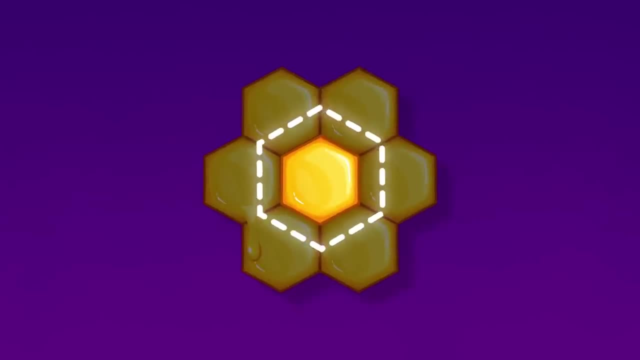 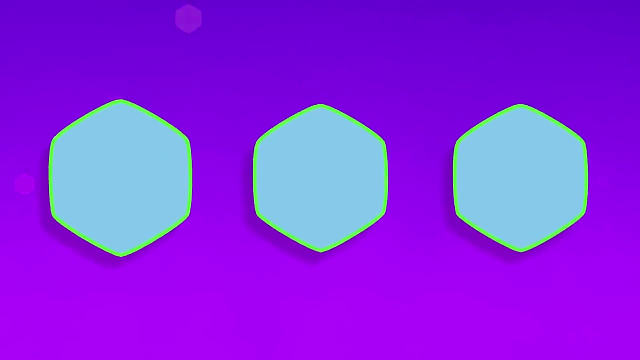 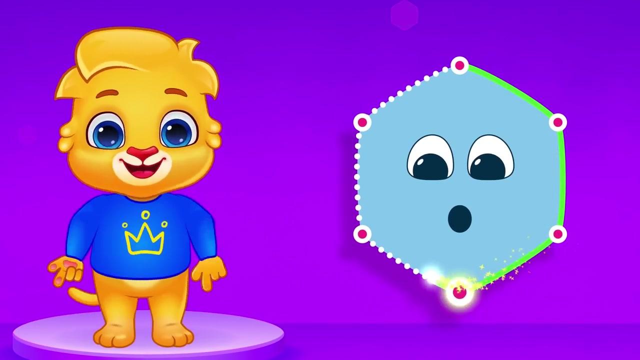 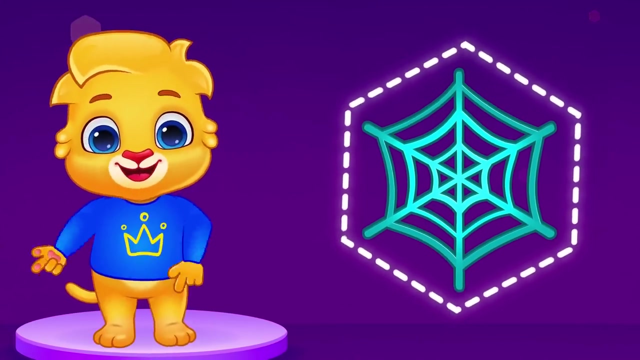 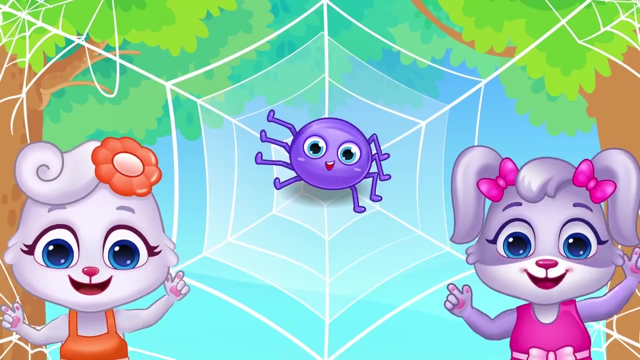 Honeycomb, honeycomb, hexagon, hexagon, hexagon, hexagon. Nut metal honeycomb, hexagon, Wow, Hexagon, hexagon, hexagon, Wow A web. looks like a hexagon Spider is dancing on its web. 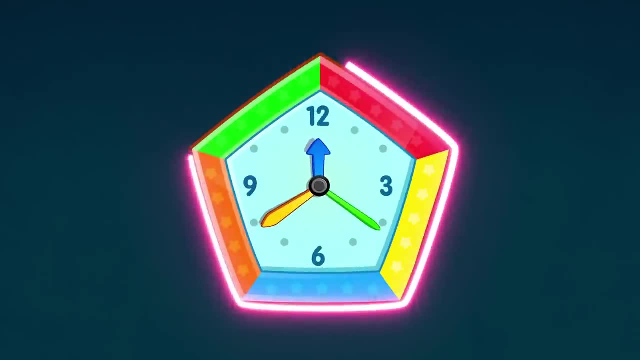 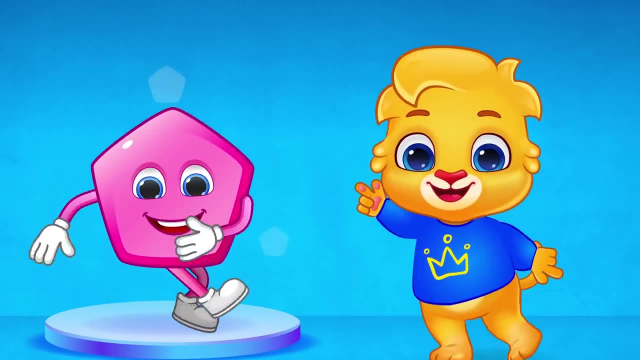 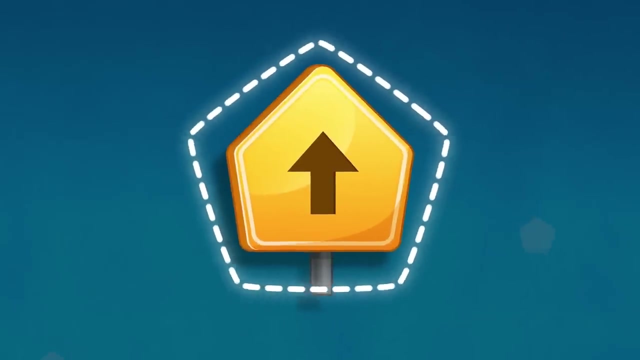 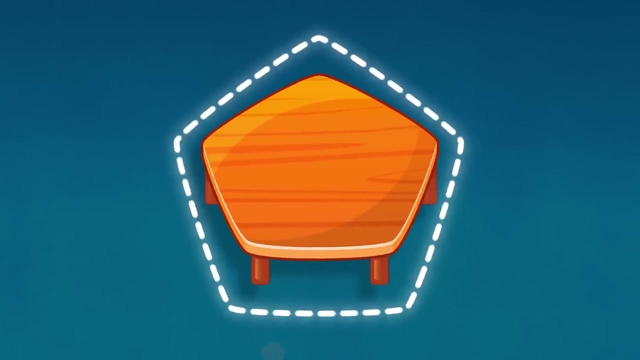 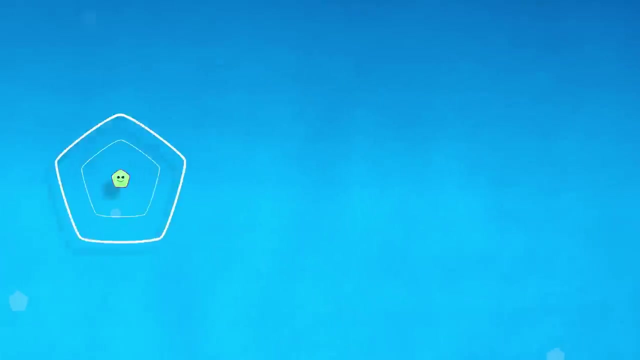 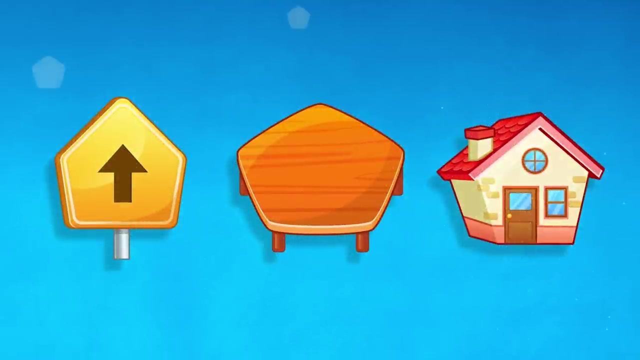 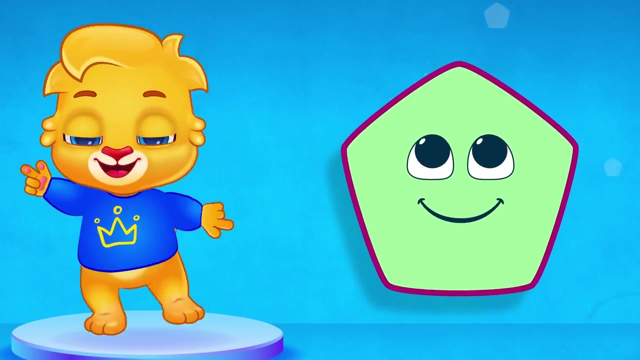 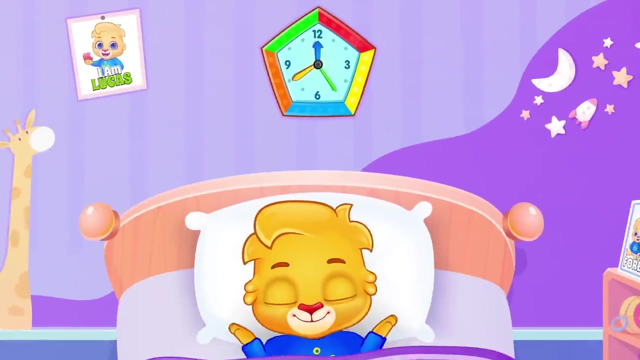 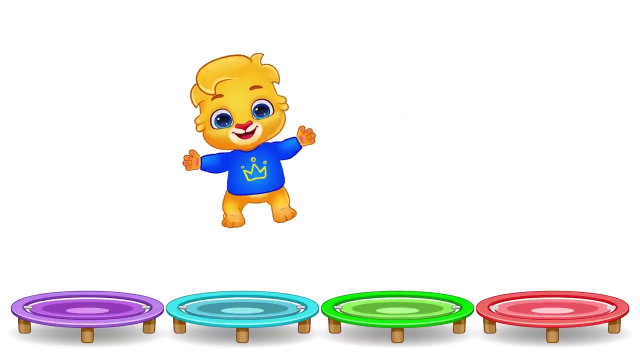 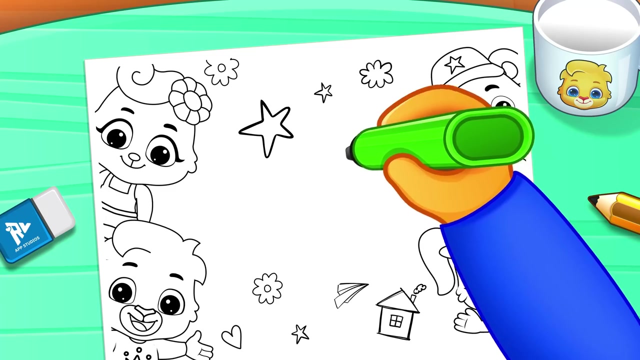 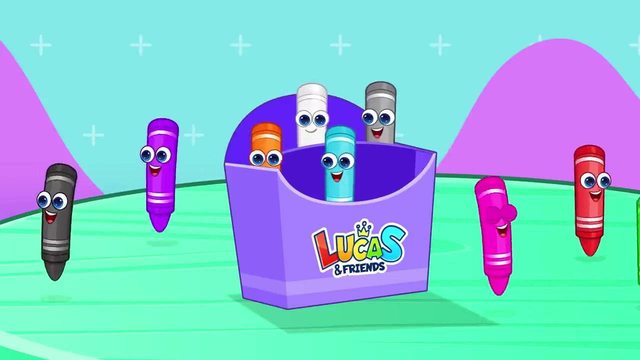 Clock Pentagon. This is Pentagon Signboard Table, Pentagon House. Pentagon Signboard Table House, Pentagon, Pentagon. The shape of this clock is like a pentagon. Lucas has a beautiful clock. The size of this clock is like a pentagon. The size of this clock is like a pentagon. 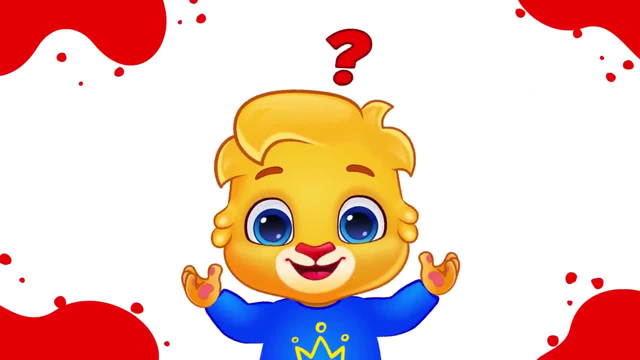 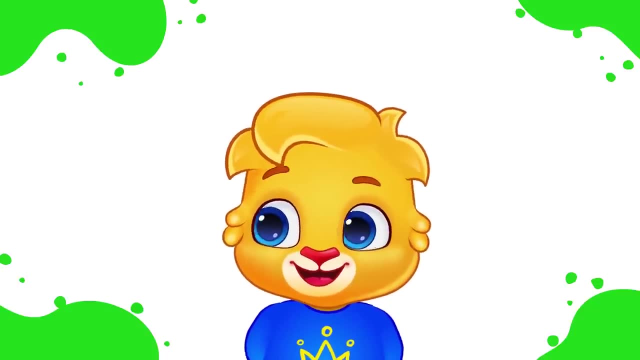 Red color: red color: where are you Here? I am, here, I am. how do you do? Green color: green color: where are you Here? I am here, I am. how do you do? Here I am, how do you do. 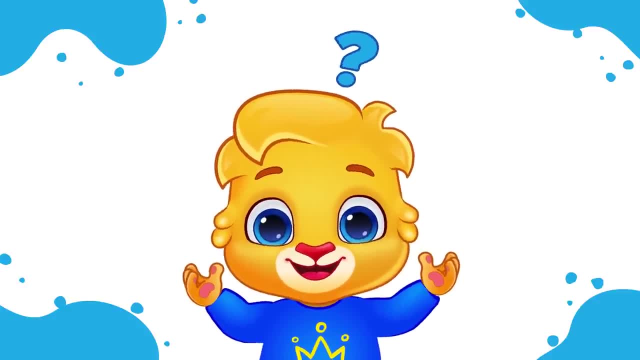 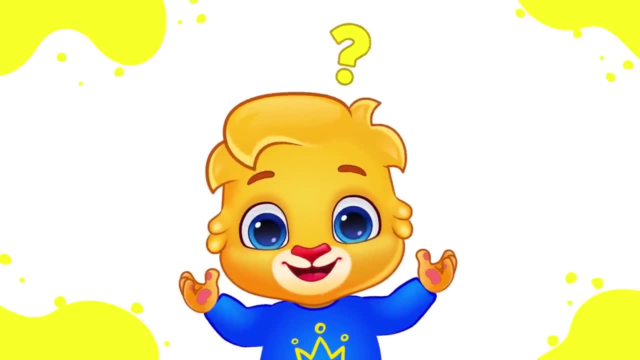 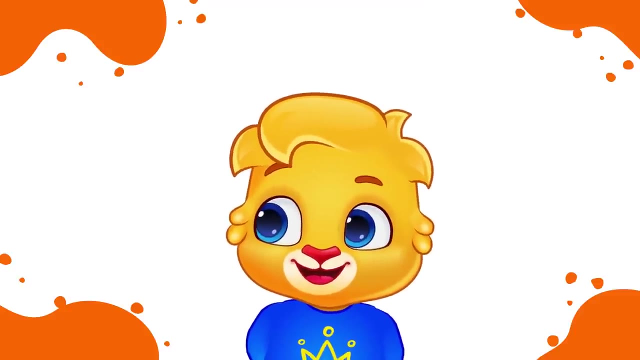 Blue color, blue color- where are you Here? I am here, I am. how do you do Yellow color, yellow color- where are you Here? I am here, I am. how do you do Orange color, orange color- where are you? 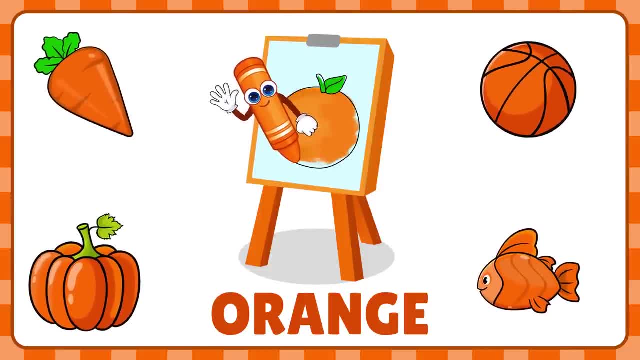 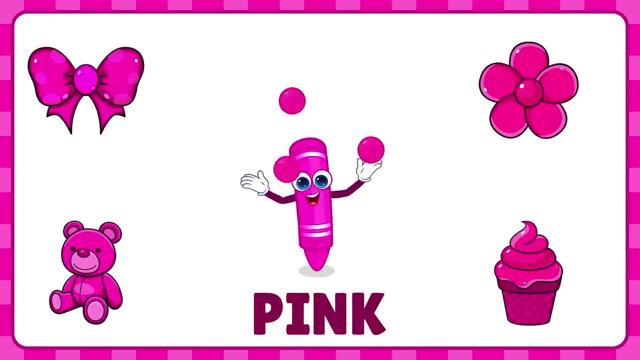 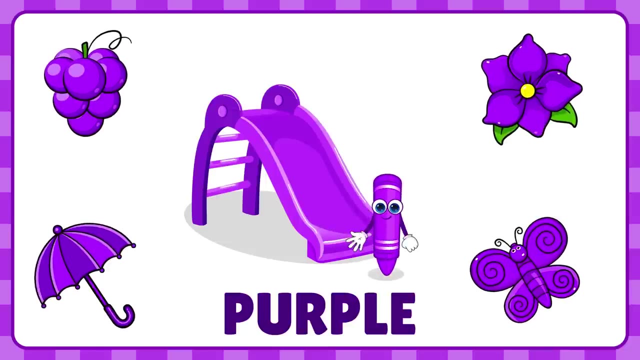 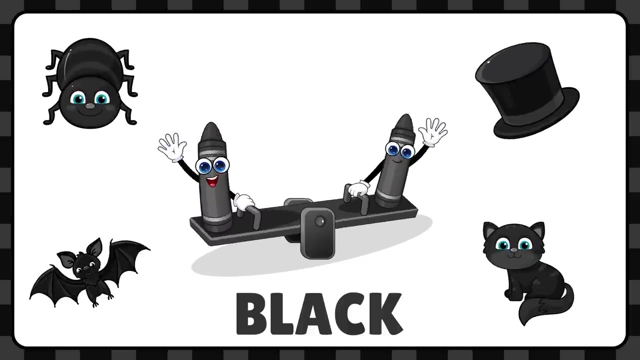 Here I am, here I am. how do you do pink color, pink color- where are you here? i am, here, i am. how do you do purple color, purple color- where are you here? i am here i am. how do you do black color, black color- where are you here? i am here, i. 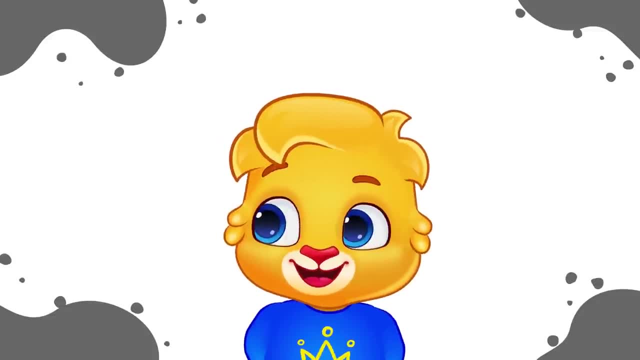 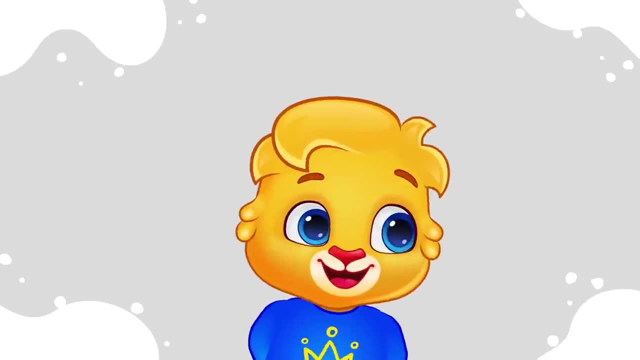 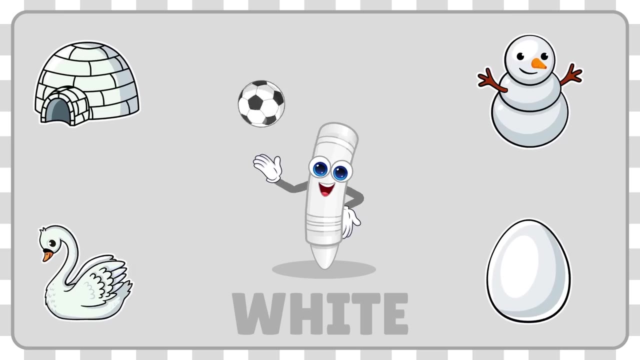 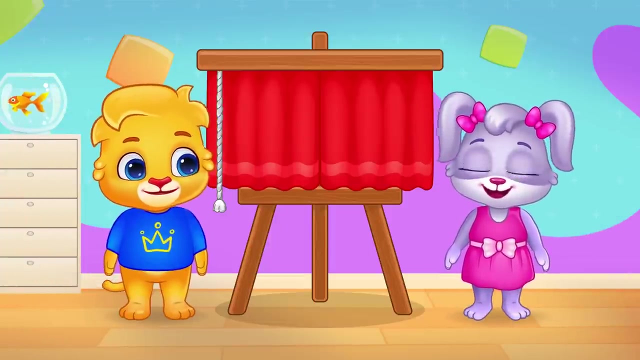 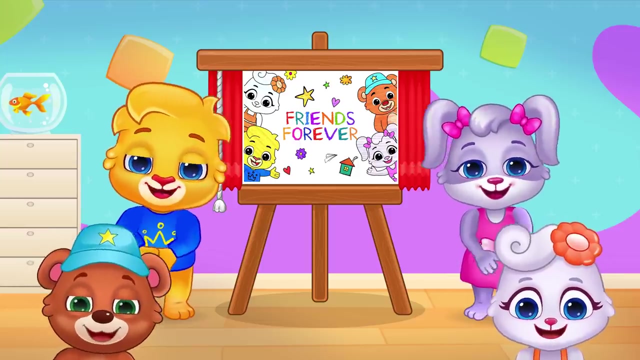 How do you do Gray color? gray color- Where are you Here? I am here, I am. How do you do White color? white color- Where are you Here? I am here, I am. How do you do? Yeah, Woo-hoo. 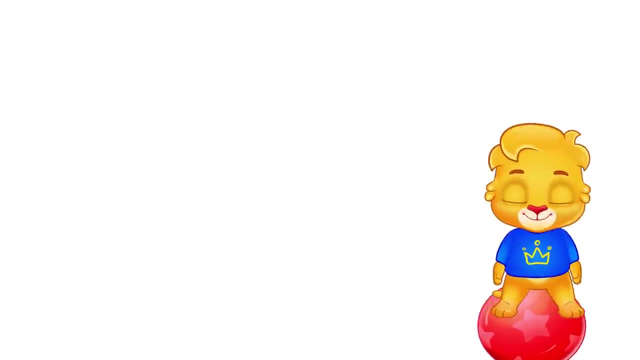 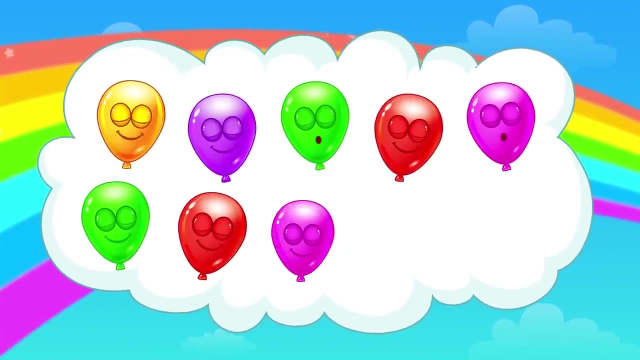 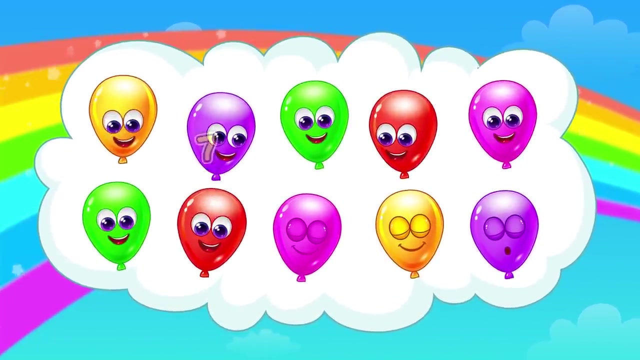 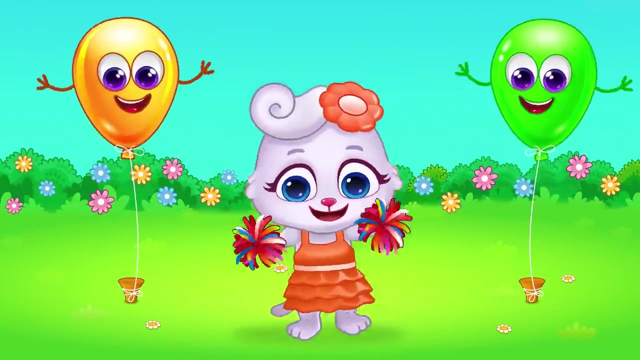 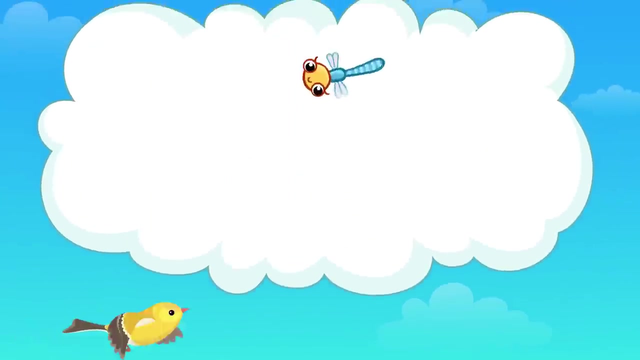 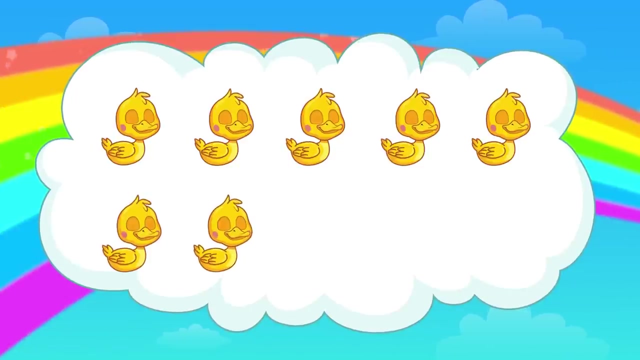 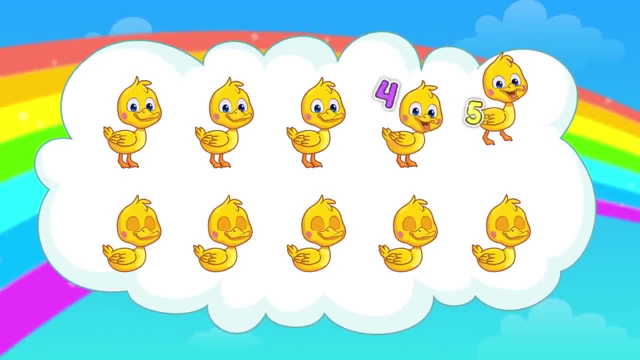 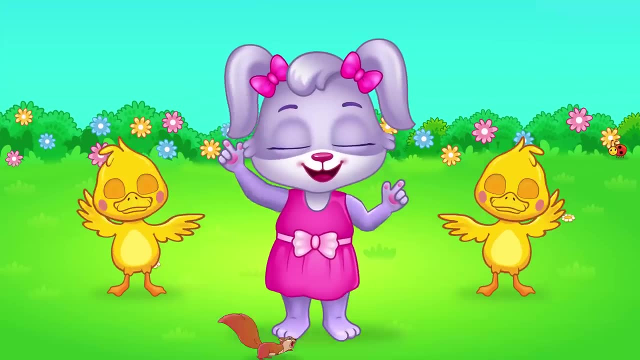 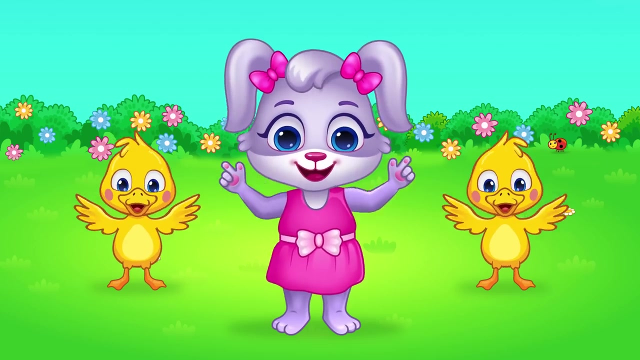 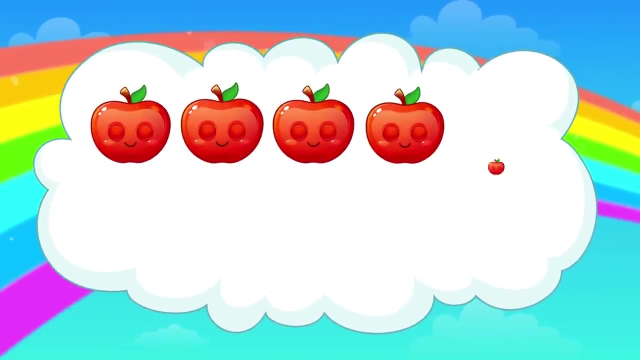 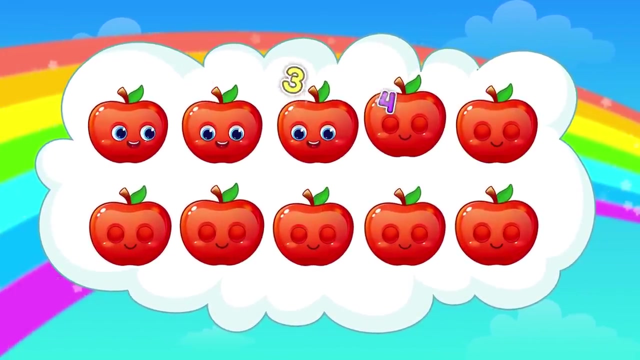 One, two, three, four, five, six, seven, eight, nine, ten, Woo-hoo Woo-hoo. One, two, three, four, five, six, seven, eight, nine ten. One, two, three, four, five, six, seven, eight, nine ten. 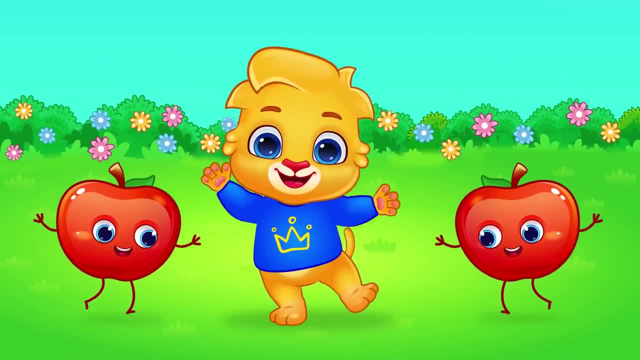 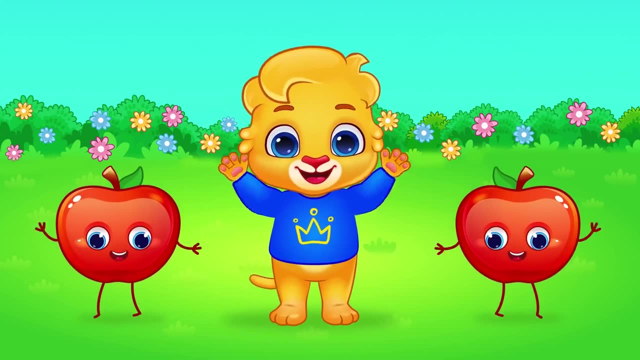 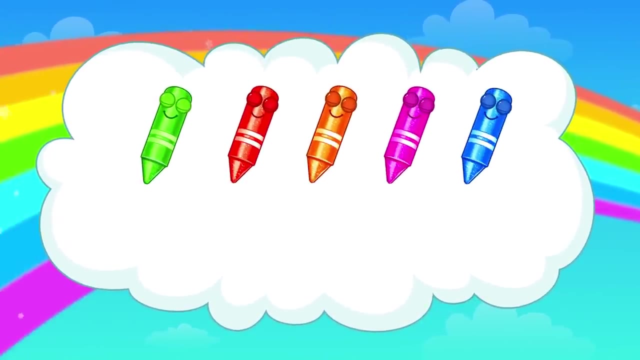 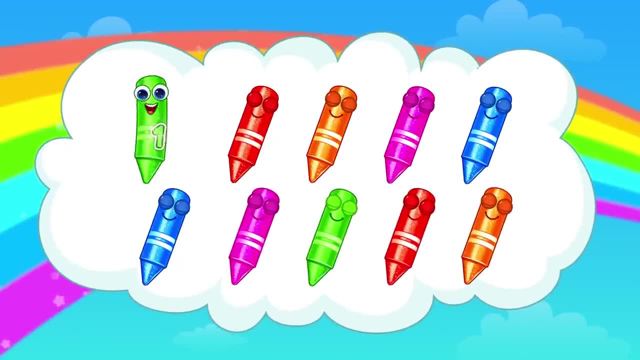 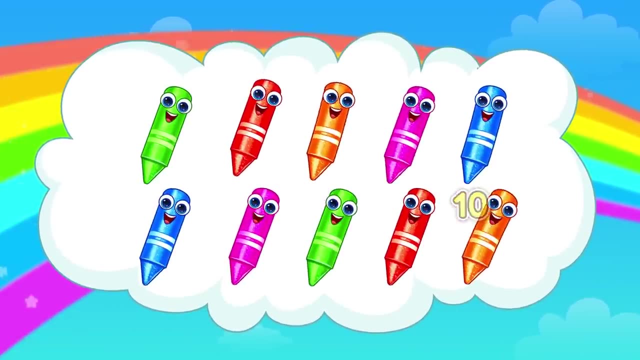 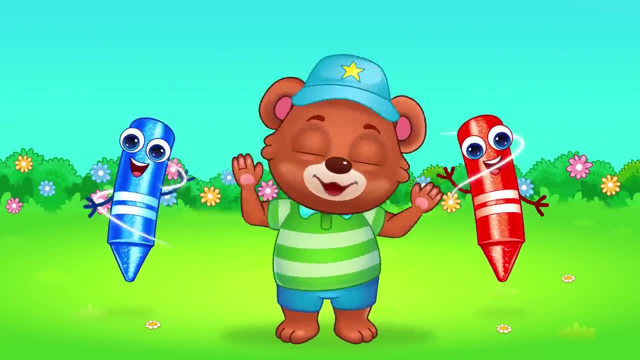 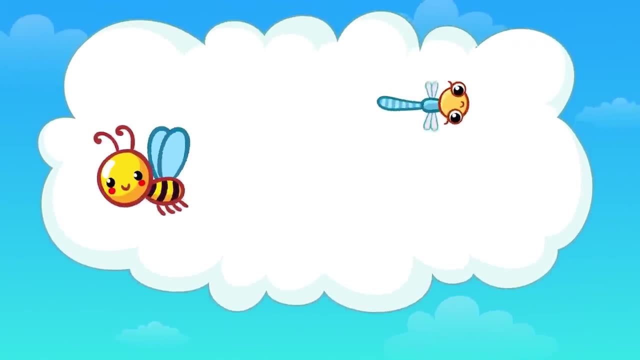 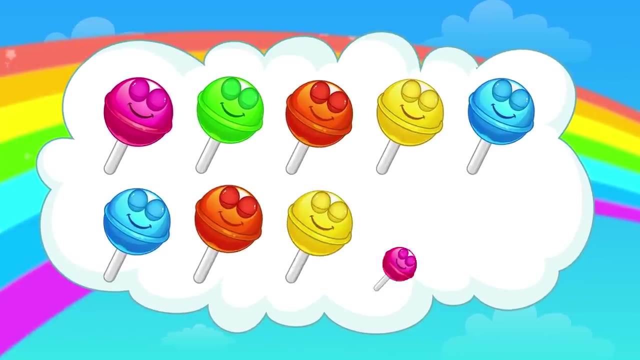 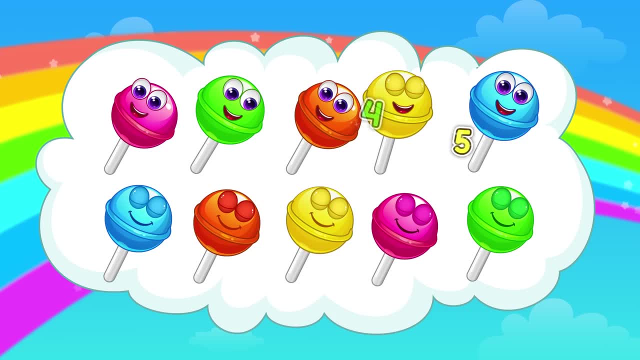 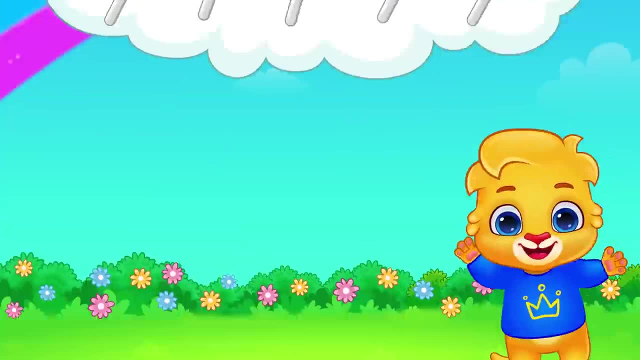 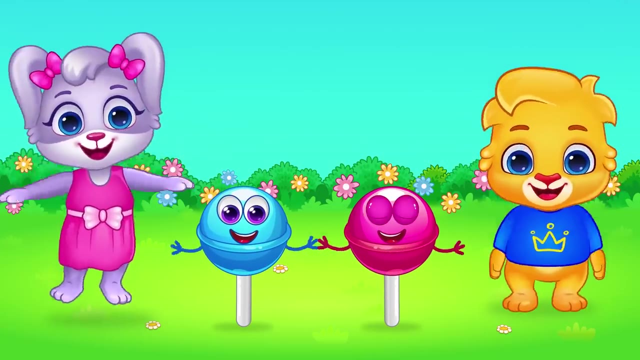 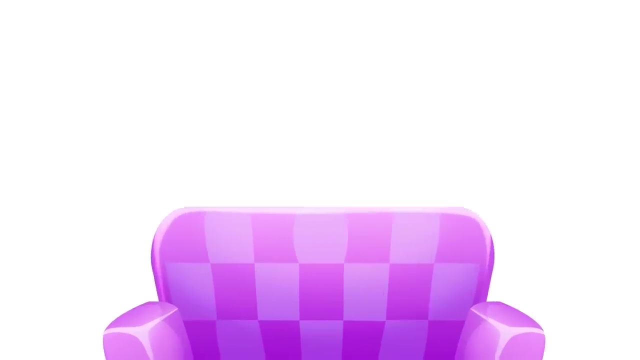 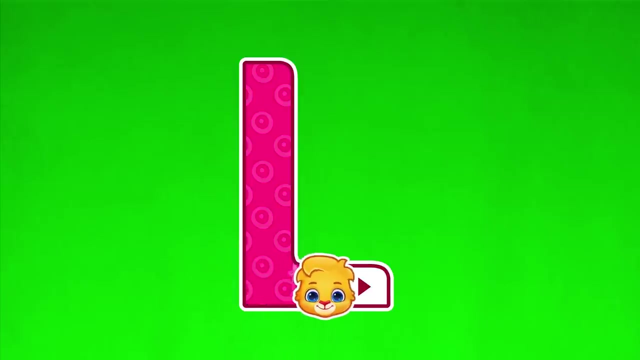 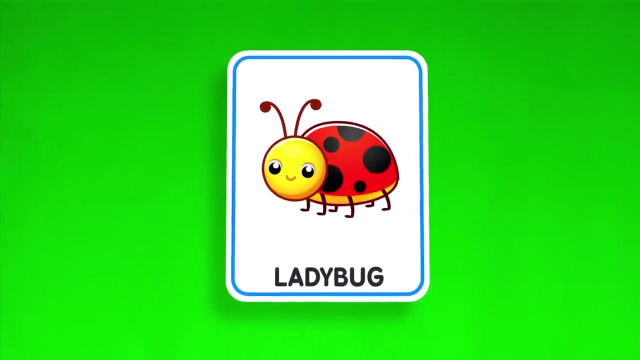 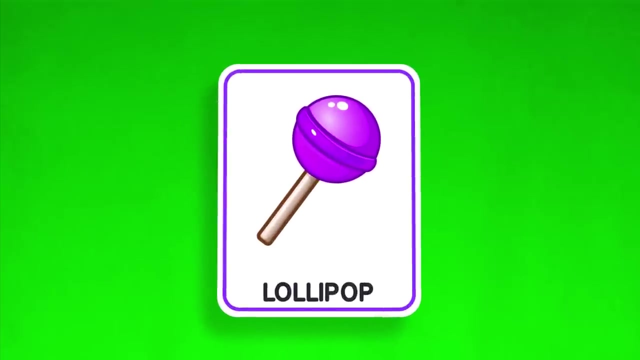 1,, 2,, 3,, 4,, 5,, 6,, 7,, 8,, 9, 10. 1,, 2,, 3,, 4,, 5,, 6,, 7,, 8,, 9, 10. 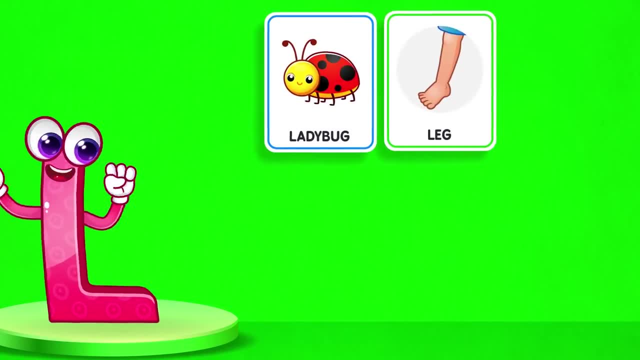 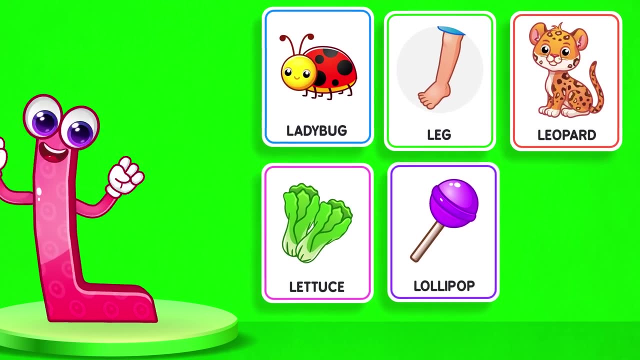 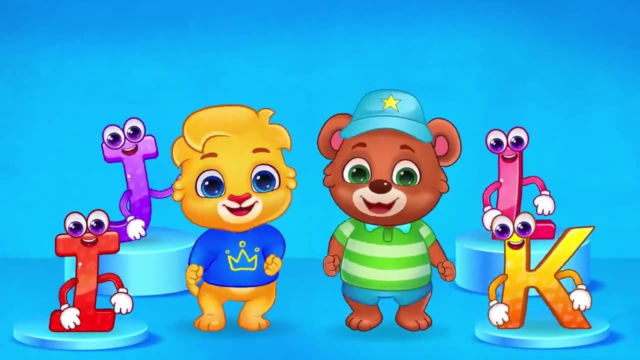 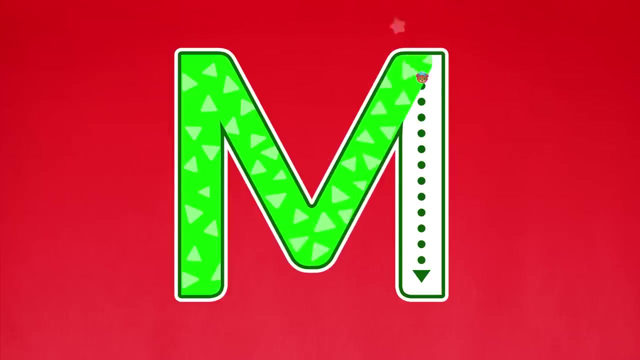 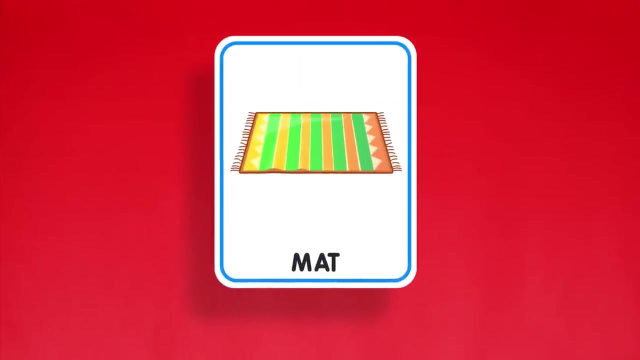 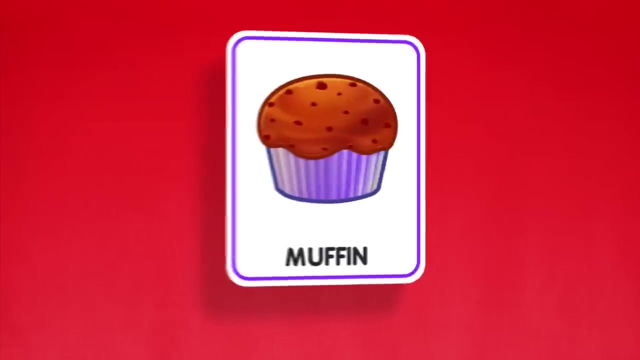 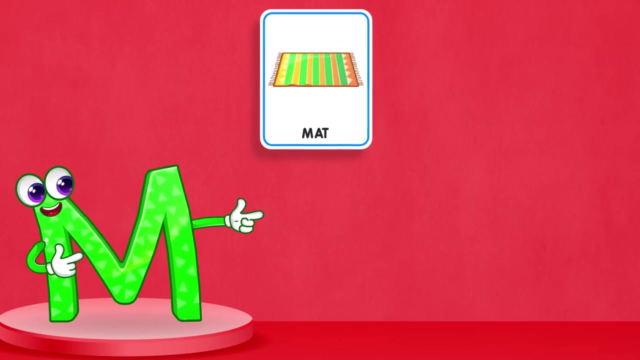 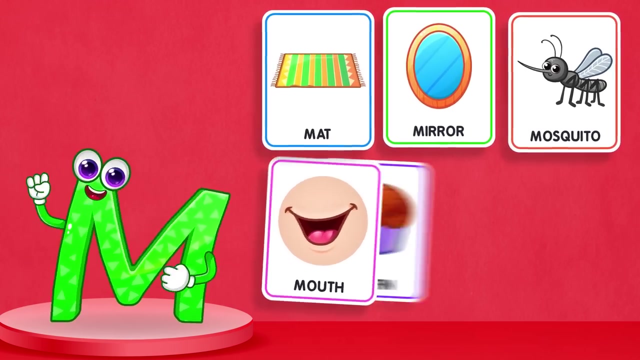 L is for Ladybug. Leg Leopard, Lettuce, Lollipop, Lotus M. This is M? M is for Ladybug. M is for Ladybug. M is for Mat Mirror Mosquito Mouth Muffin Mug. This is M. M is for Mat Mirror Mosquito Mouth Muffin. 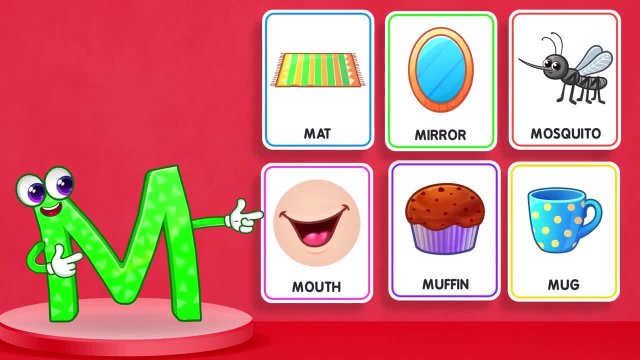 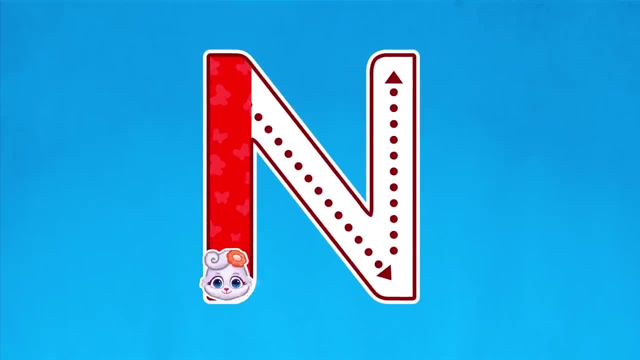 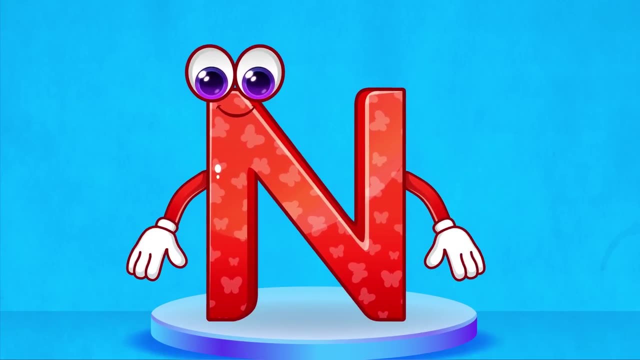 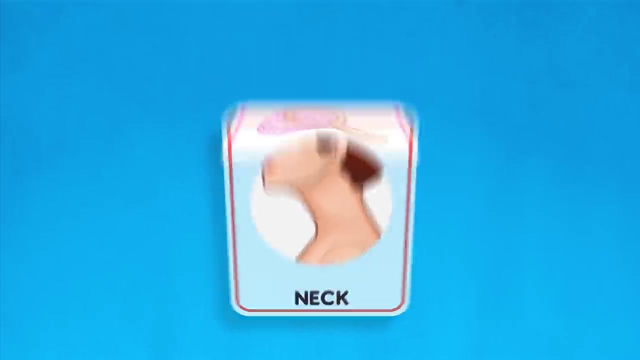 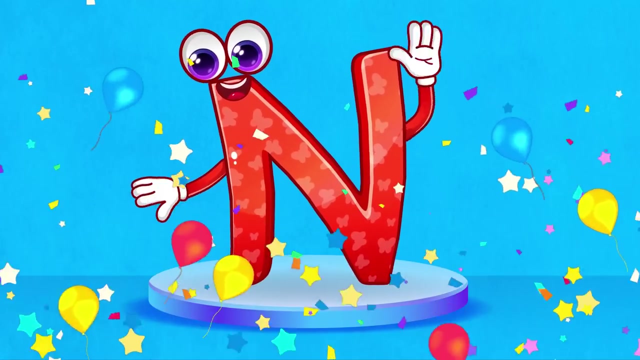 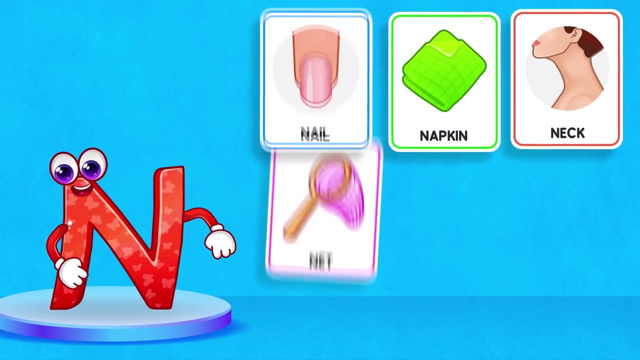 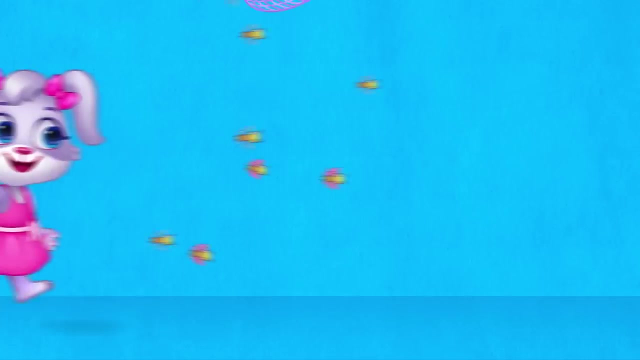 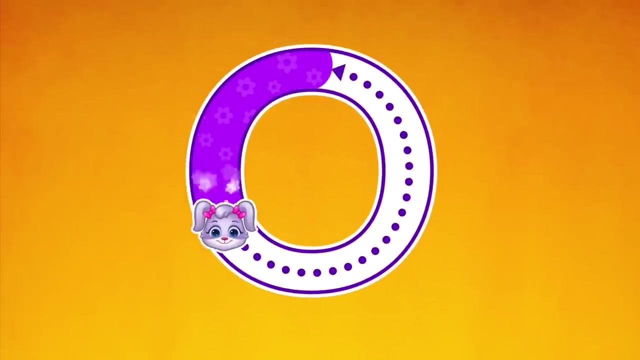 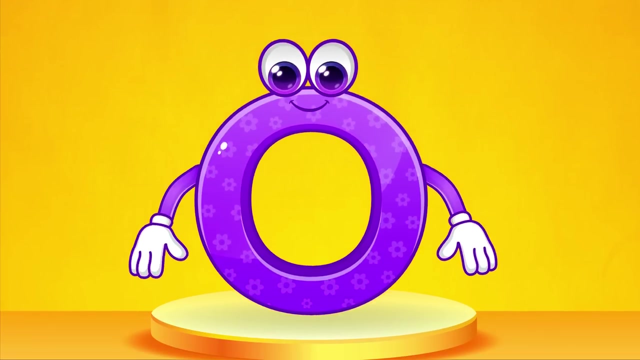 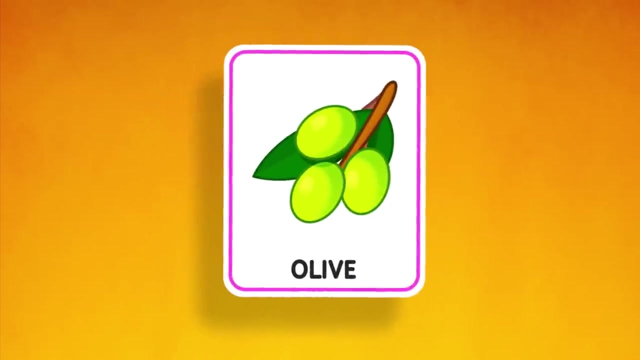 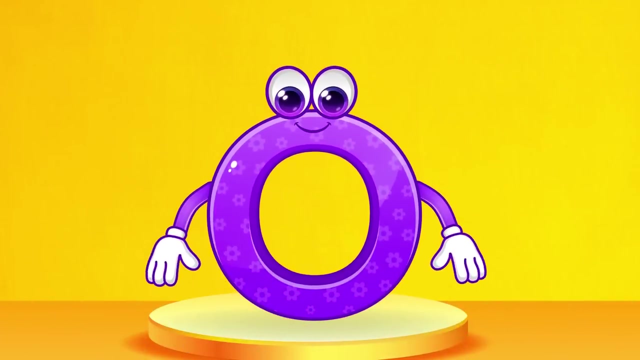 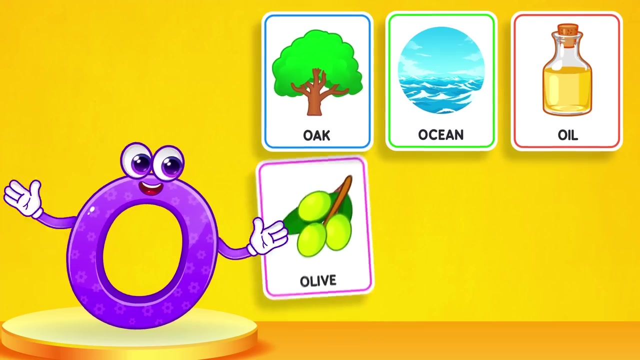 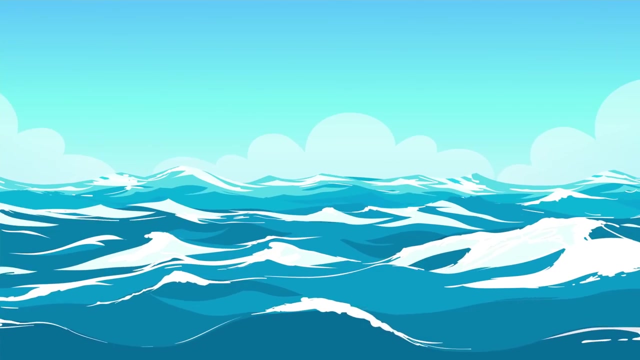 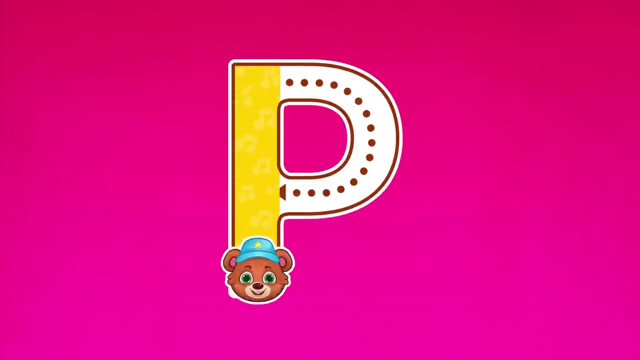 Mug Leopard Mouth Mouth Mouth Knot Wall fy Knit Nut Warm In Fil Neck Net Noodle Nurse. O. This is O. O is for Oak Ocean Oil- Olive Orchids- Ox. This is O. O is for Ork Ocean Oil, Olive Orchids Ox. P. This is P. 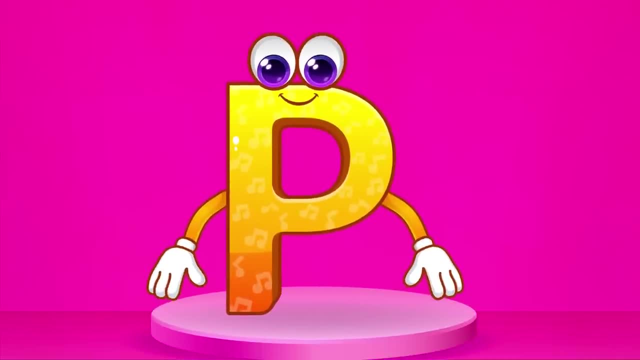 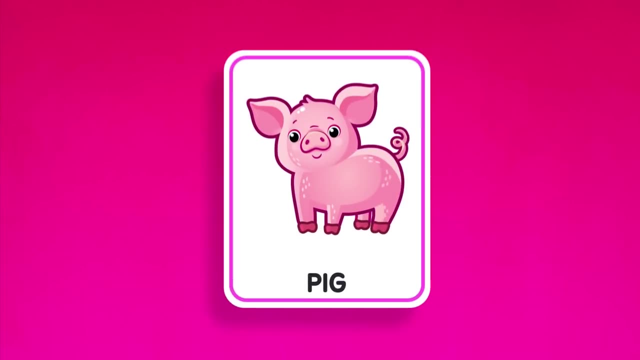 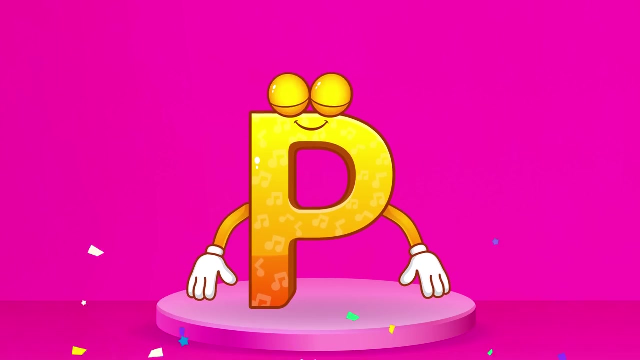 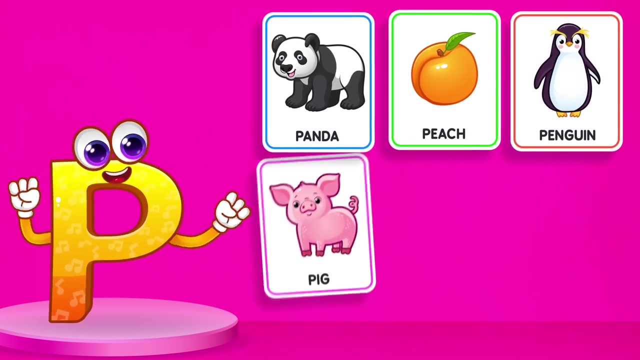 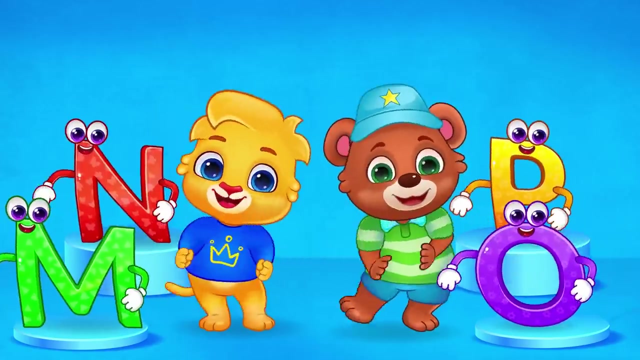 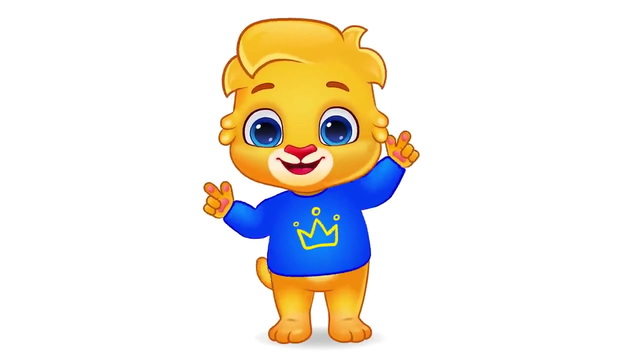 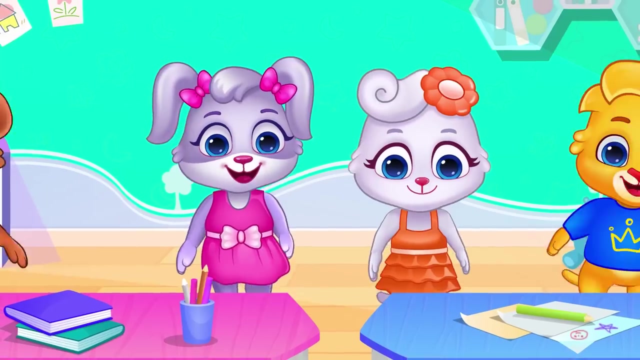 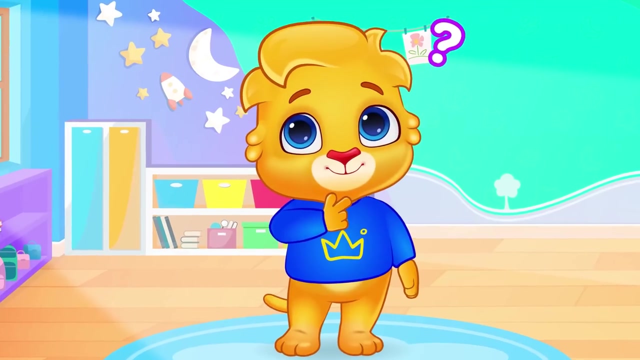 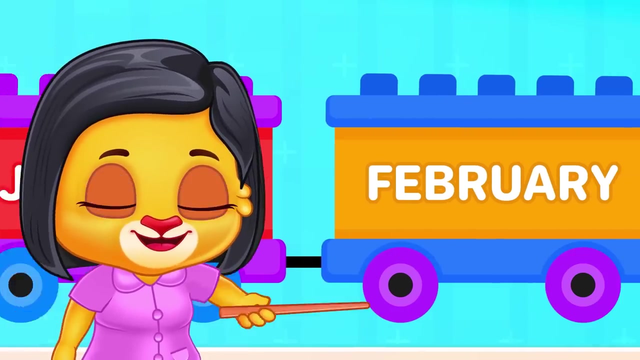 This is P. P is for Panda. P is for Panda Peach Penguin Pig Pot Pumpkin. This is P. P is for Panda: Peach Penguin Pig Pot Pumpkin. Hi kids, Welcome to class. Hello, Can anyone guess what we're learning today? Let's go January. 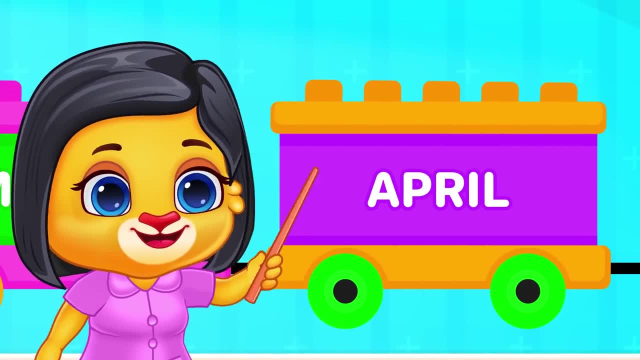 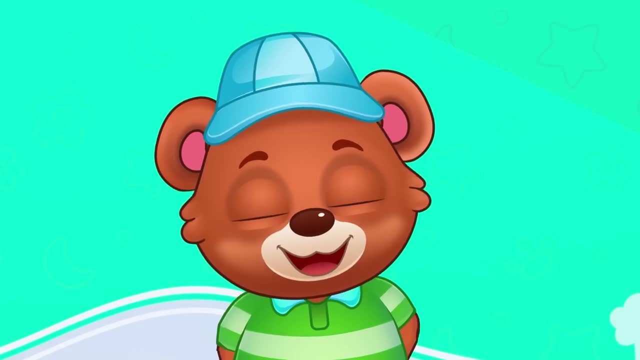 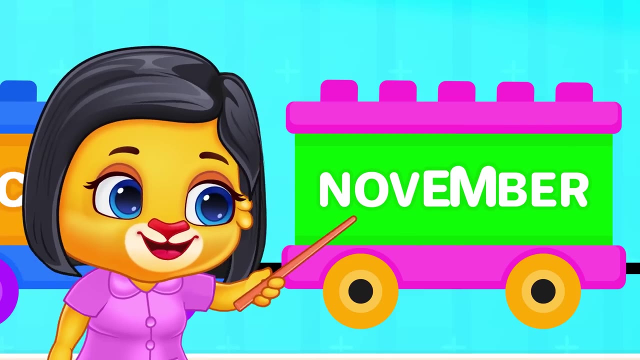 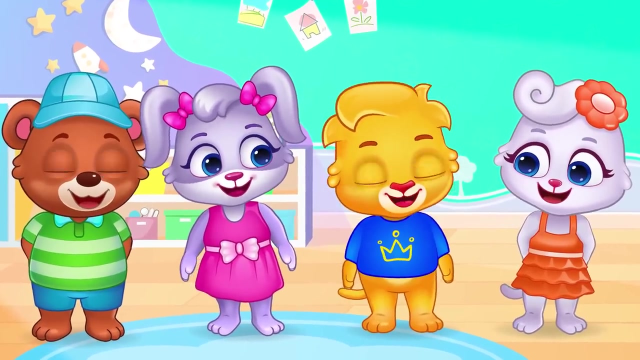 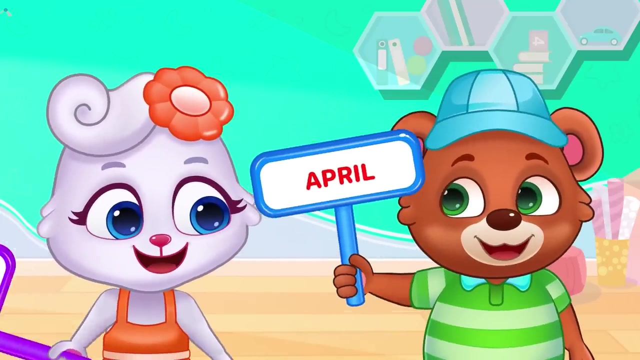 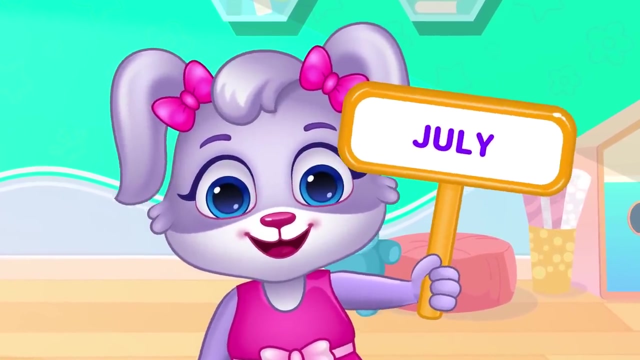 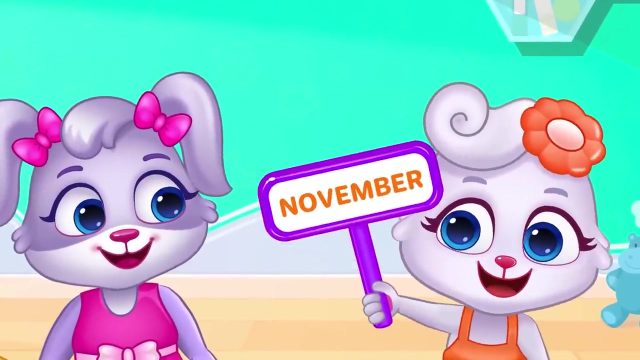 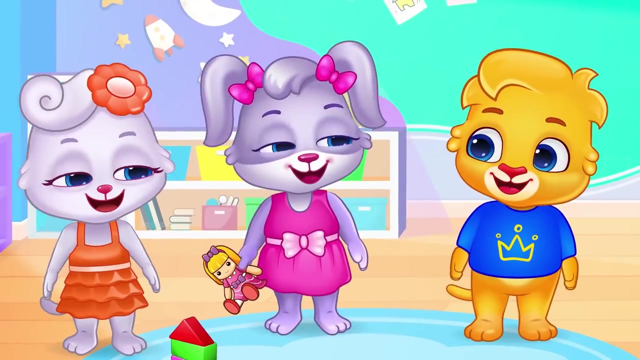 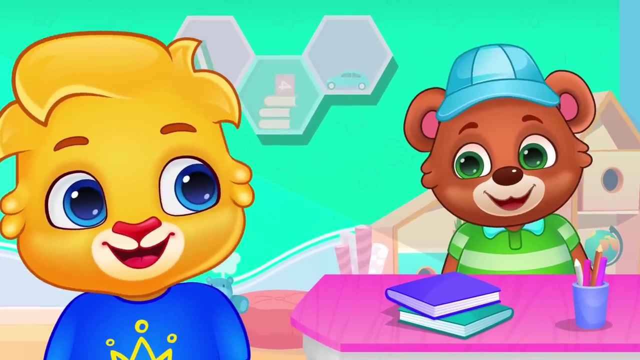 February, March, April, May, June, July, August, September, October, November, December. Let's say this again: Yes, January March, April, May, June, July, August, September, October, November, December. Can you repeat it with me? Can you repeat it with me: Yeah, January, January, February, February, March. 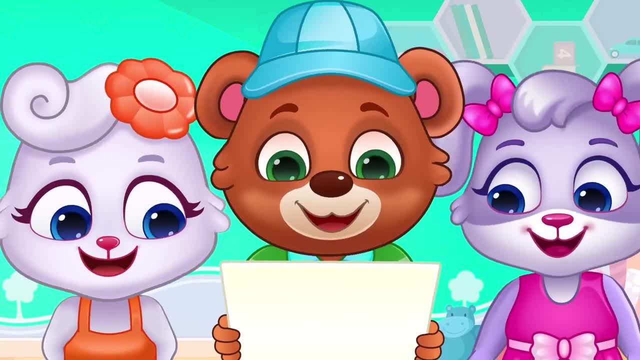 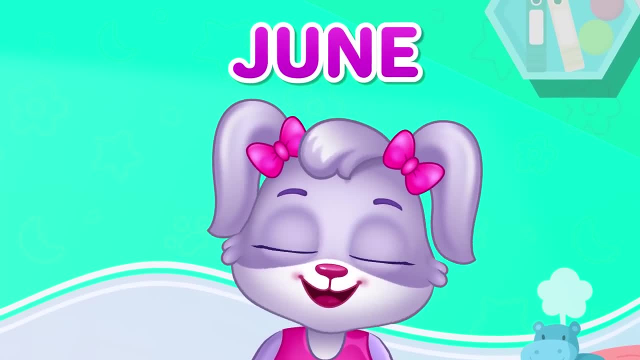 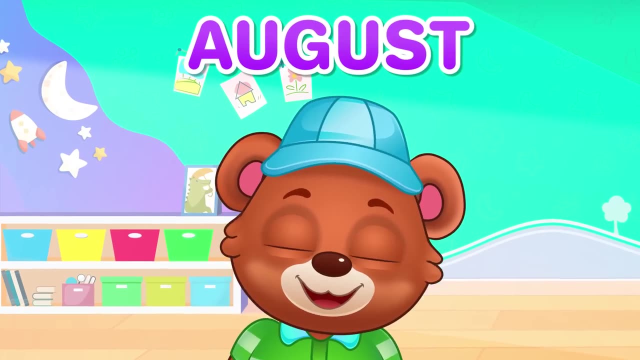 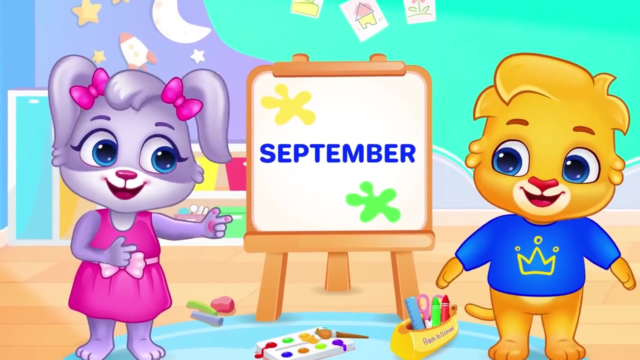 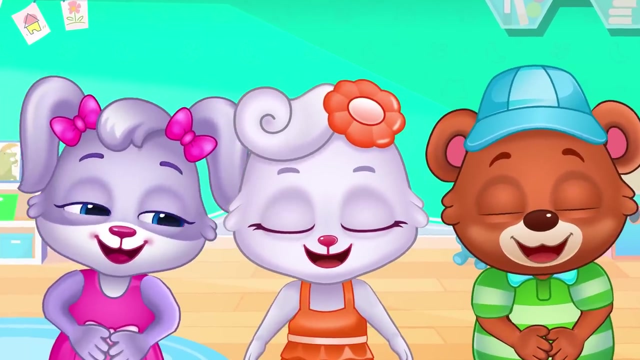 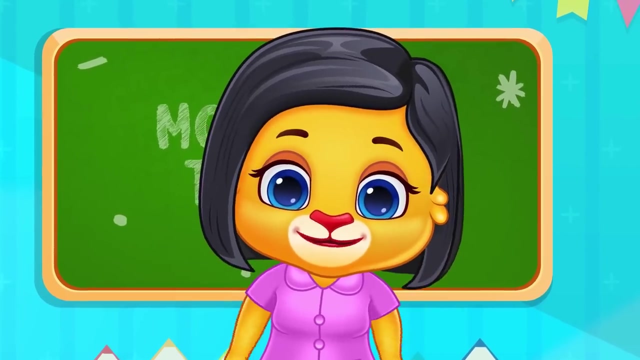 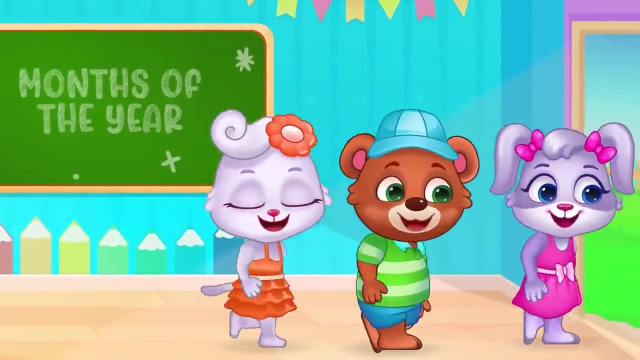 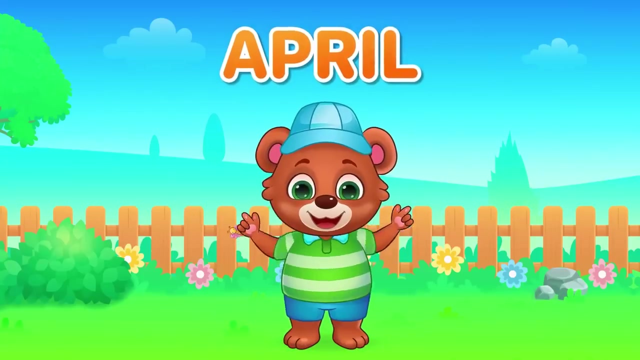 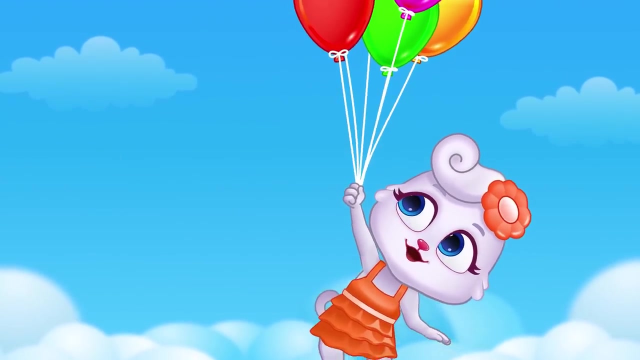 March, April, April, May, May, June, June, July, July, August, August, September, October, October, November, November, December, December. Very good children, Now it's time to dance. Now it's time to dance. Now it's time to dance. January, February, March, April, May, June, July, August. 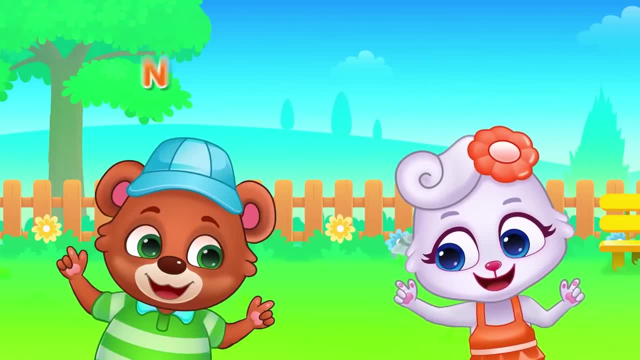 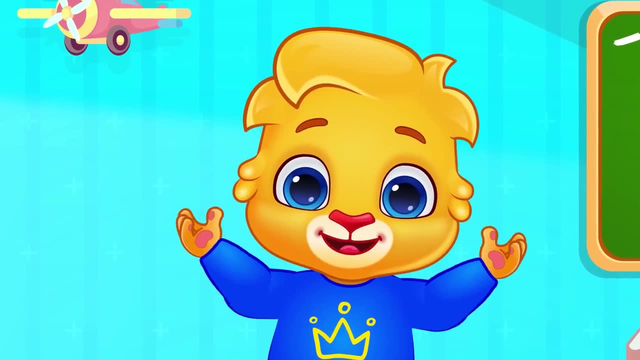 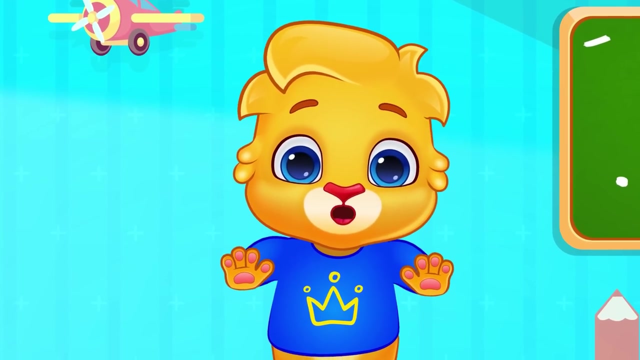 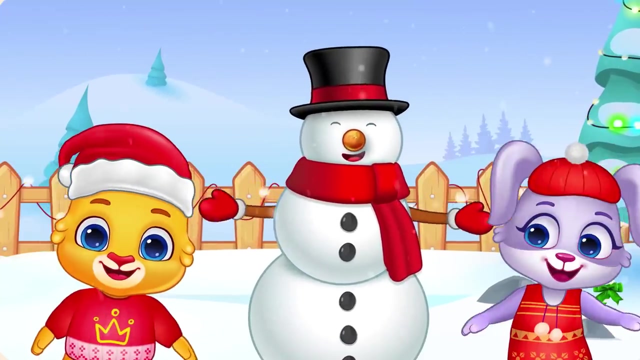 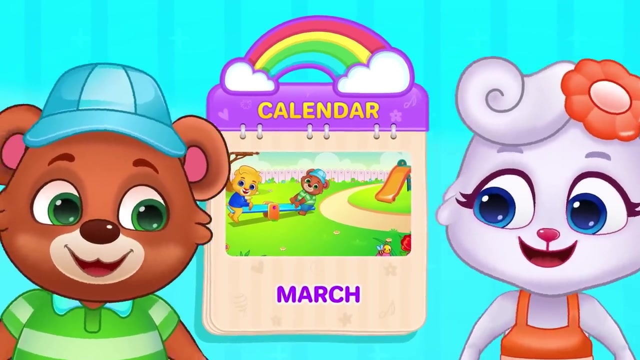 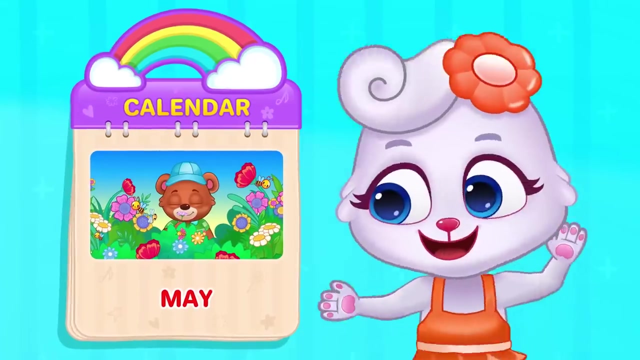 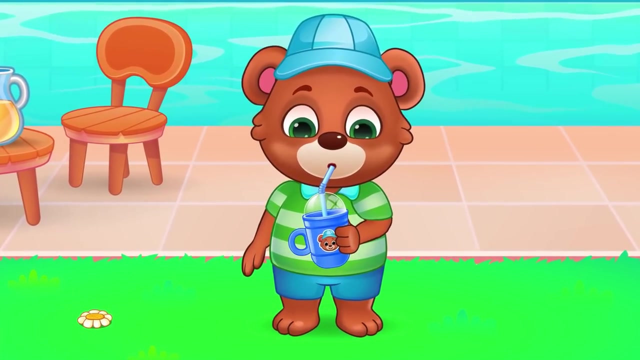 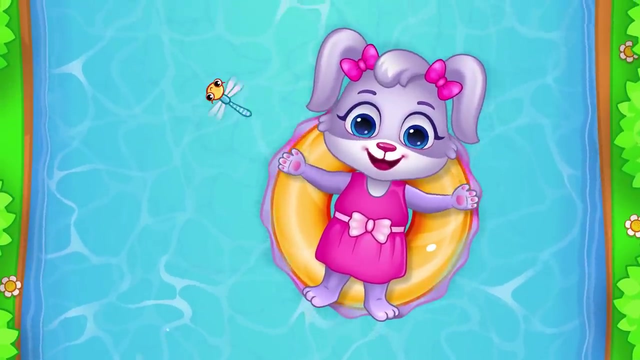 September, October, November, December. Hi, Let's sing it one more time to make sure we remember it, But this time very slowly. Are you ready? Yeah, January. Well, hello there, boys and girls. February, Woo, March, April, May, June, July, August, August. 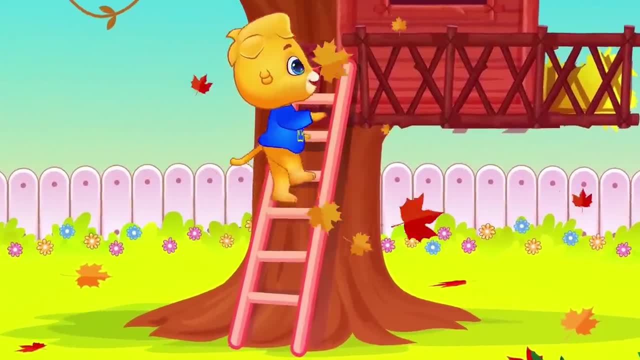 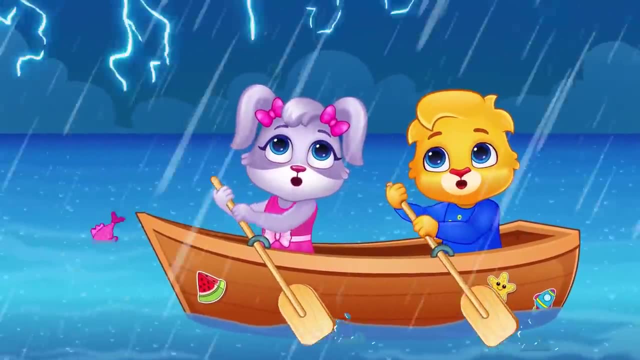 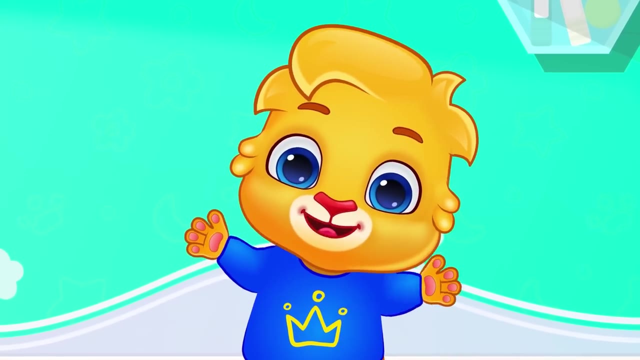 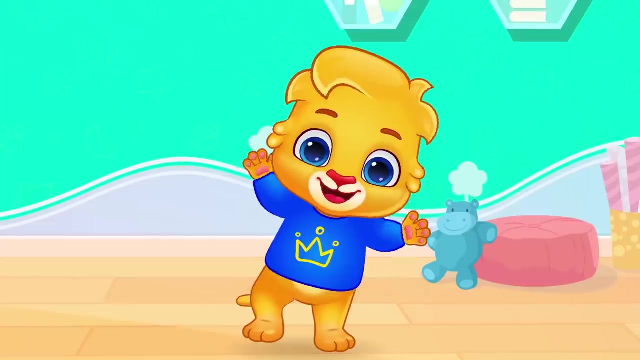 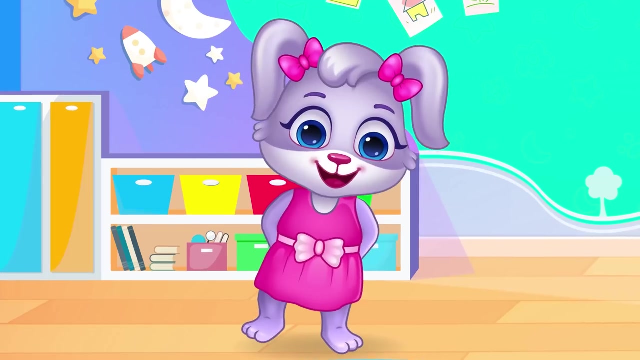 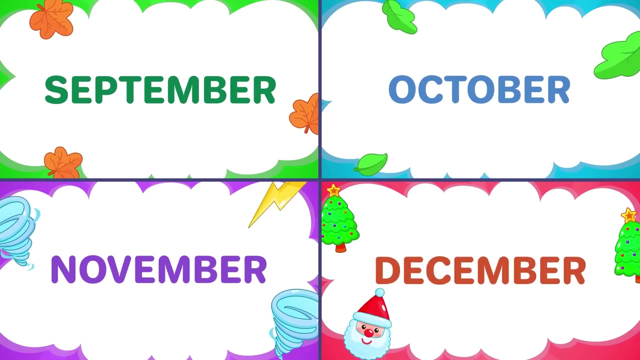 September, September, October, October, November, November, December, December. Hey, Now let's do it a little faster. Hey, Now let's do it a little faster. January, February, March, March, April, May, June, July, August, May, June, July, August, September, October, November, December, September, October, November, December. 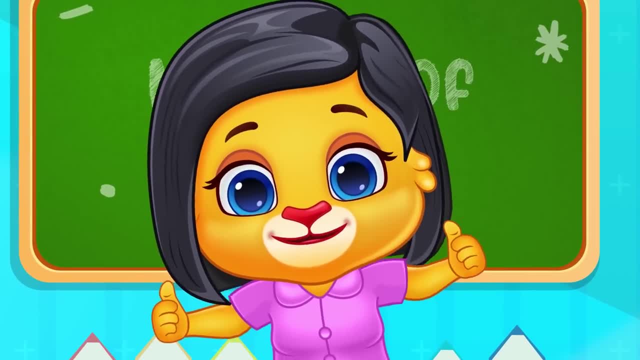 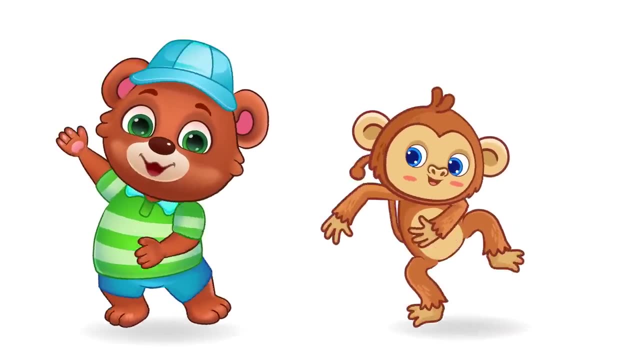 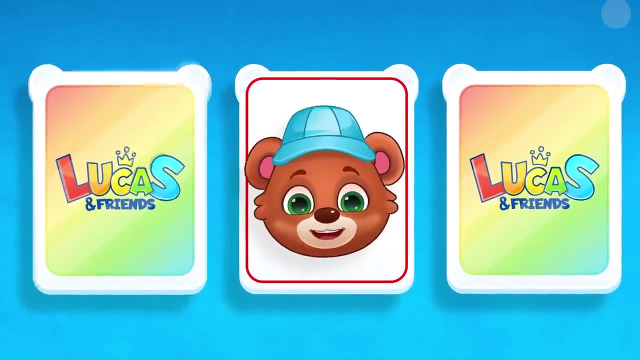 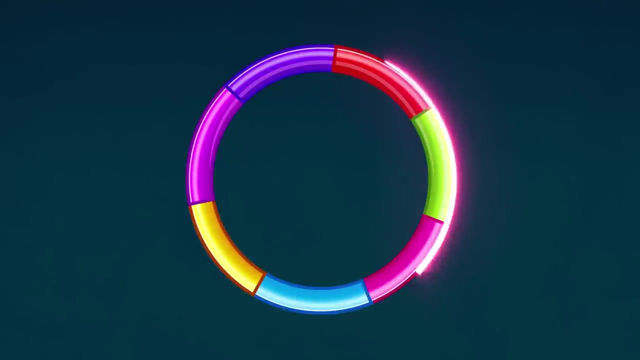 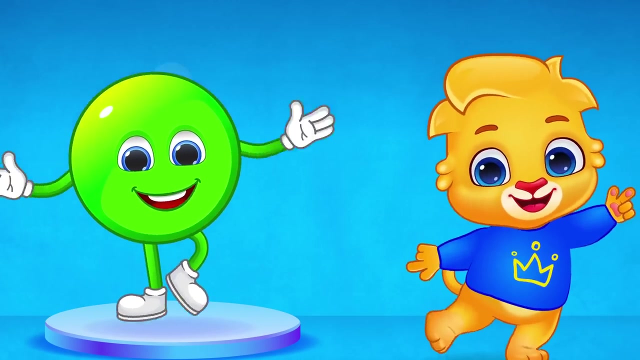 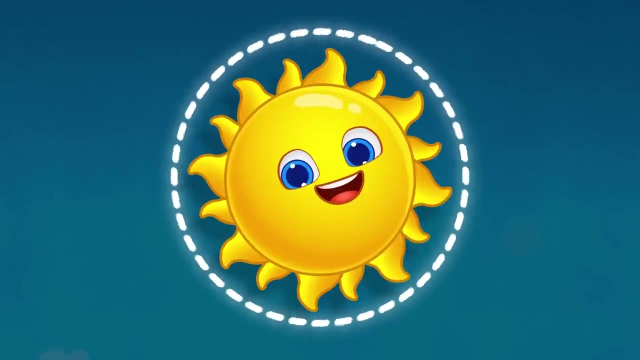 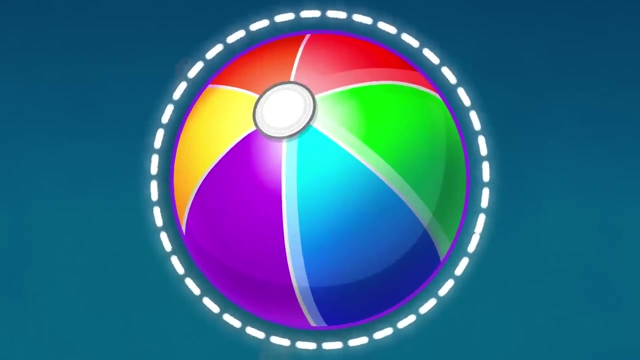 Woohoo, That was really fun. Very good children, Very good children. Laughter, Laughter, Laughter. Hula Hoop Ring, Hula Hoop, Ring, Hula Hoop, Ring, Circle Circle. This is Circle, Sun, Sun Circle, Ball Ball, Circle Donut. 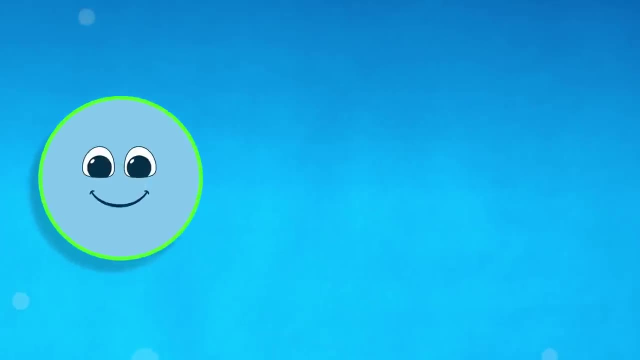 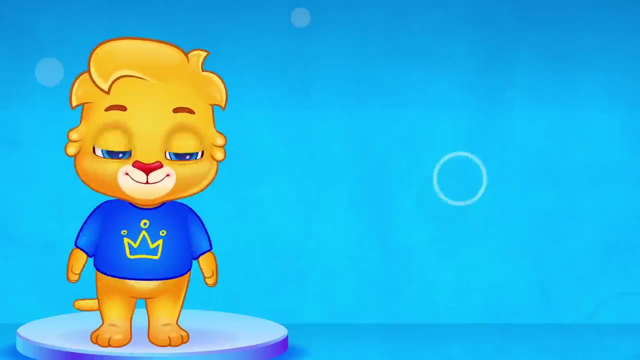 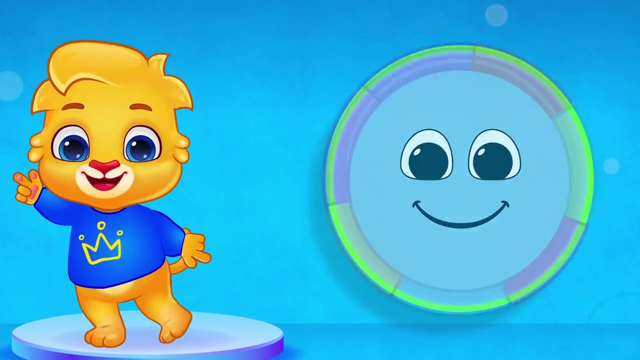 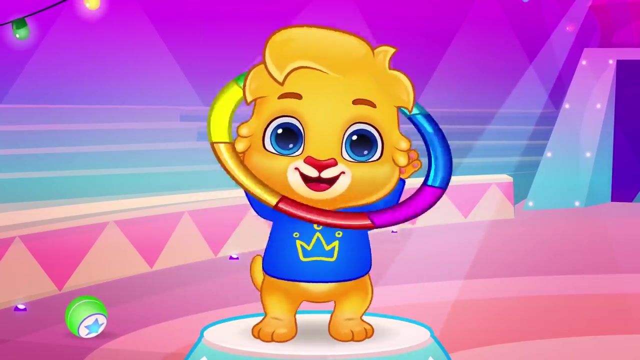 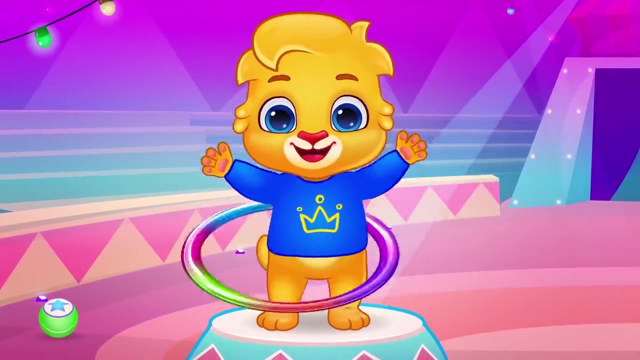 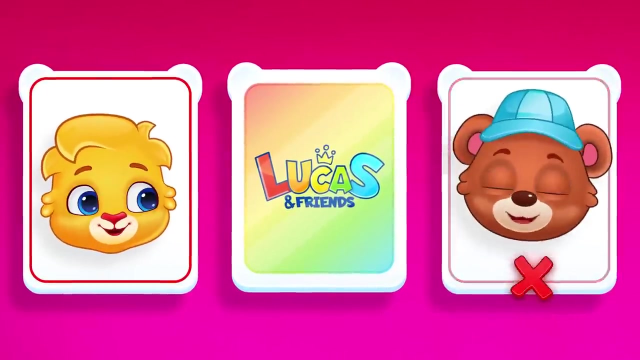 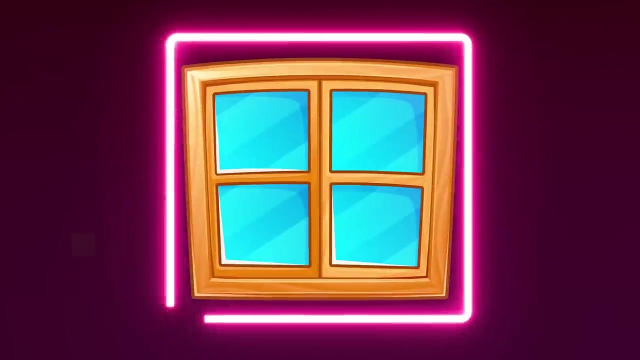 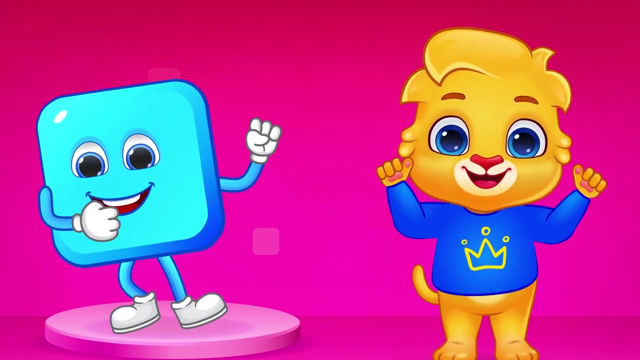 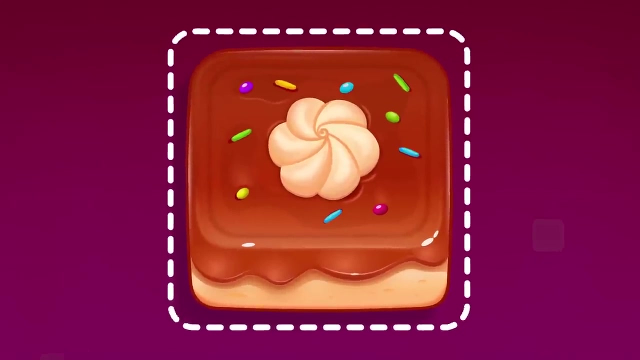 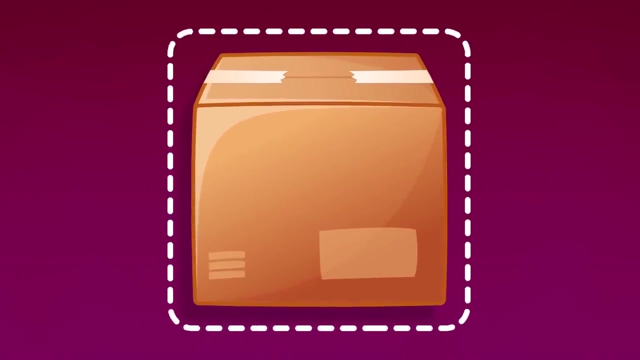 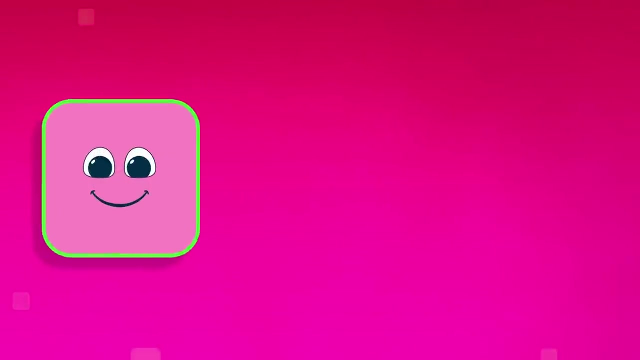 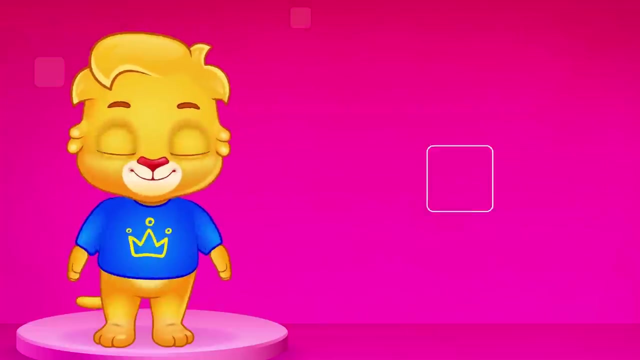 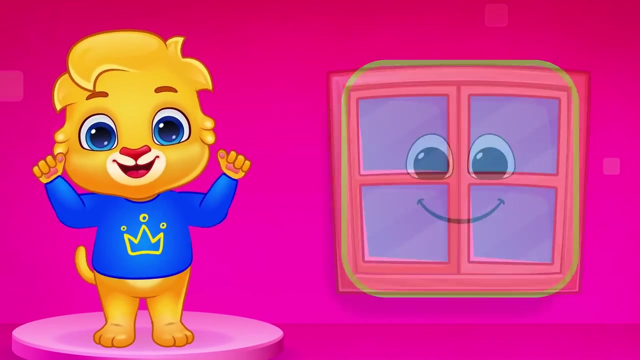 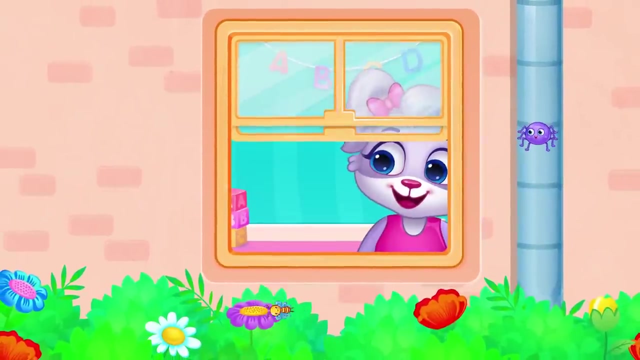 Donut Circle Circle Circle, Sun Ball. Donut Circle Circle, Circle, Circle, Circle, Circle Circle, Sun, Sun, Moon, Moon, Moon square, square square. this is square cake cake square box box square dice dice square, square, square. square cake box dice square, square, square. this window has a square shape. Ruby is looking out the window. 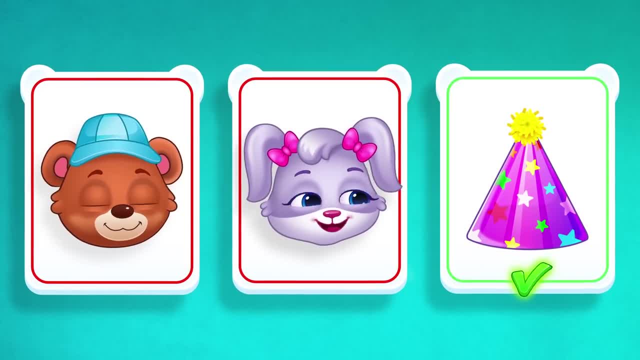 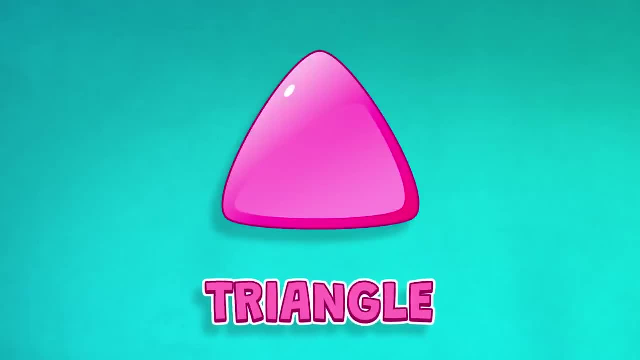 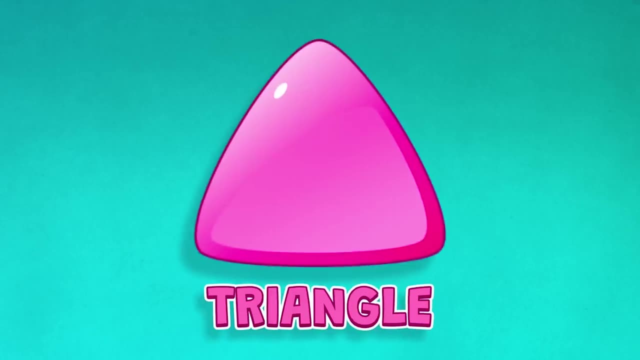 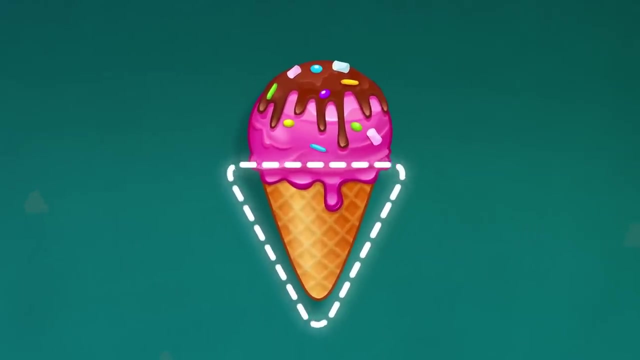 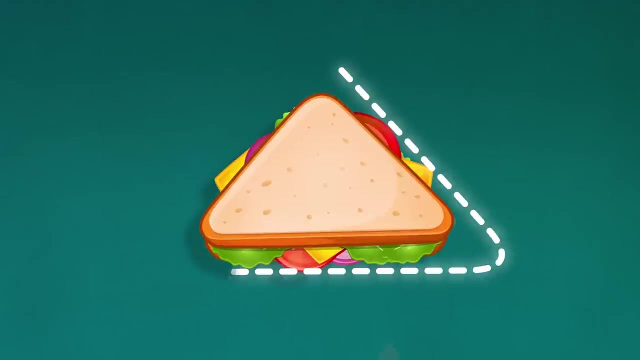 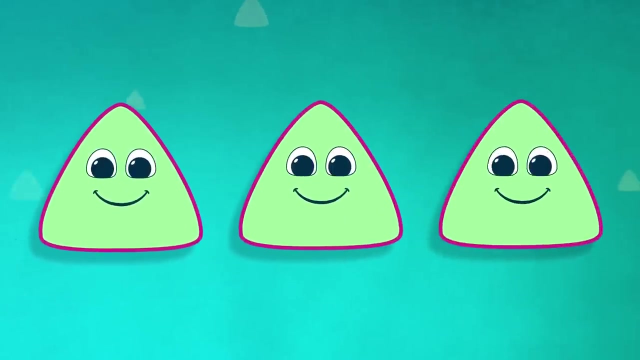 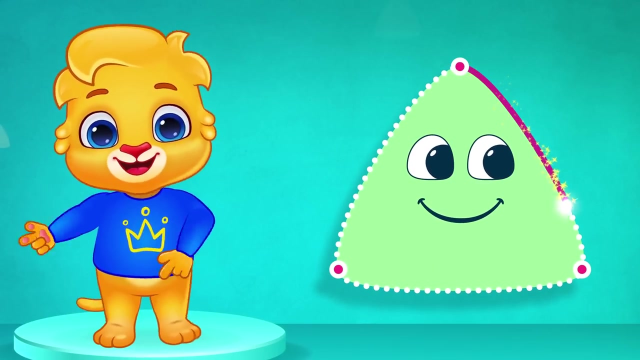 yeah, yeah, Oh. cap Camp triangle triangle triangle- video triangle- try and go. ice cream cone- ice cream cone triangle- tree tree triangle triangle. ice cream cone Sandwich Sandwich Triangle- Triangle Triangle Triangle- Ice cream cone Tree Sandwich Triangle- Hoorah. 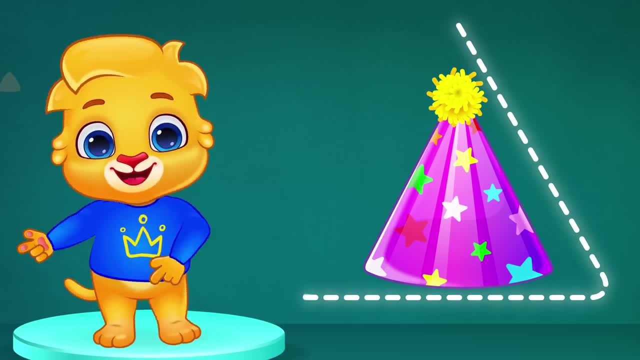 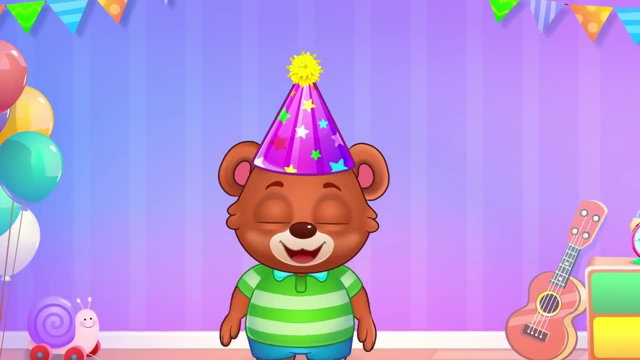 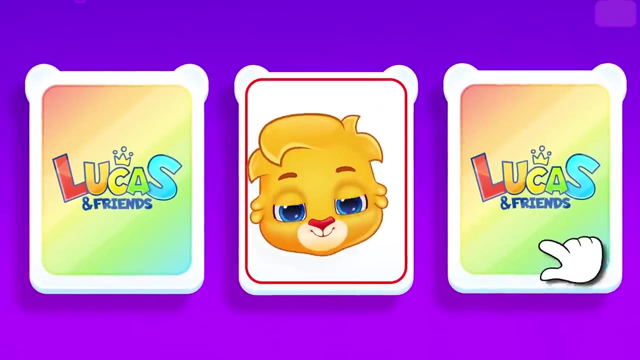 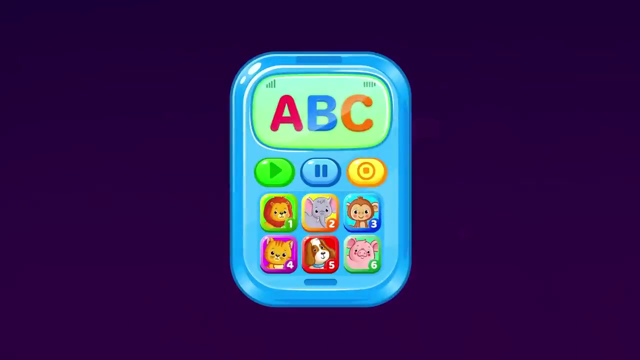 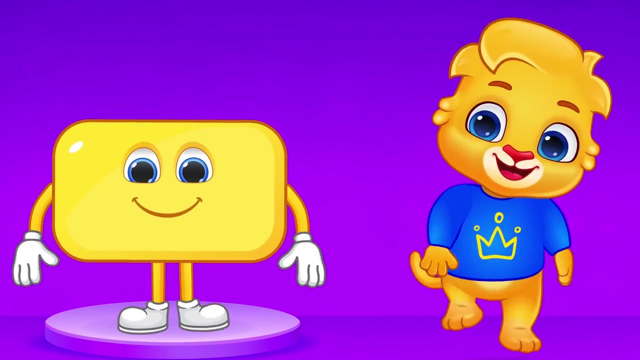 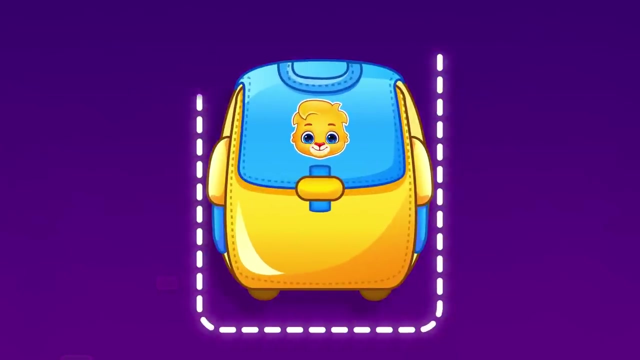 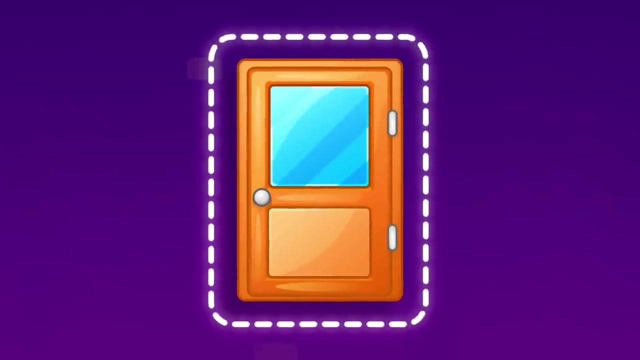 Triangle, Triangle. A birthday cap looks like a triangle shape. Brody's wearing a birthday cap. Ha ha, ha, ha ha, Phone, Phone, Rectangle, Rectangle, Rectangle. This is rectangle Bag. Bag, Rectangle, Door, Door Rectangle. 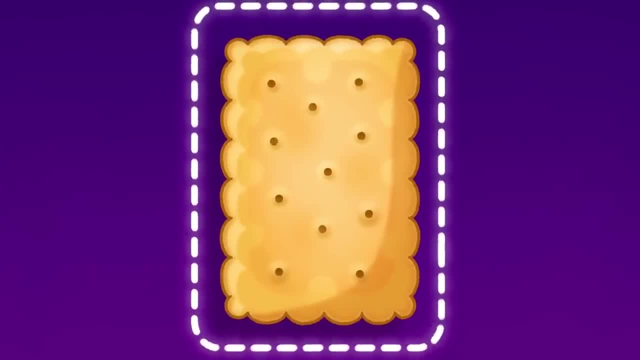 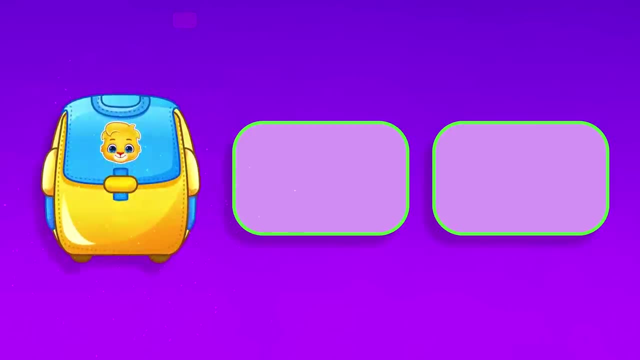 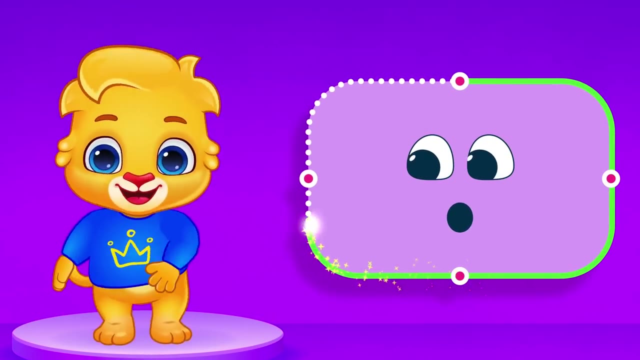 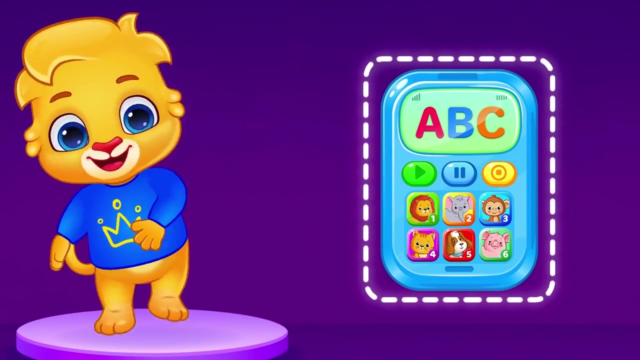 Biscuit Biscuit, Rectangle, Rectangle, Rectangle, Rectangle, Bag Door Biscuit Rectangle- Wow, Rectangle, Rectangle. The shape of a phone is a rectangle. Can you guess who's watching? Lucas is playing music on the phone. 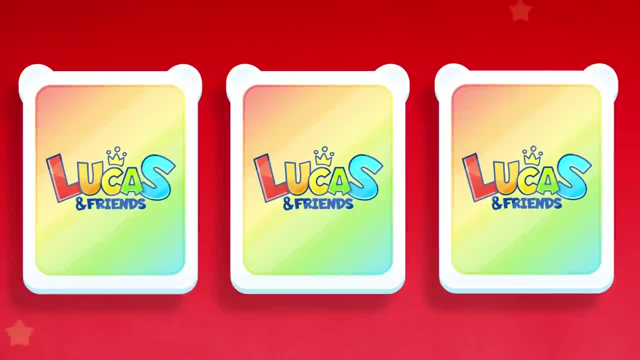 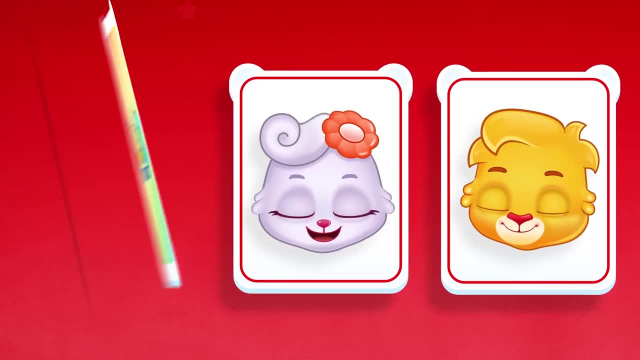 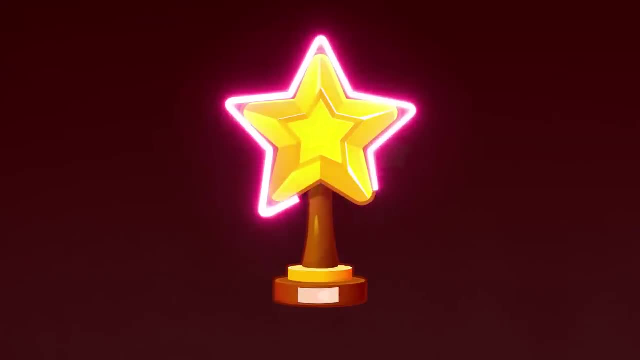 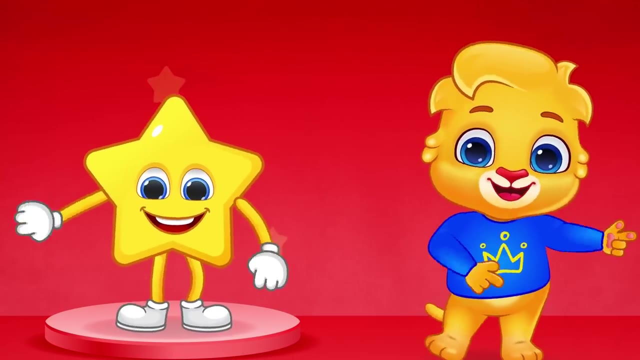 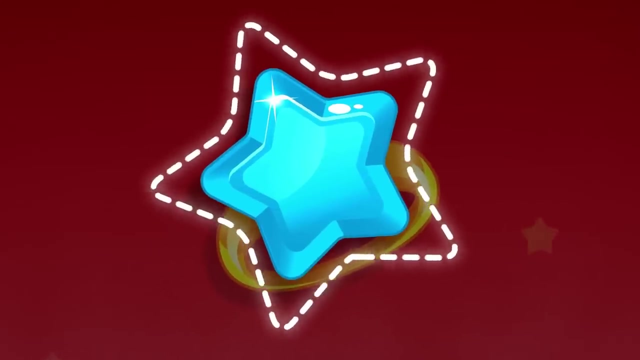 Trophy Aww Ha ha, ha, ha, ha, ha ha. Trophy Star Ha ha, ha, ha ha ha. Star. Hello Star Ha ha, ha, ha, ha ha. This is Star Star, star ring ring star starfish starfish. 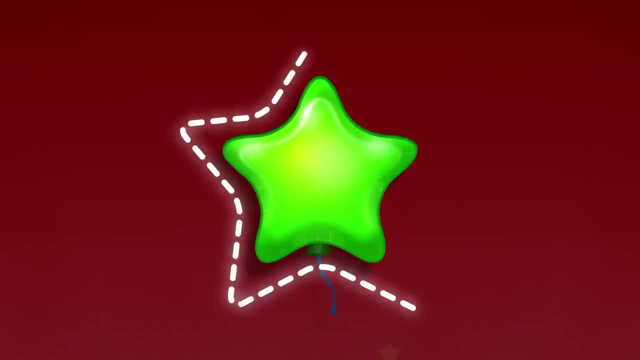 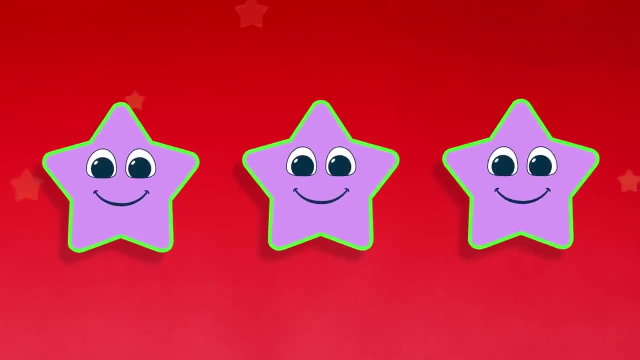 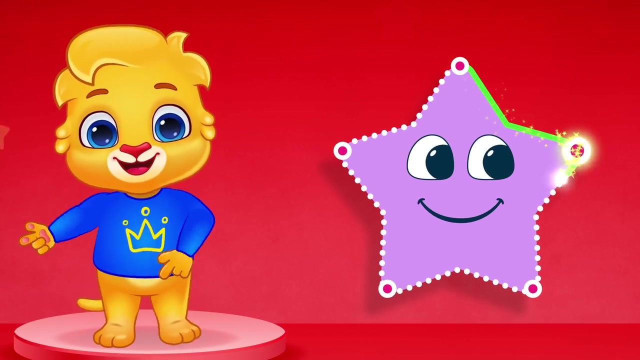 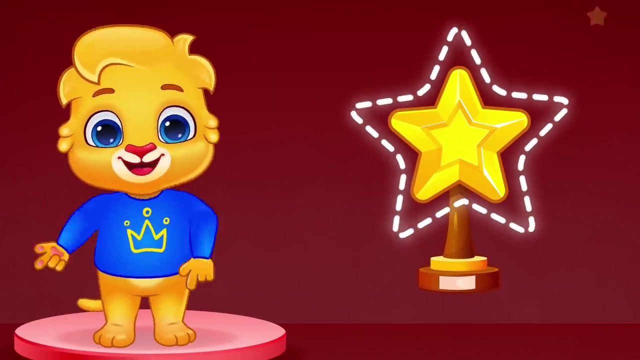 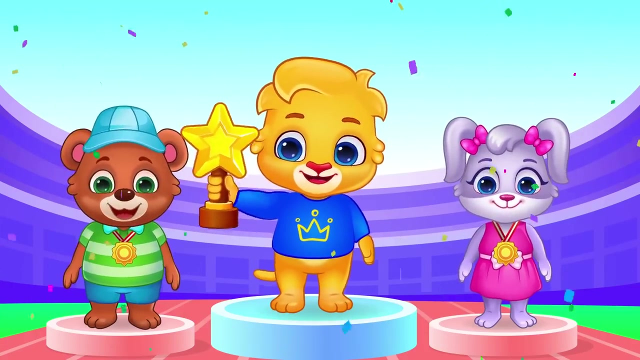 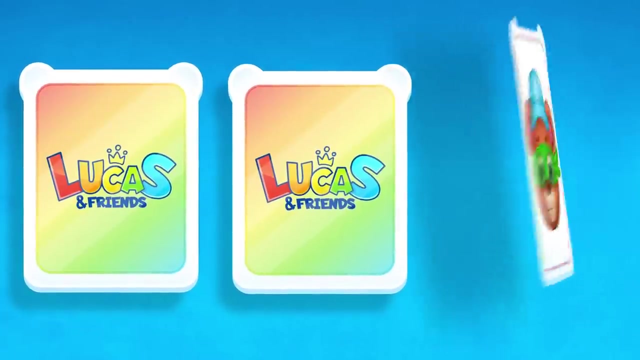 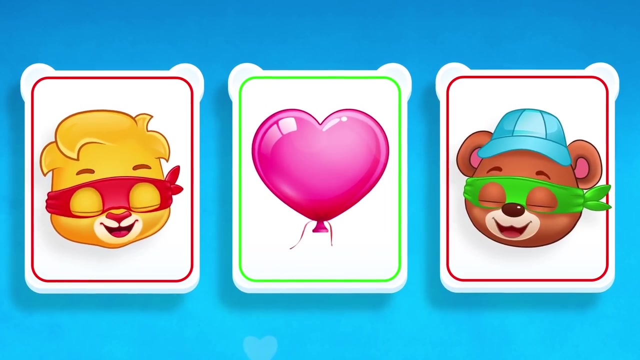 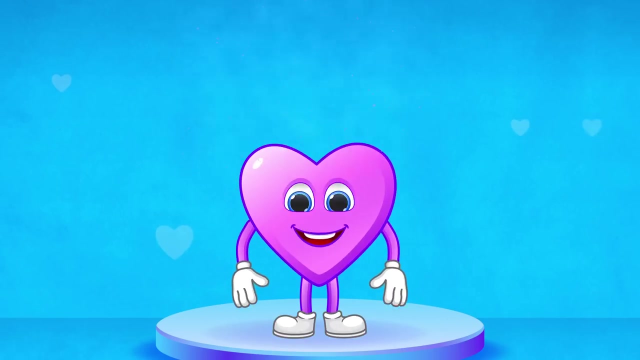 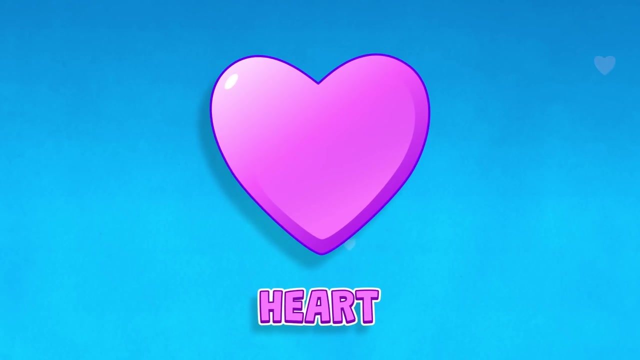 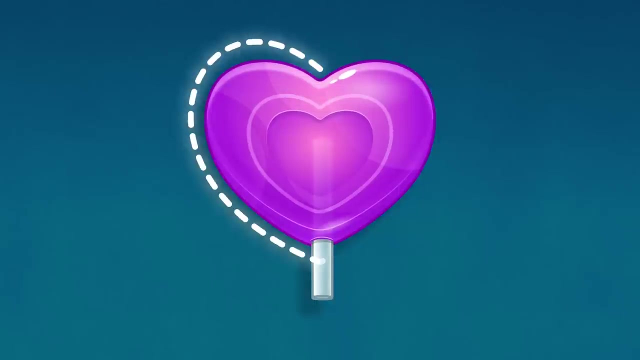 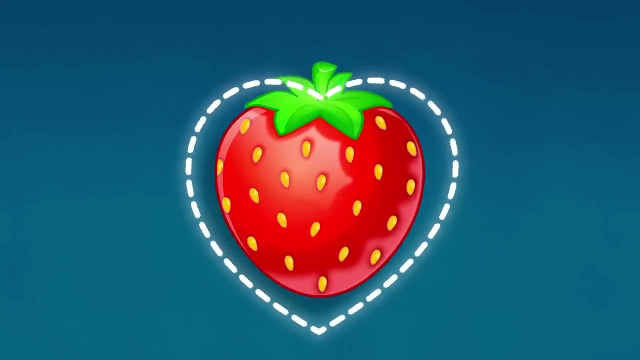 star balloon. balloon: star star, star, star ring. starfish balloon: star star, star star. The shape of this trophy is a star. Lucas won the star-shaped trophy in a tournament balloon balloon. balloon: heart, heart, heart. This is heart leaf, leaf, heart candy, candy, heart strawberry. 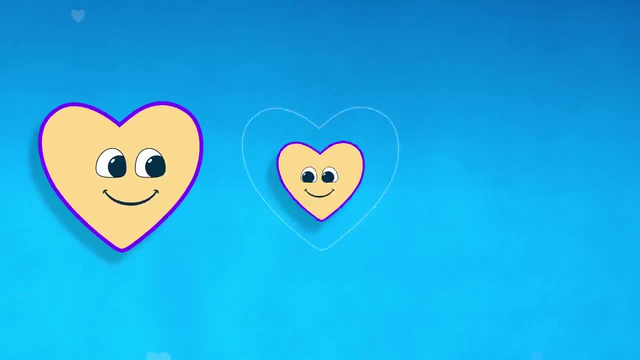 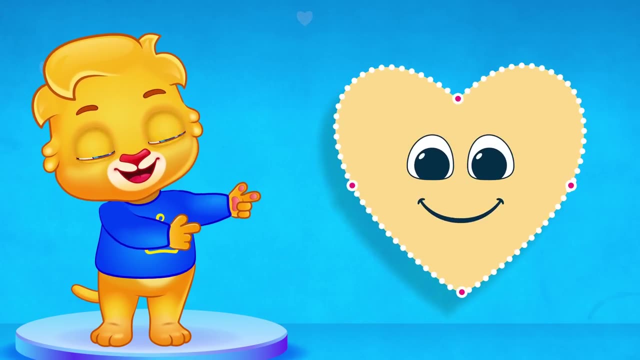 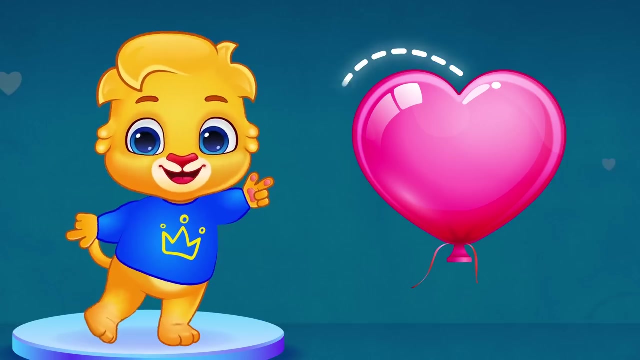 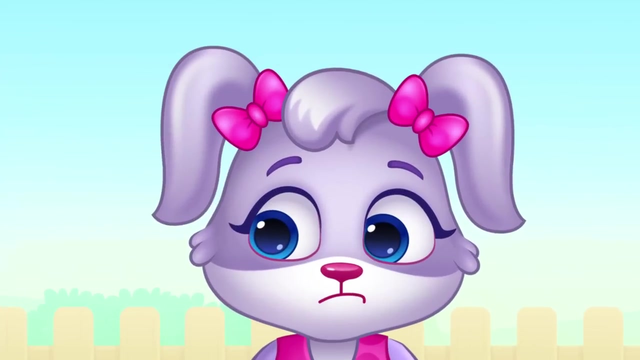 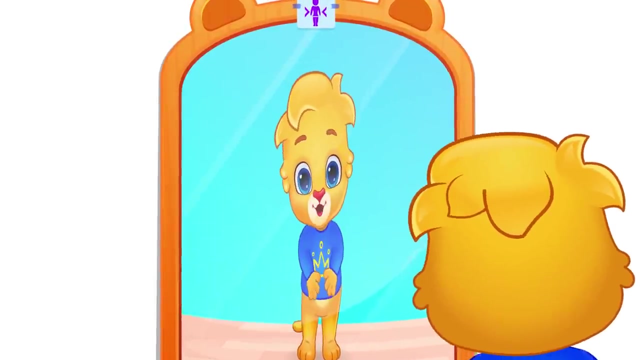 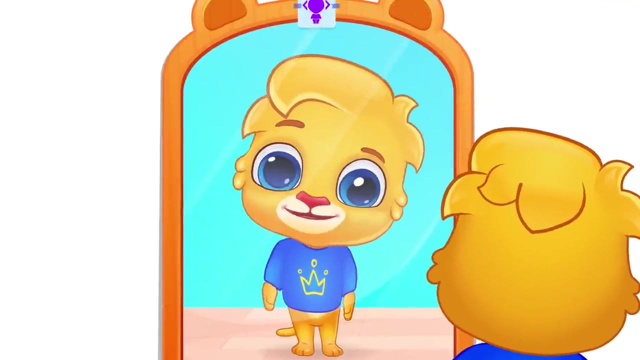 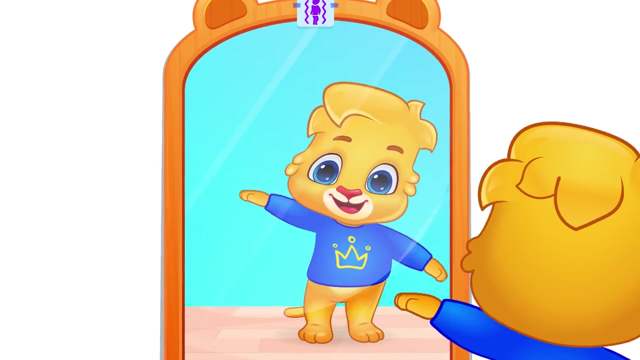 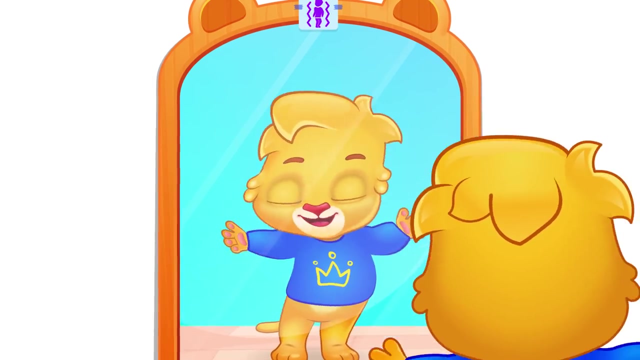 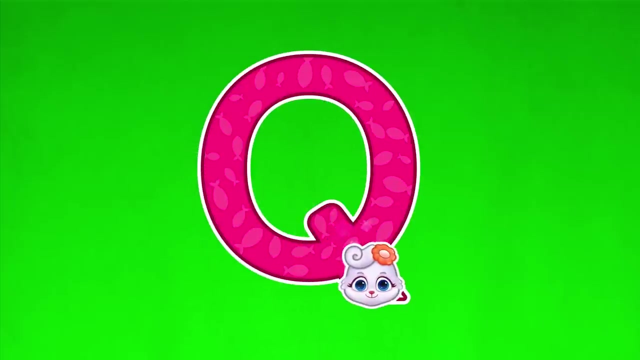 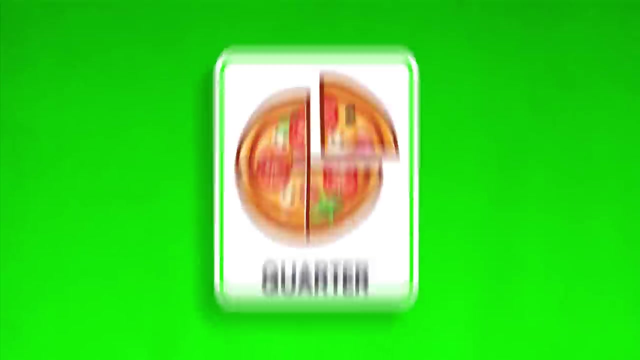 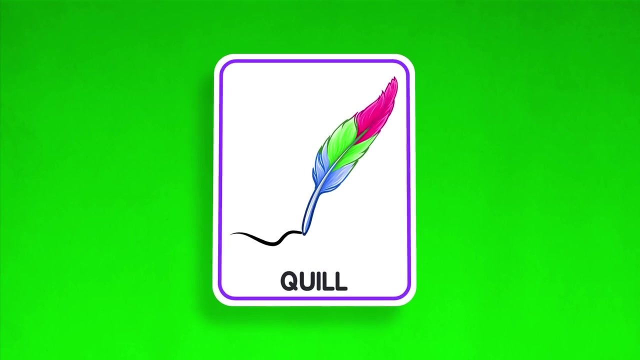 strawberry heart, heart, heart, leaf, leaf, Candy candy, strawberry. strawberry quiere, heart, quiere heart, heartbeat, heart, heartbeat, heart, heart, heart, heart. Town hte Tool, Tool, Hard Oh Q. This is Q? Q is for quail. Quarter Queen Q, Quill King walk. This is Q? Q is for quail. 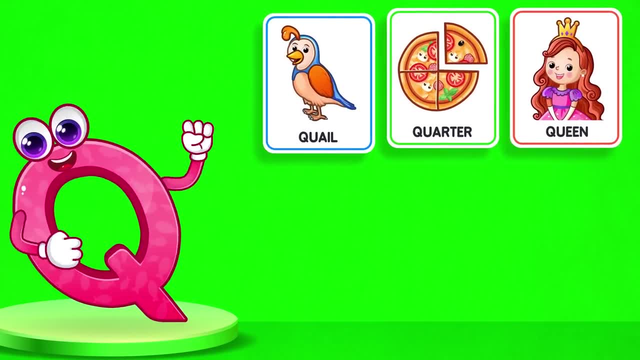 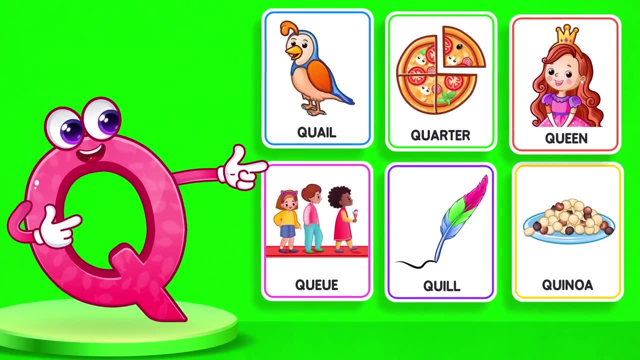 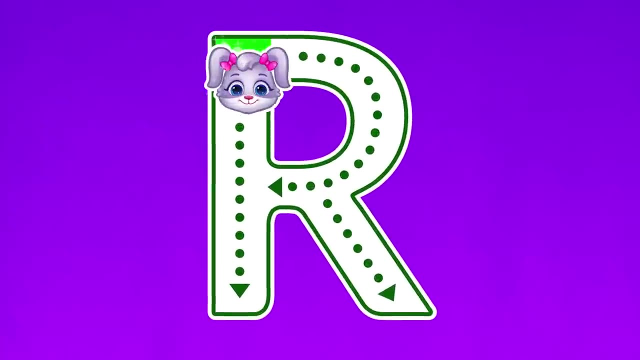 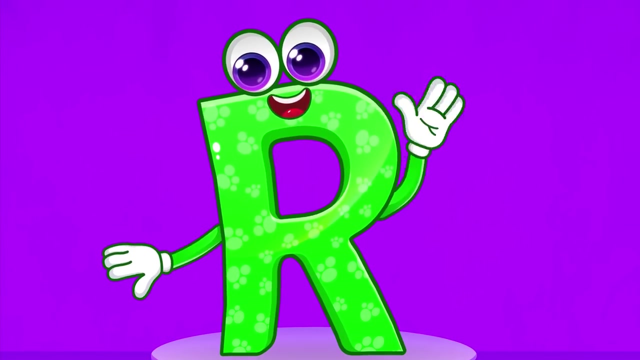 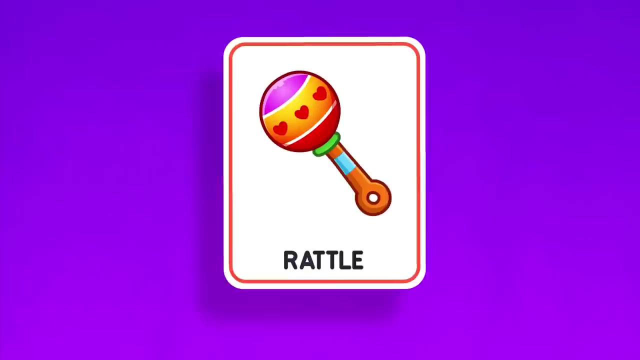 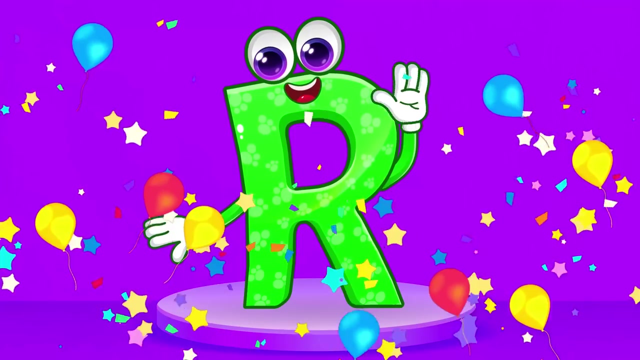 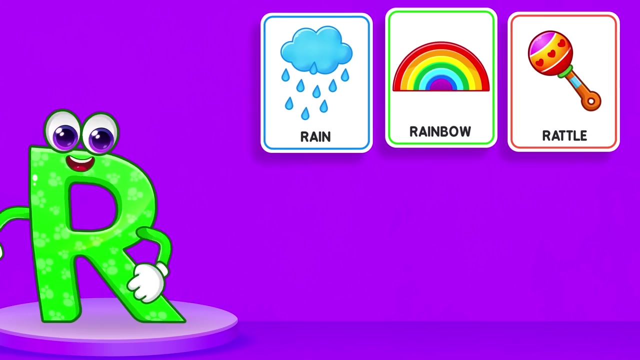 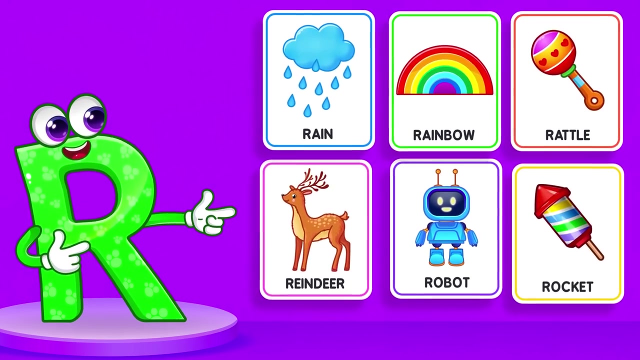 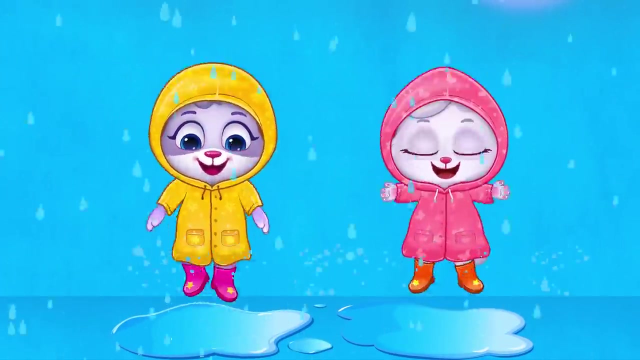 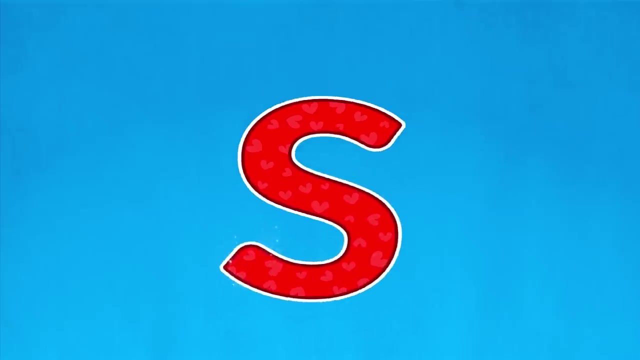 Quarter Queen. Q. This is Q. This is Q. Quill King walk. Aha R. This is R. R is for rain. Rainbow Rattle Reindeer Robot Rocket. This is R. R is for rain. Rainbow Rattle Reindeer Robot Rocket. S. This is S Hi. 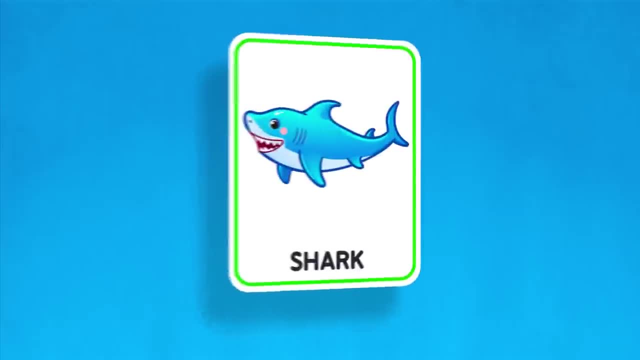 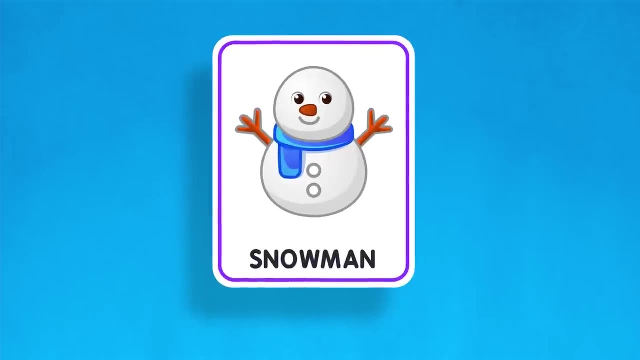 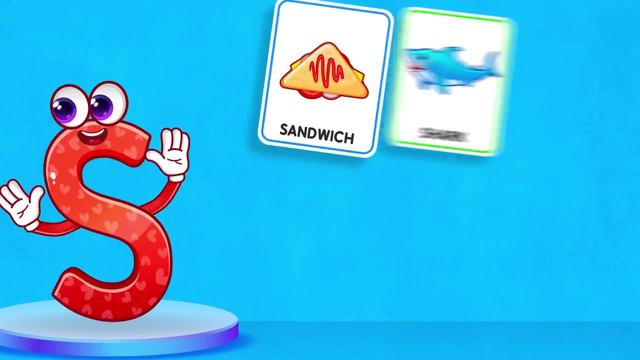 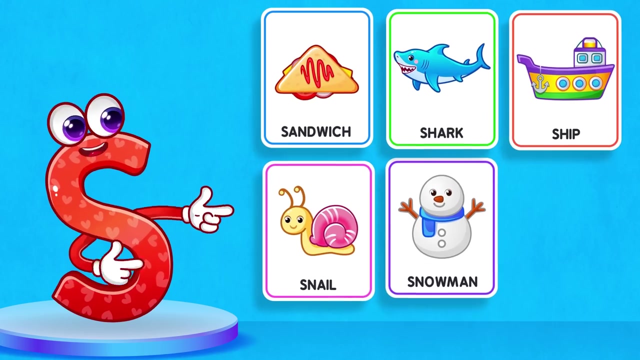 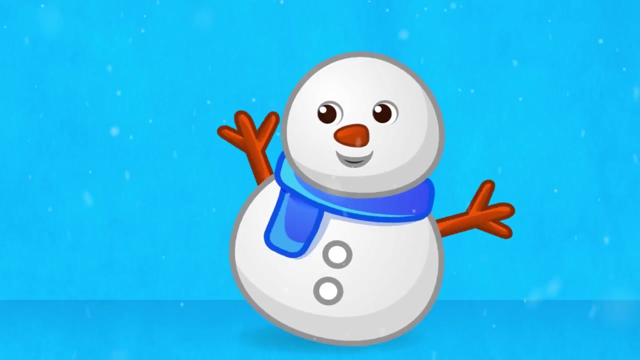 S is for sandwich Shark Ship Snail Snowman Swing. This is S. S is for sandwich Shark Ship Snail Snowman Swing. One S is for P, P, S is for Chips, S is for Tell, S is for, J Is for, T Is for, H Is for 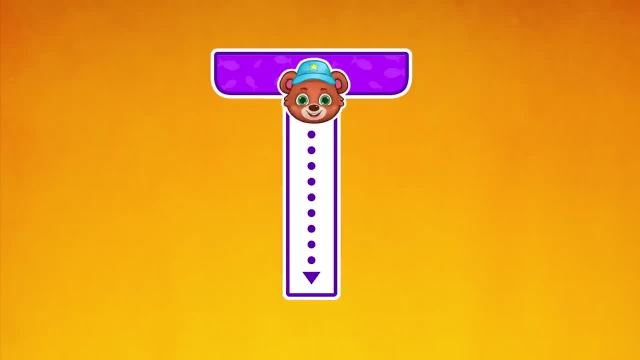 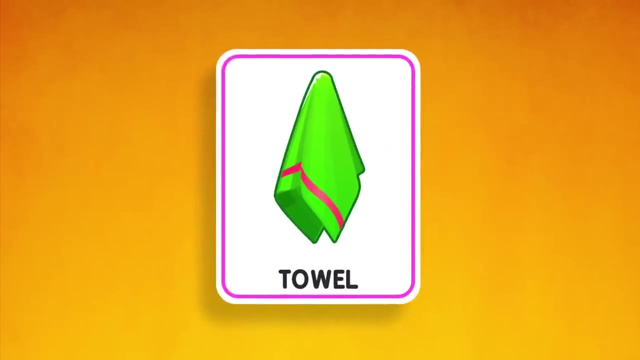 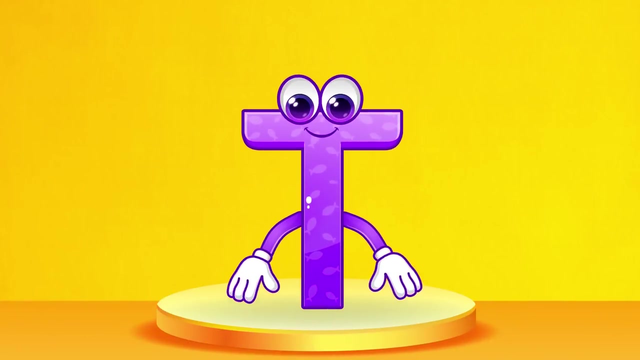 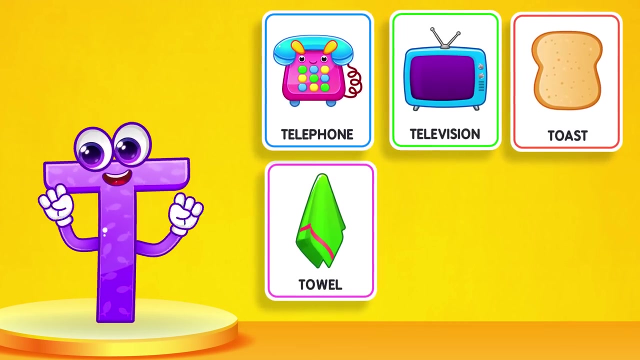 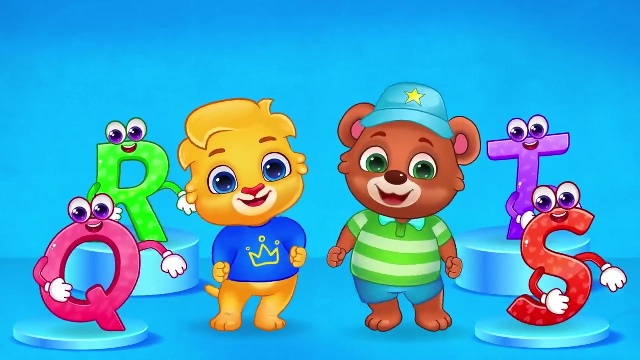 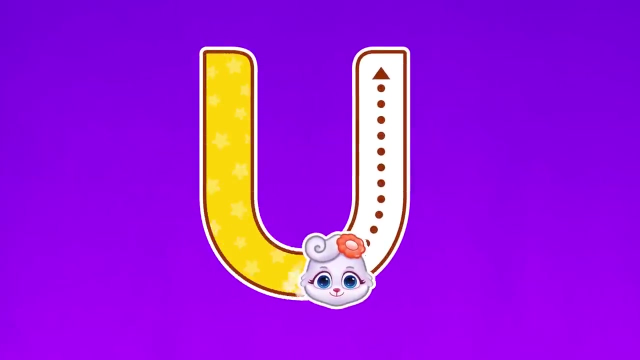 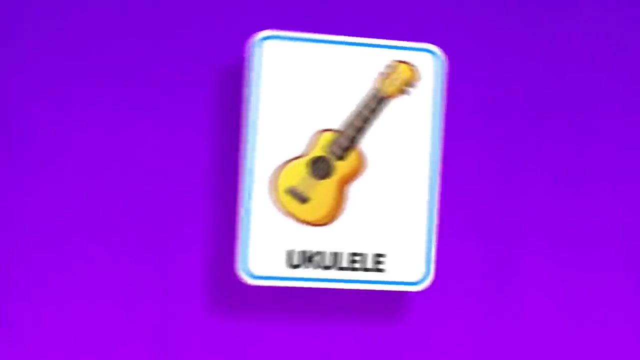 D Is for A Is for Ya. This is T. This is T. Hi Is for A Ss. T Is for Telephone Television. Toast, Towel, Toys, Turtle. This is T. This is T. T is for TELEPHONE TELEVISION. TOAST, POWEL, TOYS, TURTLE. U. this is U. U is for UKULELE. 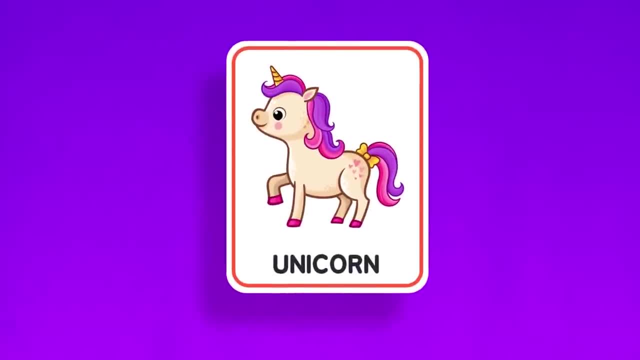 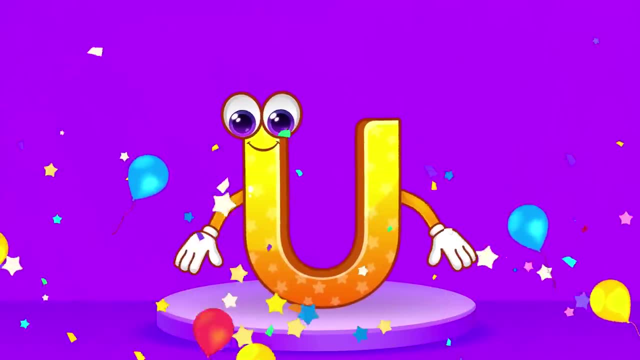 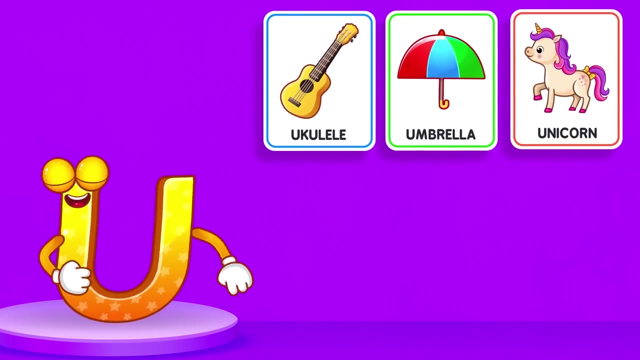 UMBRELLA UNICORN UNICYCLE UNIFORM URCHIN. this is U? U is for UKULELE. UMBRELLA UNICORN UNICYCLE UNIFORM URCHIN. 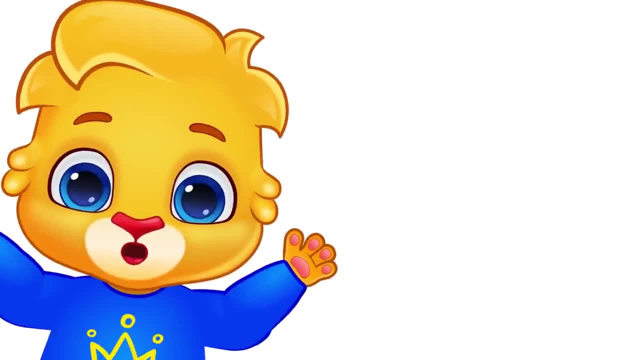 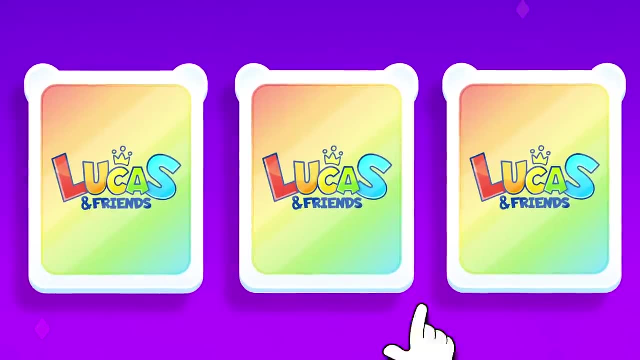 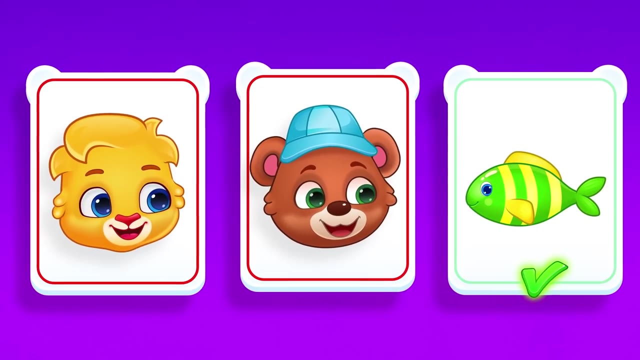 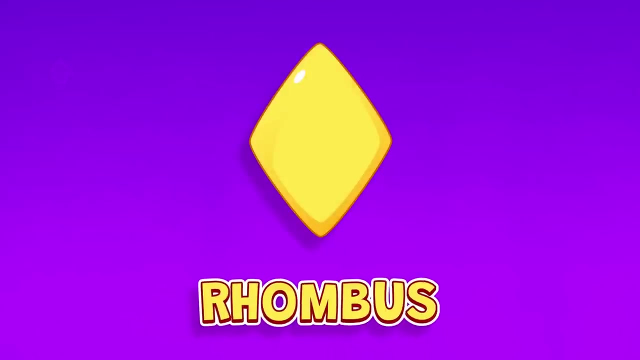 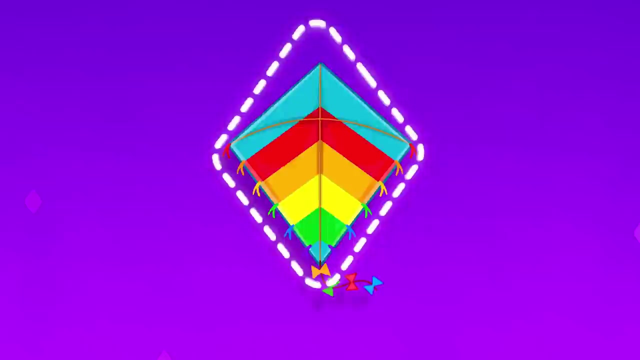 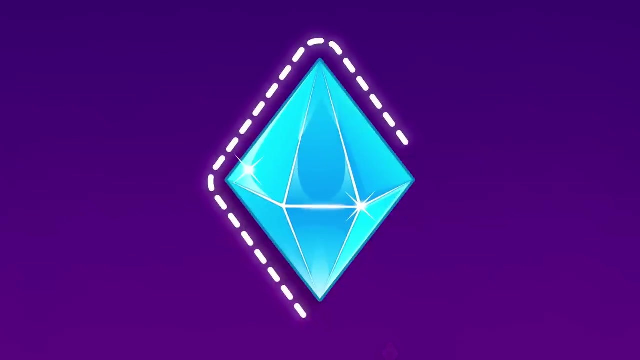 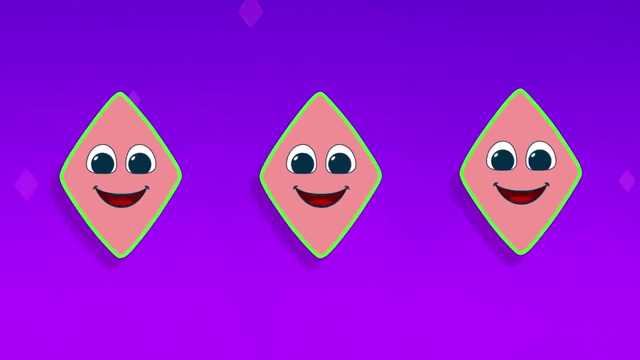 PEEKABOO, PEEKABOO, PEEKABOO. Yahoo FISH, FISH, ROMBUS, ROMBUS, ROMBUS, this is, is rhombus kite, kite, rhombus toy toy. rhombus diamond, diamond. rhombus rhombus, rhombus rhombus. 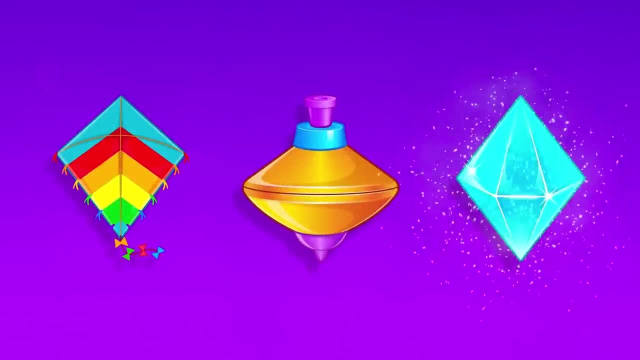 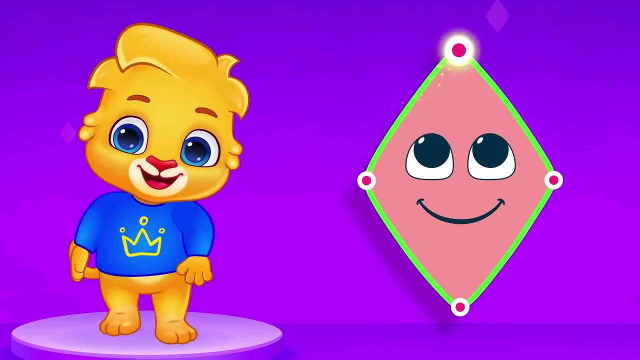 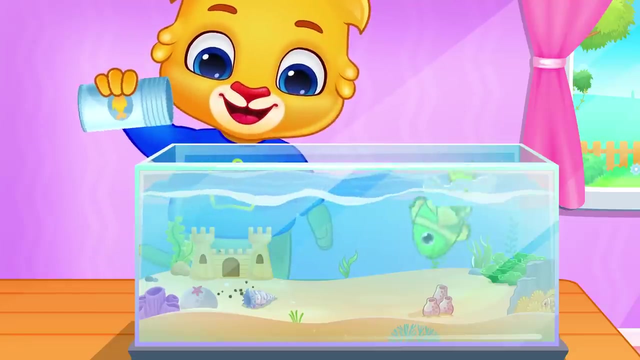 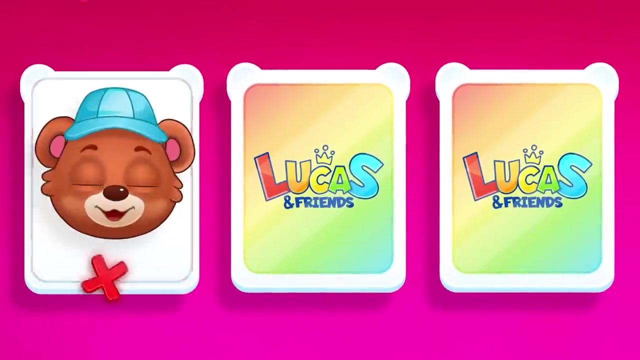 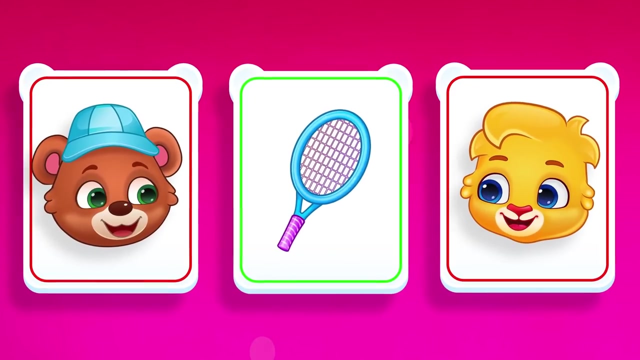 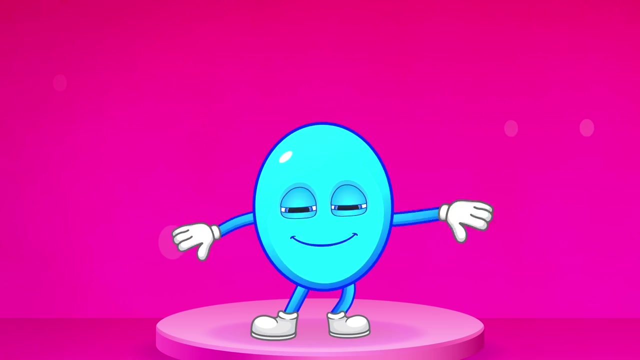 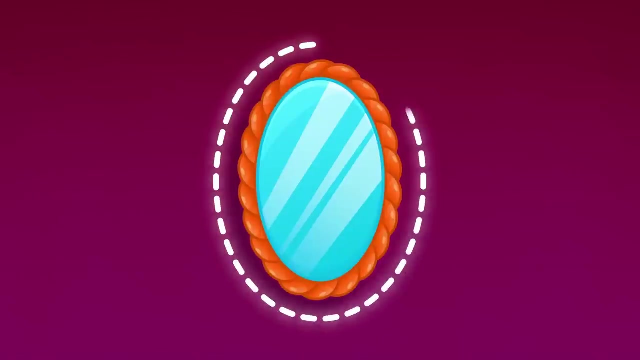 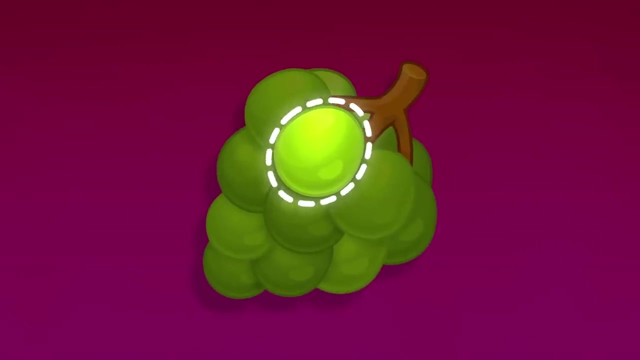 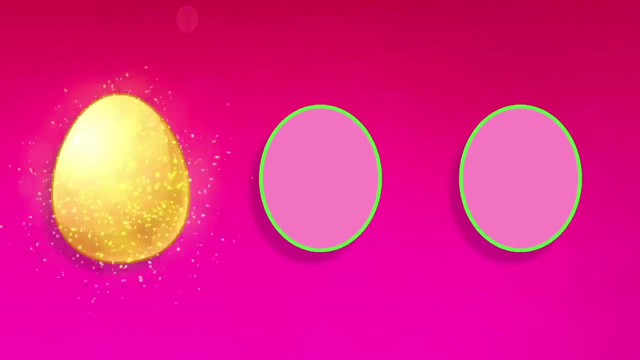 kite toy diamond rhombus, rhombus rhombus. this fish has a rhombus shape. lucas is feeding his pet fish racket, racket, oval, oval oval. this is oval egg egg oval mirror mirror oval grapes, grapes, oval oval, oval oval egg mirror grapes, oval. 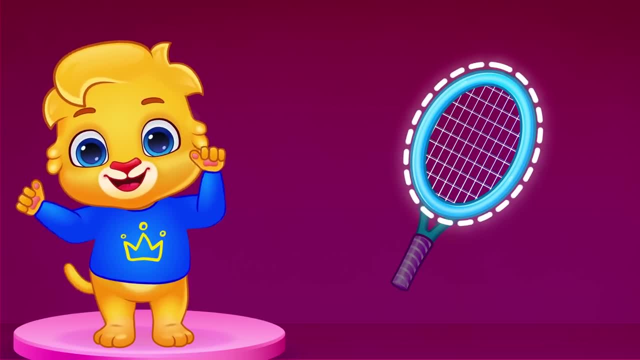 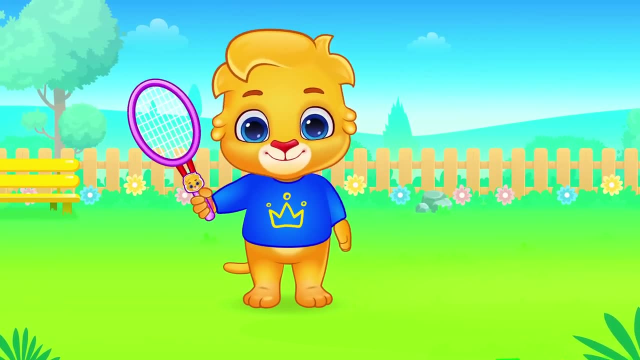 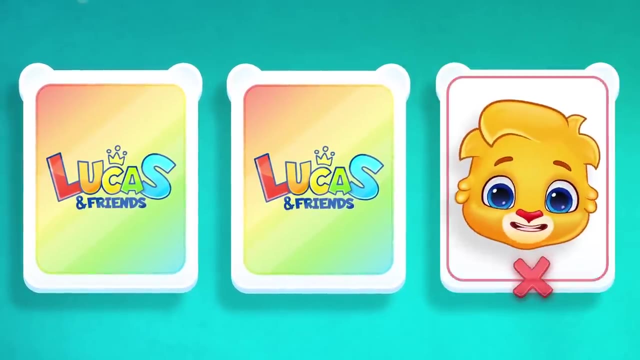 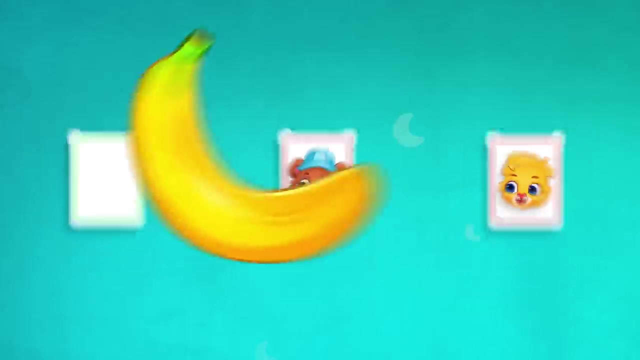 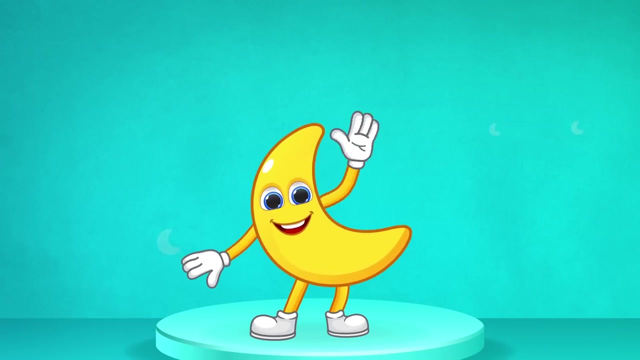 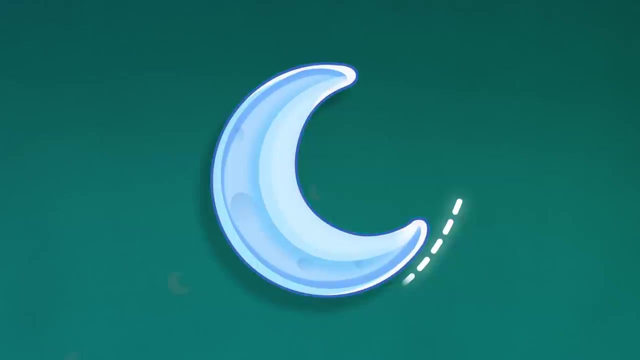 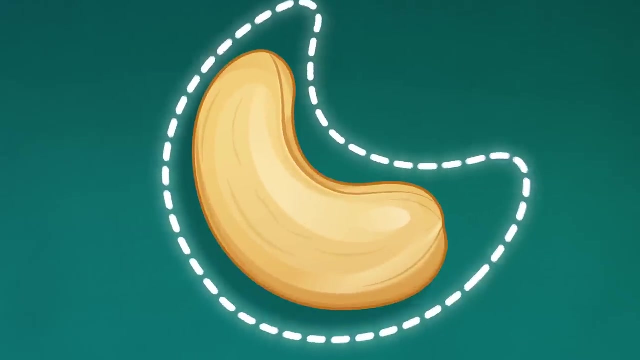 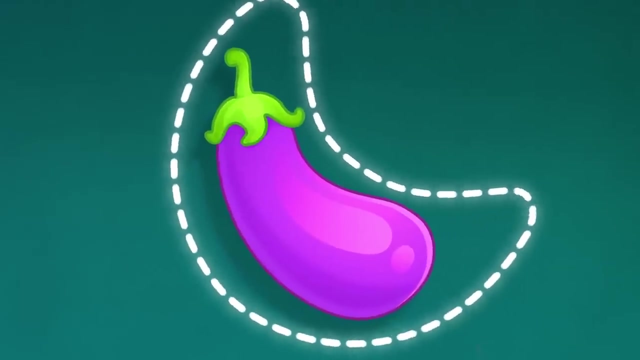 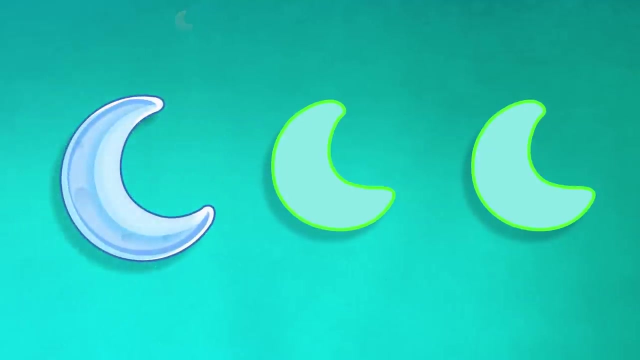 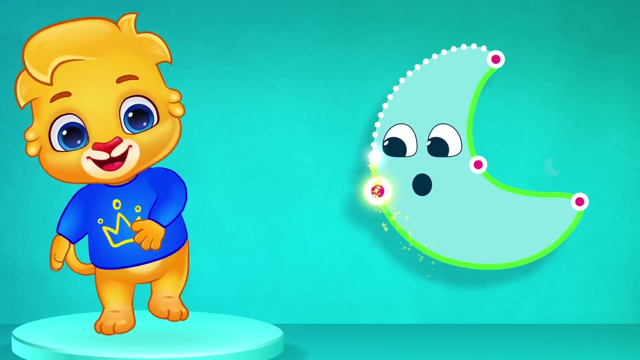 oval oval. the racket looks like an oval. lucas and his dad are playing with a racket. little, crescent moon crescent, cashew crescent. fringile- crescent, crescent, crescent. Boon- cashew, fringal crescent, crescent, crescent. 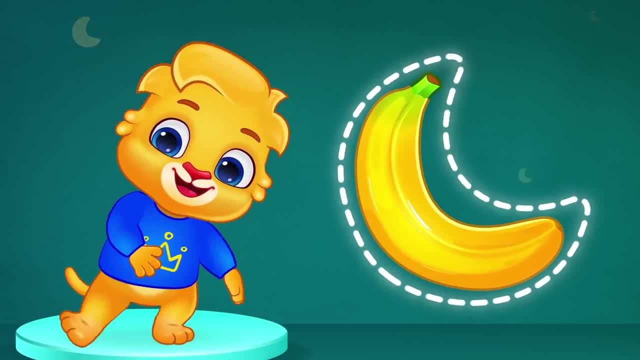 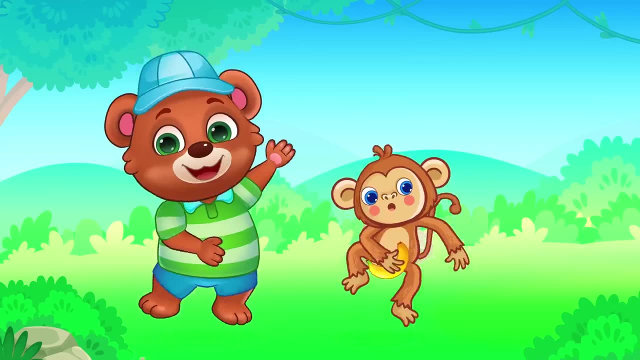 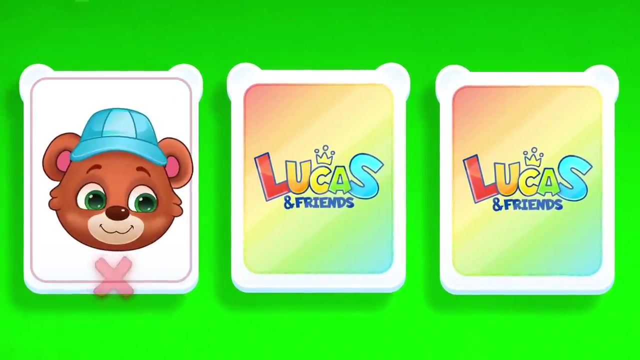 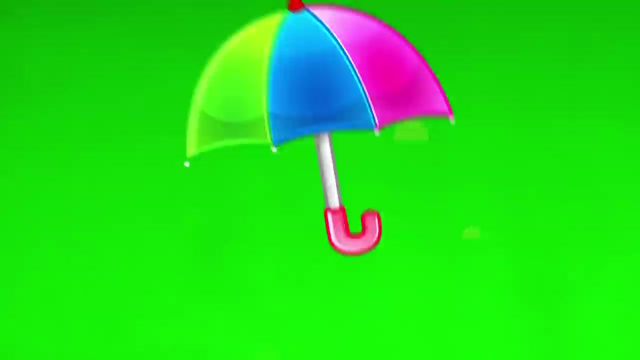 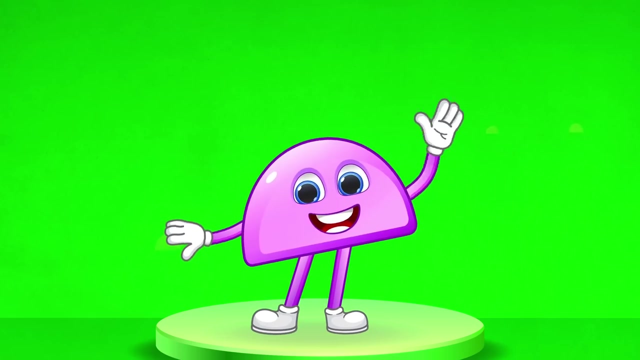 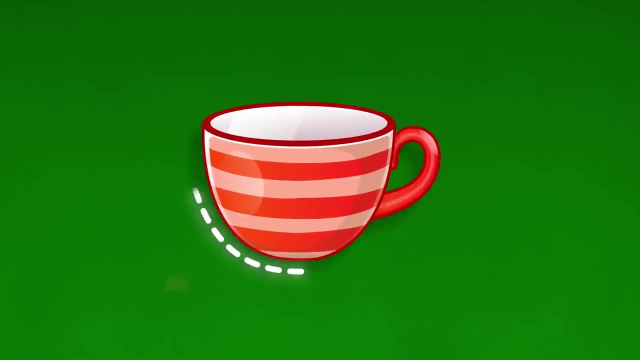 The shape of the banana is like a crescent. Brody gave a banana to the monkey. Umbrella, umbrella, semicircle, semicircle, semicircle. This is semicircle, Cup, cup, semicircle. 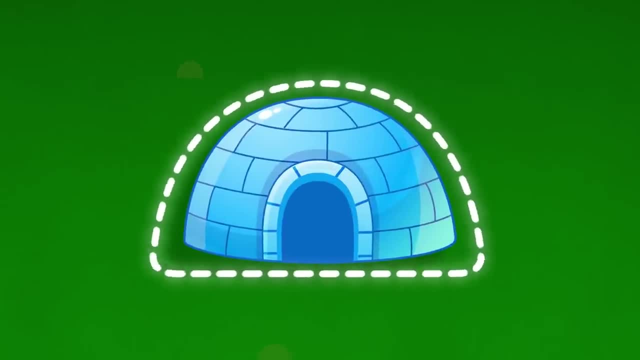 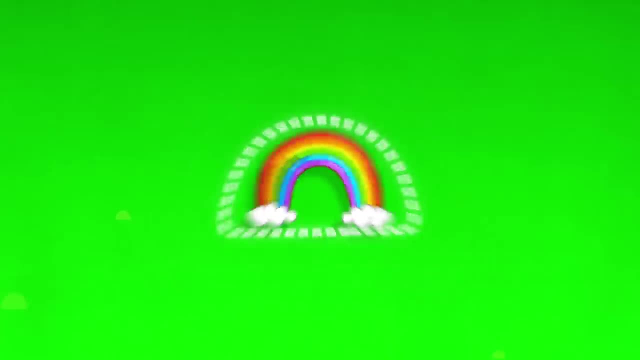 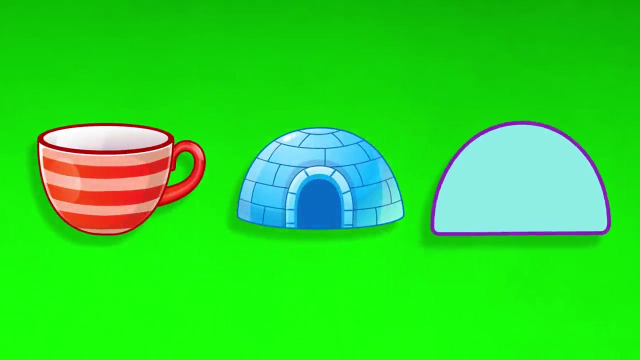 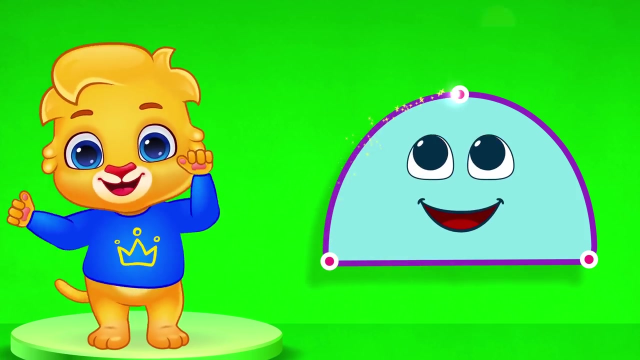 Igloo- igloo- semicircle, Rainbow. Rainbow rainbow- semicircle, semicircle, semicircle, semicircle. Cup igloo- rainbow- semicircle, semicircle, semicircle. 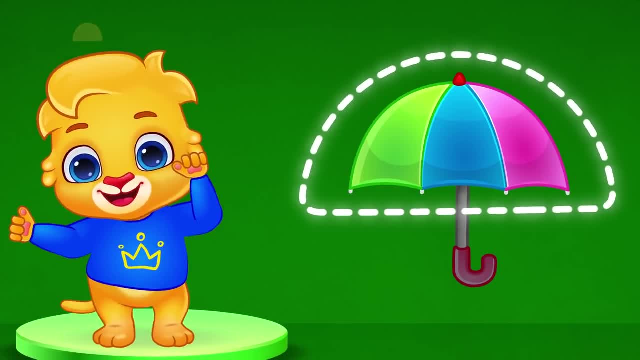 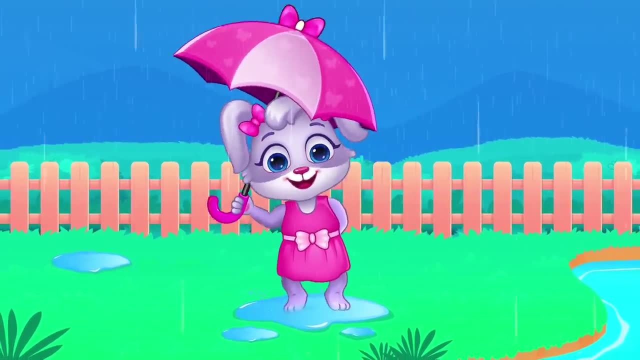 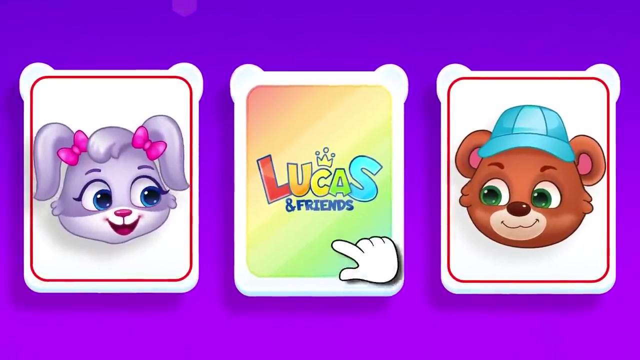 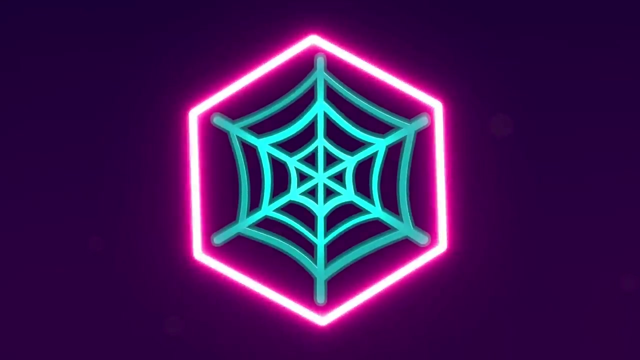 Umbrella looks like a semicircle. Ruby is dancing with an umbrella: Cup, igloo, rainbow, semicircle, semicircle, semicircle, semicircle, Web web, hexagon, hexagon, hexagon. 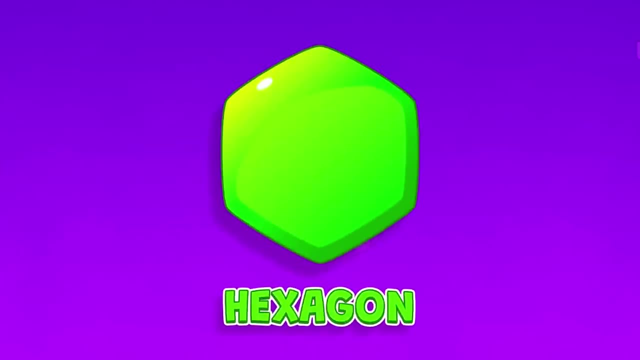 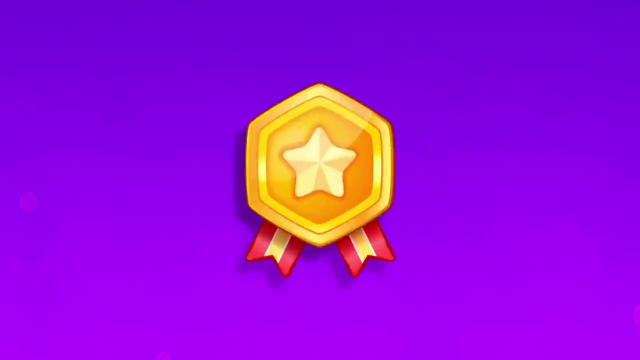 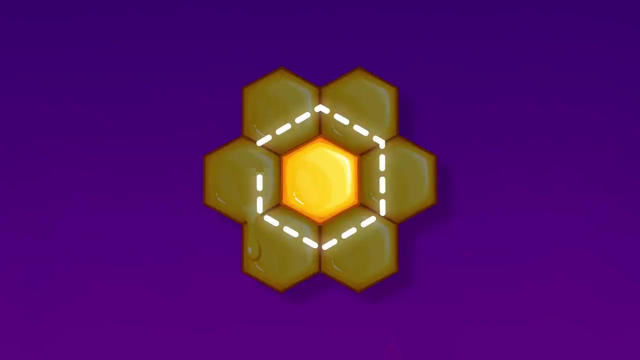 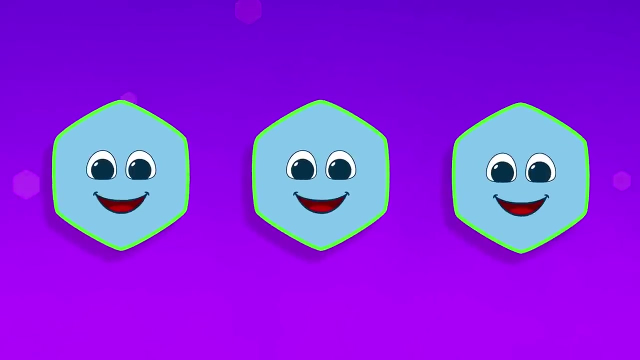 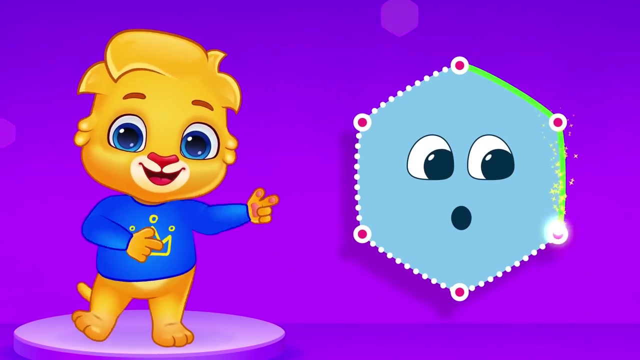 This is hexagon- Nut nut, hexagon- Metal metal. hexagon- Honeycomb- honeycomb- hexagon, hexagon, hexagon. hexagon- Nut metal- honeycomb- hexagon, hexagon, hexagon. 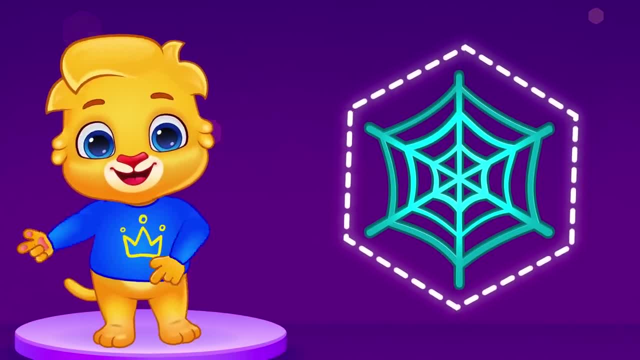 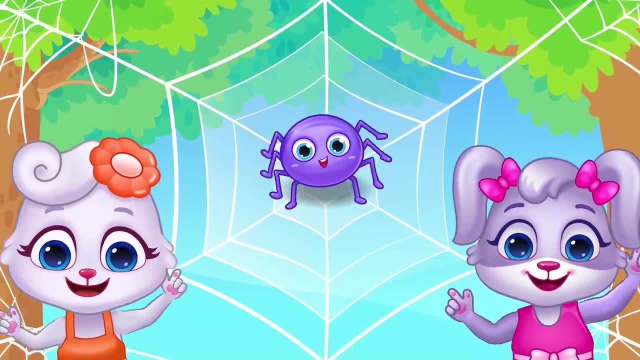 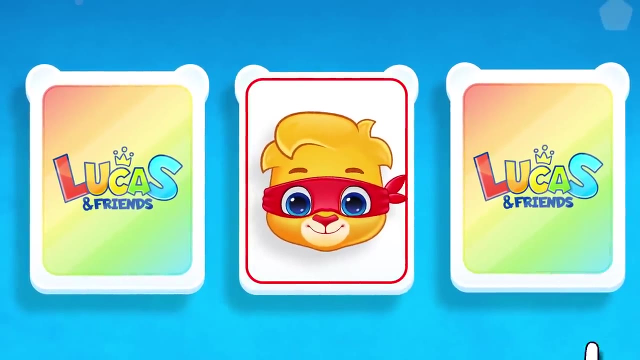 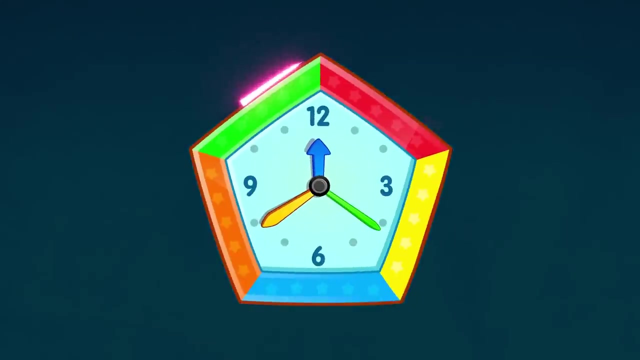 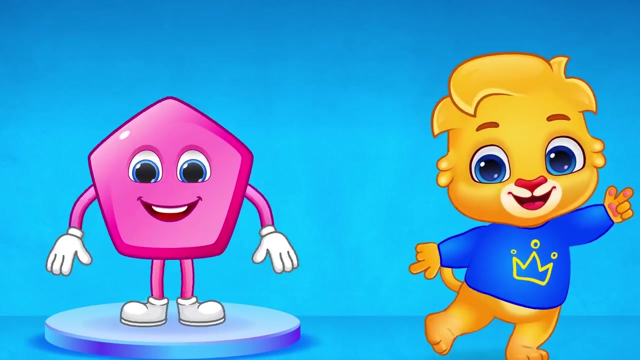 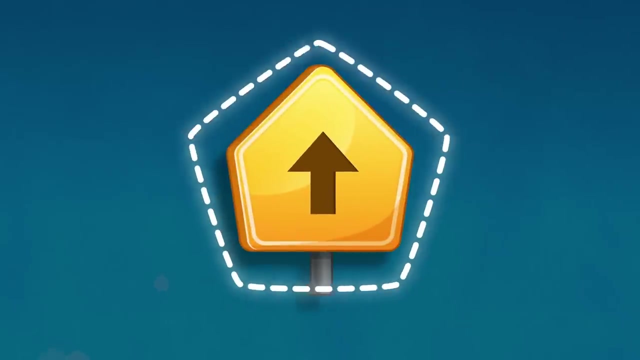 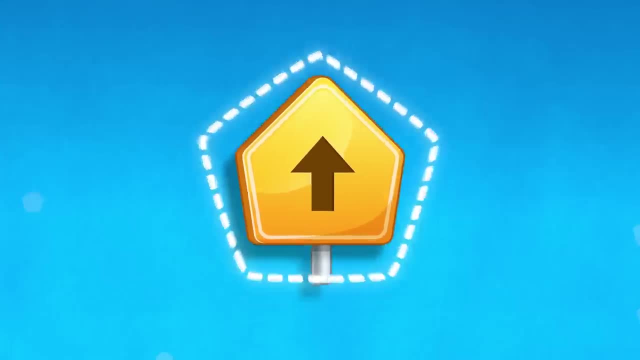 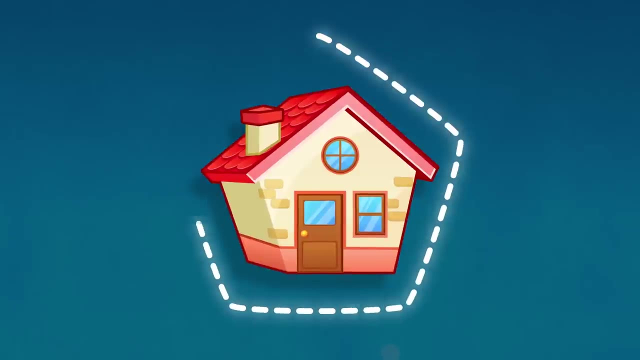 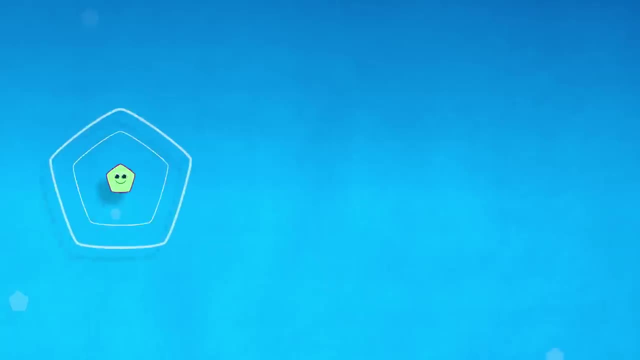 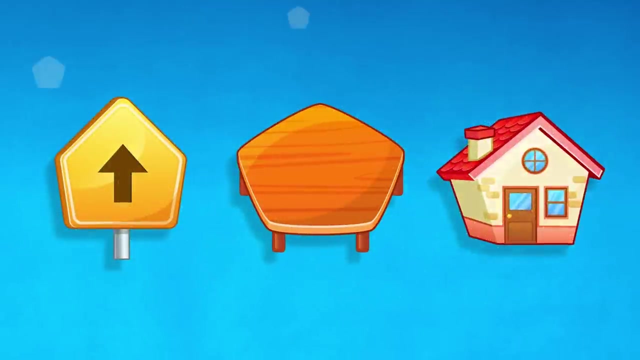 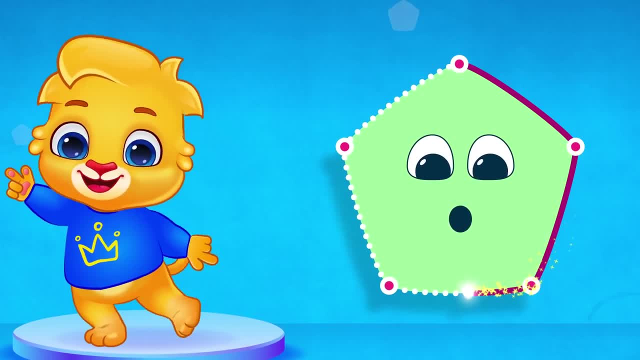 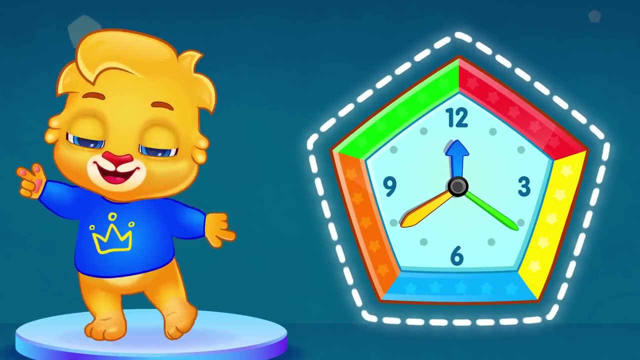 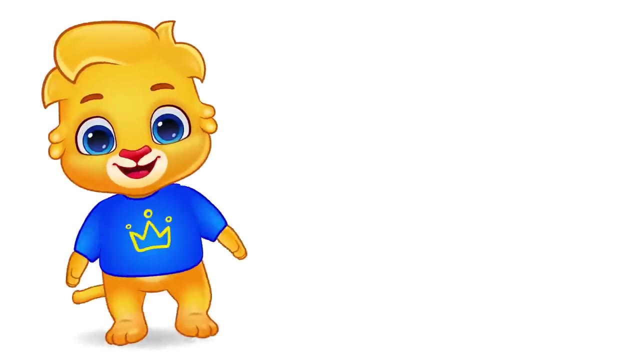 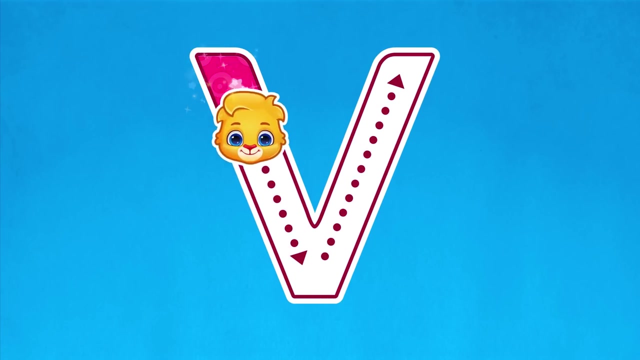 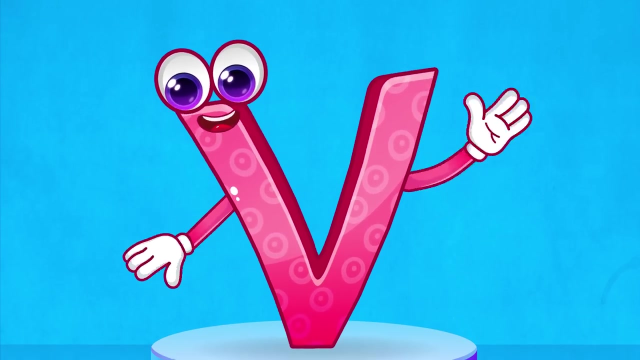 This is pentagon. This is pentagon. This is pentagon. Wow, Pentagon, Pentagon. The shape of this clock is like a pentagon. Lucas has a beautiful clock. V. This is V Hi. V is for VAN VASE. 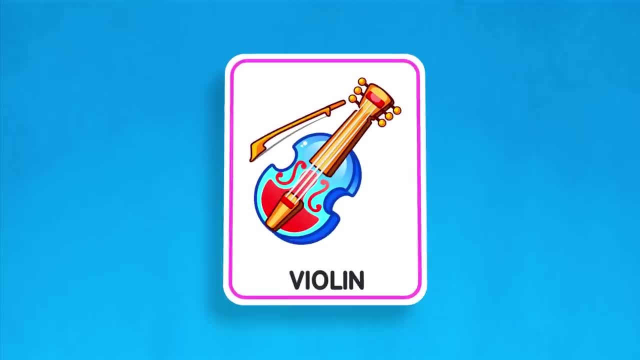 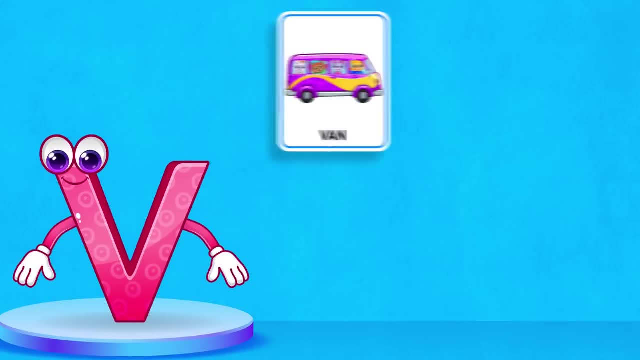 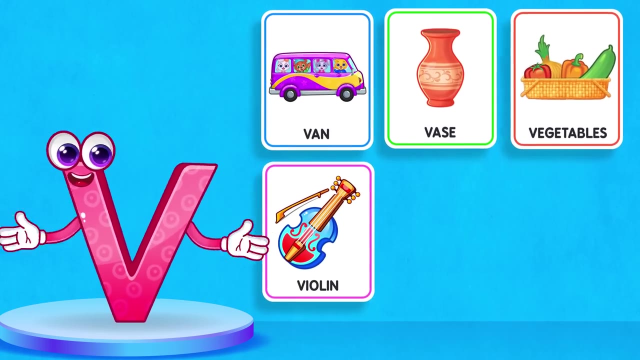 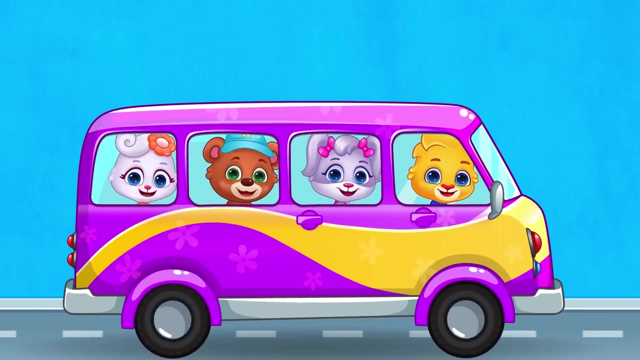 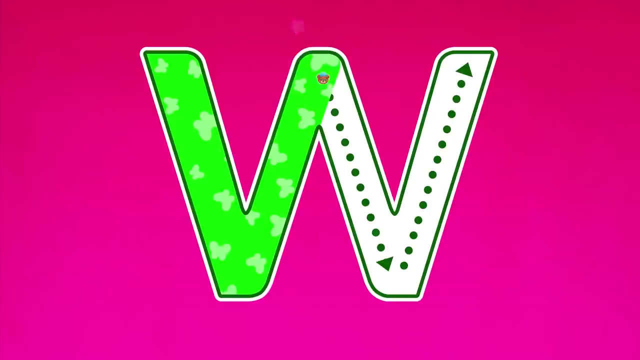 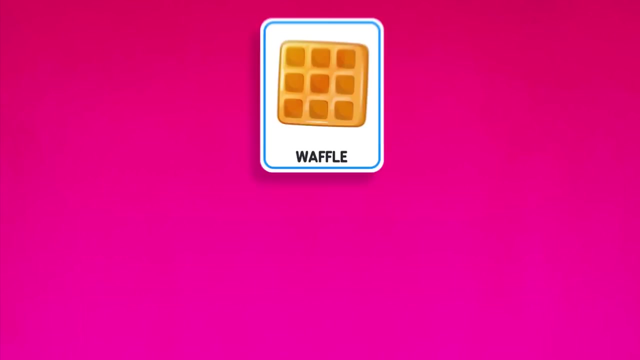 VEGETABLES VIOLIN VOLLEYBALL VULTURE. This is V, V is for VAN VASE. VEGETABLES VIOLIN VOLLEYBALL VULTURE. Hihi Kiki W, This is W, Hi W is for WAFFLE. 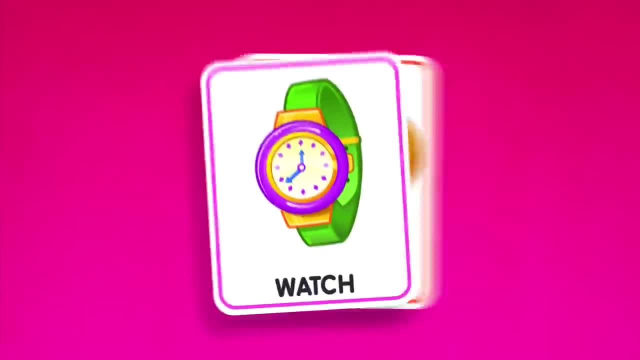 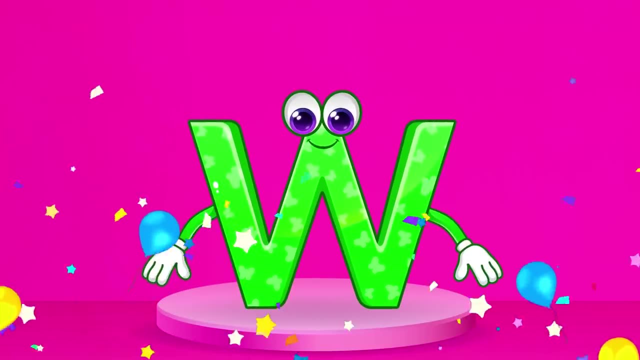 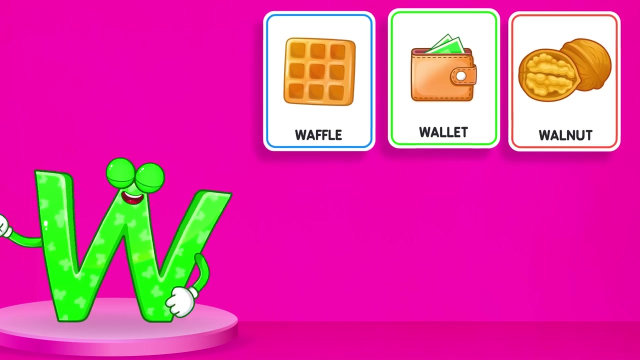 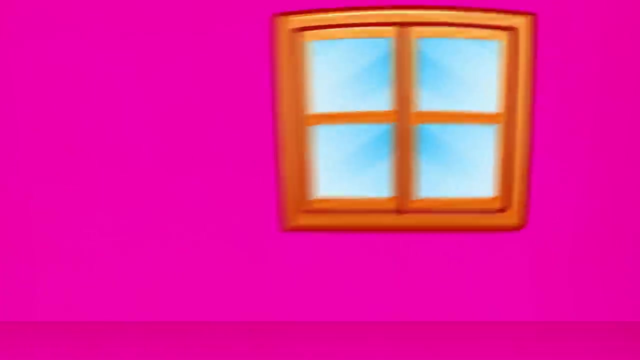 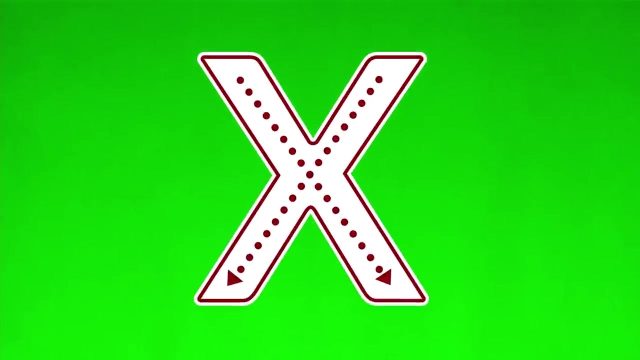 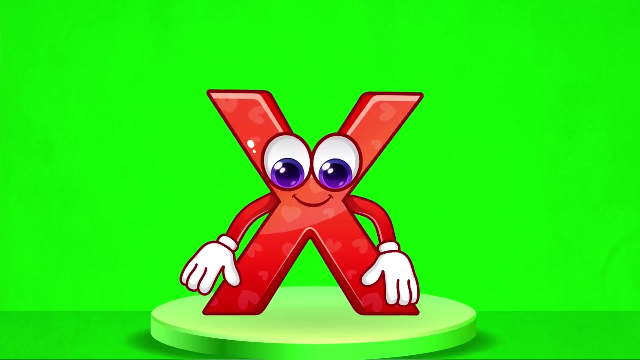 WALLET WALNUT, WATCH WELL WINDOW. This is W. W is for WAFFLE WALLET WALNUT, WATCH WELL WINDOW. Hi X, This is X. X is for CHRISTMAS TREE, X IS FOR CHRISTMAS TREE. X-Ray XYLOPHONE. 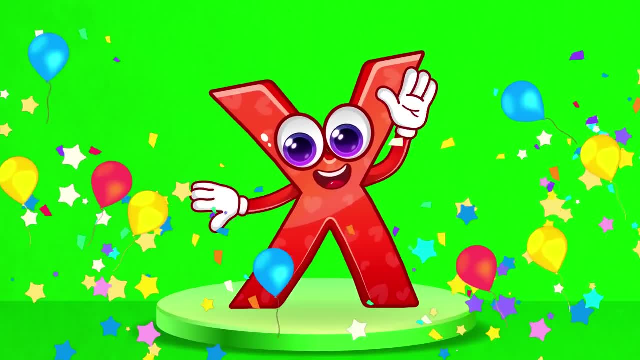 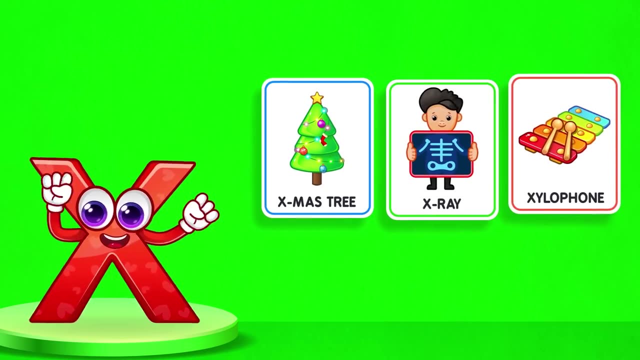 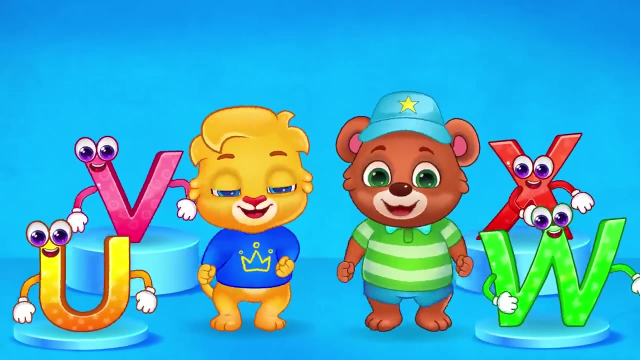 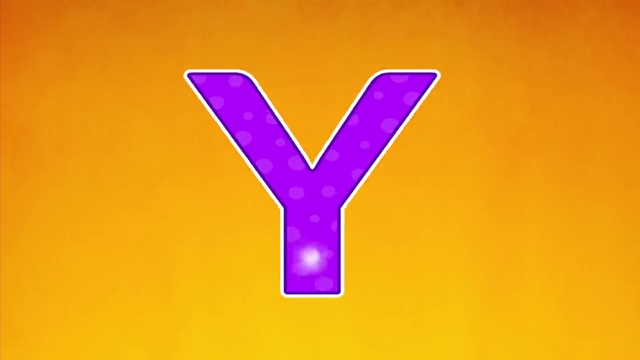 X-Ray XYLOPHONE. This is X, X, X is for CHRISTMAS TREE- X-Ray, X-Ray, XYLOPHONE. X-ray XYLOPHONE, XYLOPHONE Y, XYLA, XYLA, XYLA, XYLA, XYLA, This is Y.